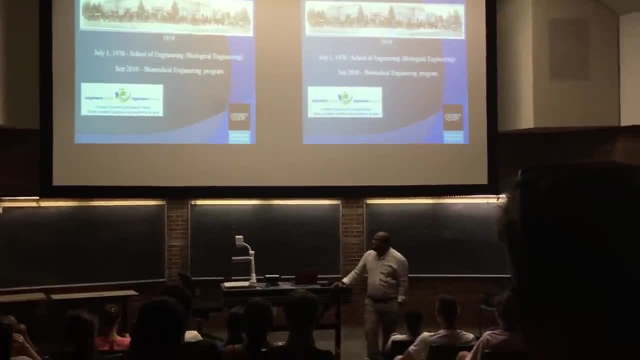 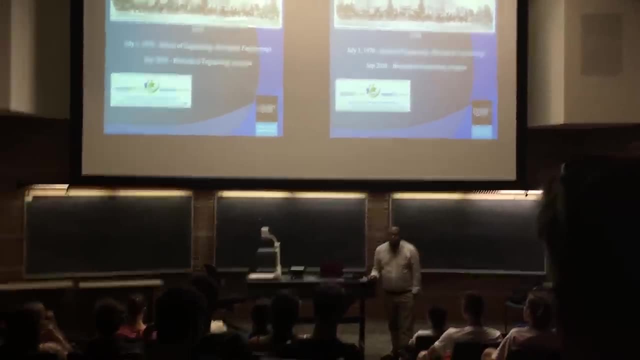 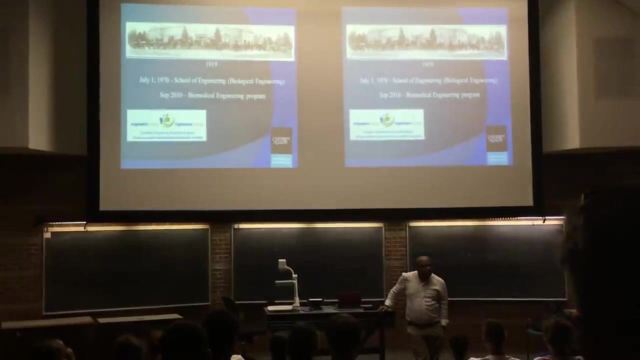 It became Biological Engineering Department in 1980.. In 1970, July 1st, Canada Day- we became the School of Engineering. The Biomedical Engineering program is relatively a new program, which was introduced in the year 2010,- about six years ago as of today. 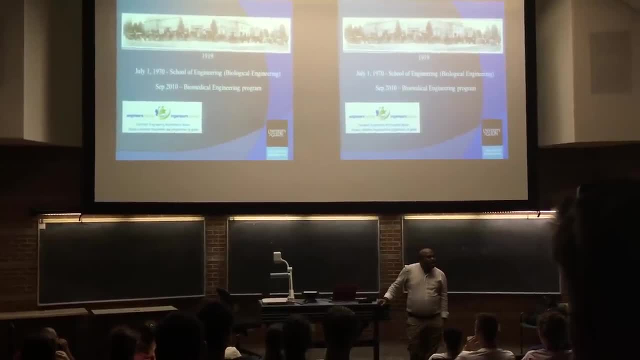 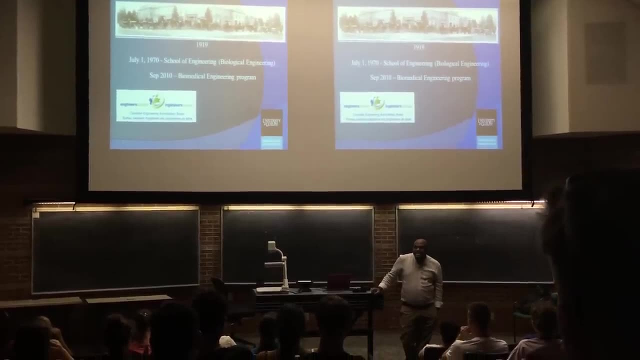 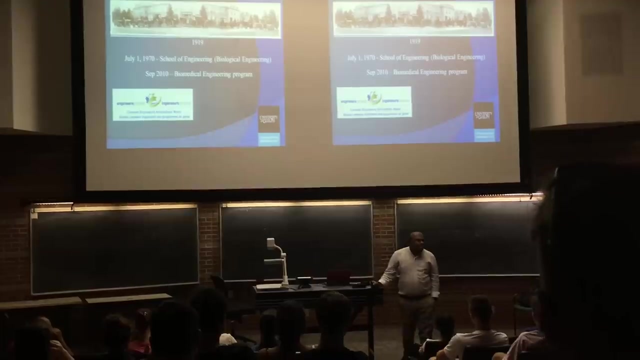 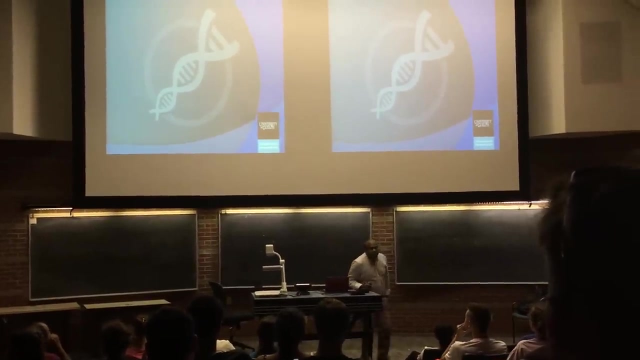 It is a well-recognized and accredited program, which means that we have gone through all the stringent regulations and the CEA- the Canadian Engineering Education Board- accreditation requirements in terms of meeting the standards and the policies. So, as you can see here, that's the logo of the Biological Engineering program. It is DNA, double helical DNA. 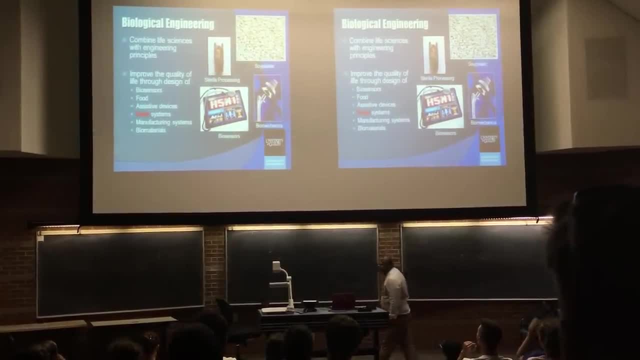 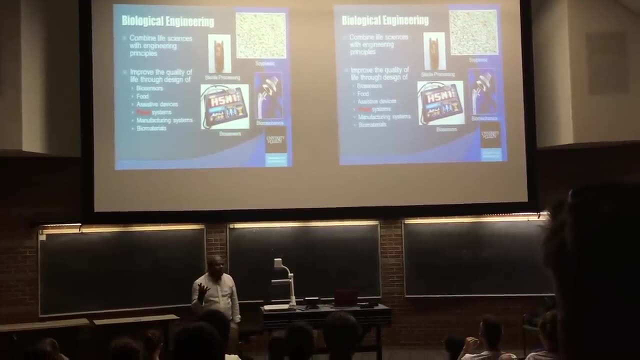 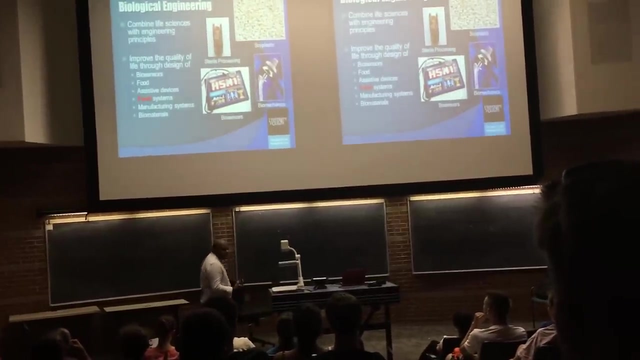 So what exactly is Biological Engineering? program means? If you look at the various universities within the country of Canada, there are only four universities, just four universities, that offer this specific program, Biological Engineering. They are unique. So what does the word bio mean? 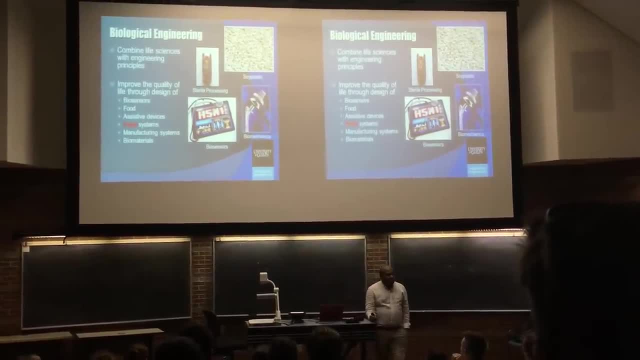 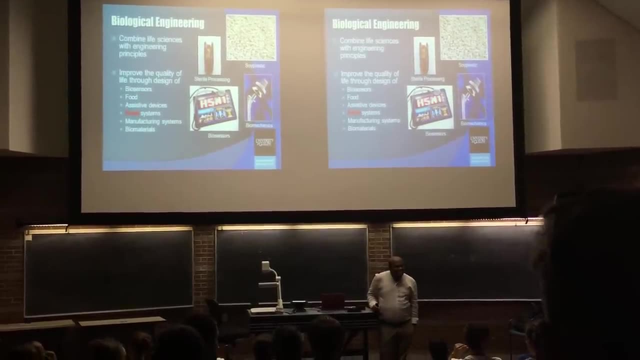 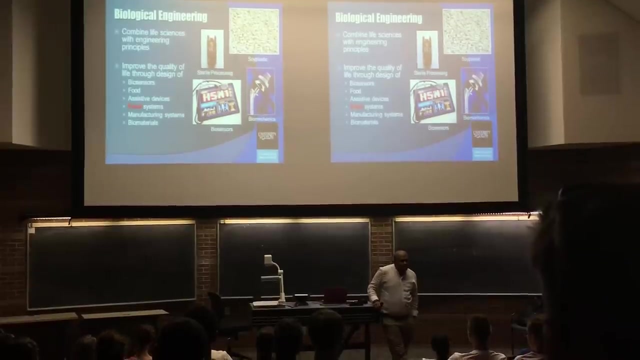 Bio. What exactly does the word bio mean? Yes, Biology, Biology. okay, Bio means life, Life, yes, exactly. So the word bio means life. When you utter the word bio here in Guelph, in the southwest Ontario, 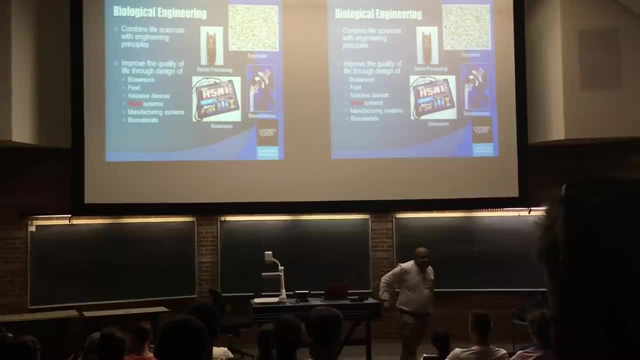 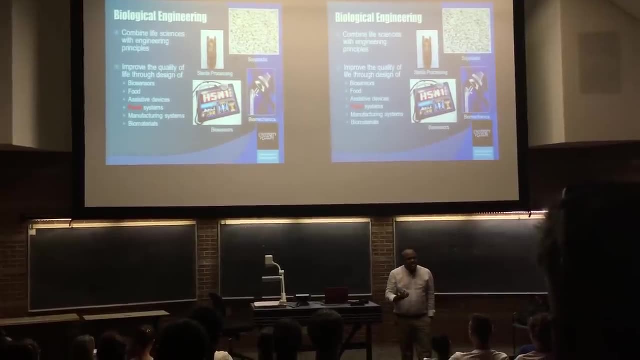 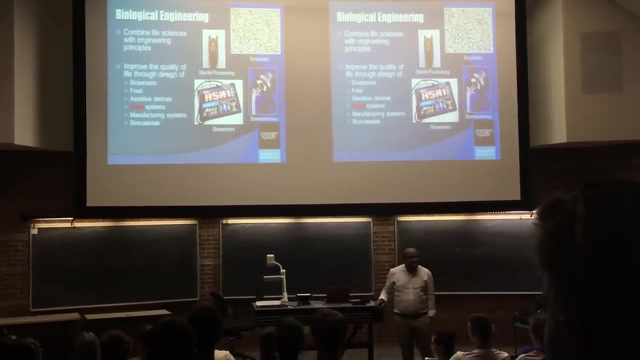 in the province of Ontario in Canada. it resonates not only within Canada but across the whole globe Because there's a trust here- mainly considering the Agricultural College, Veterinary College and also the College of Biological Sciences- the ability to provide realistic solutions for all life forms. 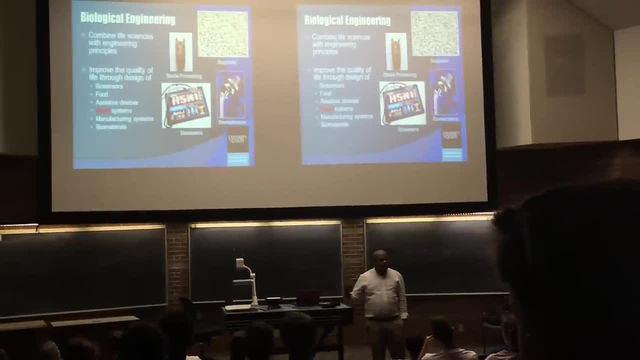 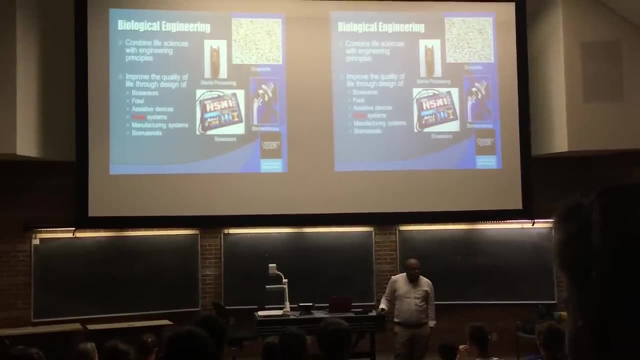 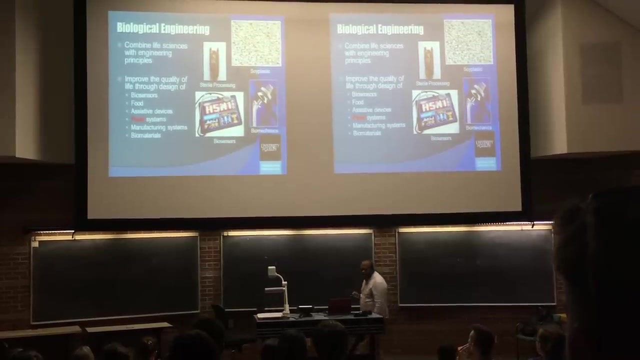 like human, animal, plant food, irrespective of the type of life forms. the ability to deploy design-based solutions using different engineering approaches is unique, So the word resonates. So in the Biological Engineering program we combine life sciences with engineering principles. 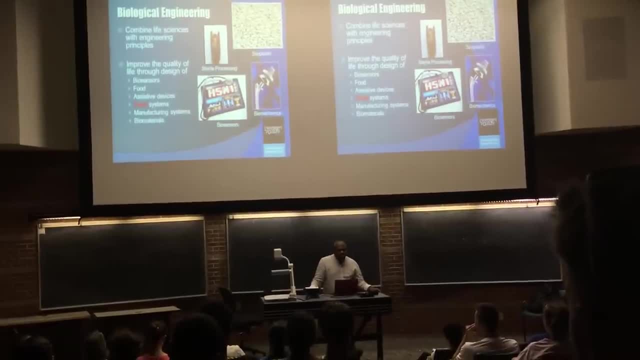 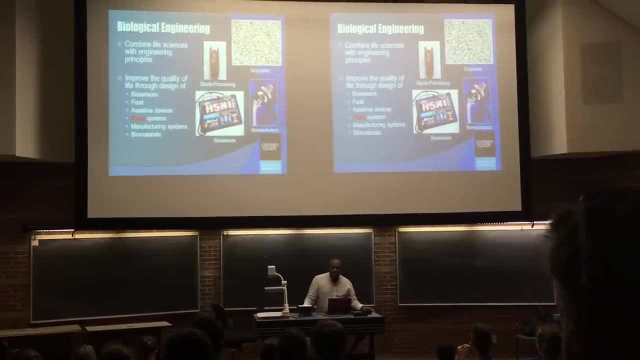 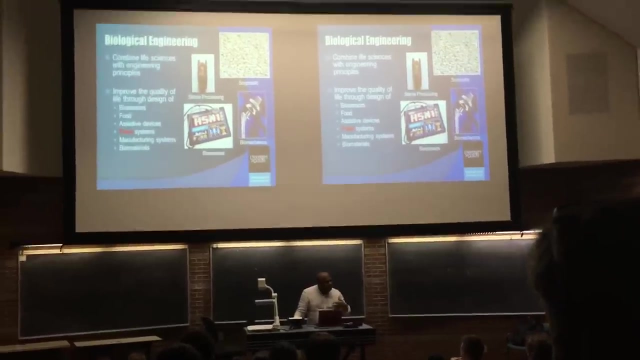 So just a flavor of the Biological Engineering program is the biosensors. We talk about and study about different concepts regarding food, food engineering, food processing, food safety, how to manufacture food. Once you manufacture food, how we can go about extending the shelf life of the food. 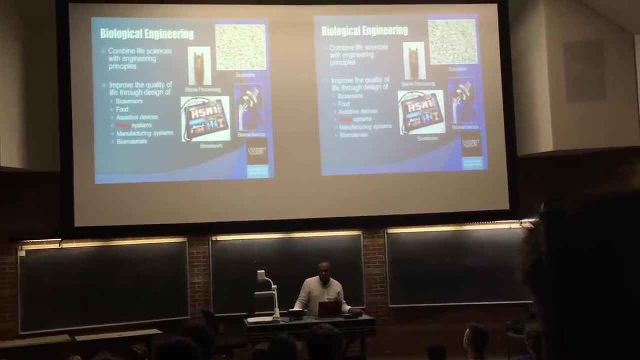 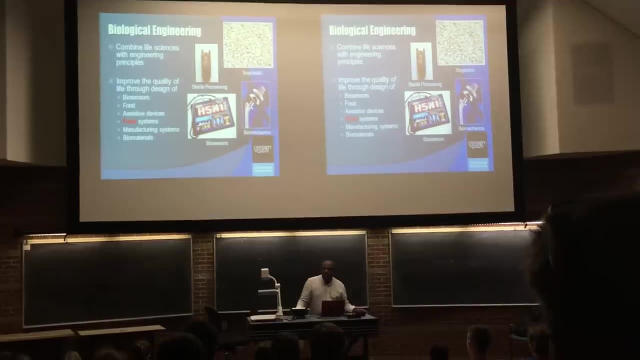 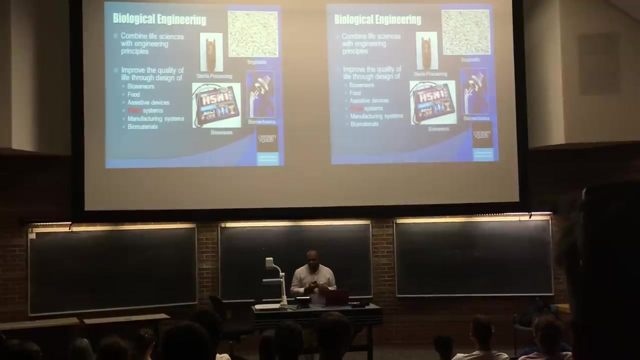 what are the different practices we could deploy in manufacturing the food in terms of bringing down the cost, in terms of meeting the sustainability requirements and the energy-related associated costs? Assistive devices, such as prosthetic devices, orthopedic screws in a human body. 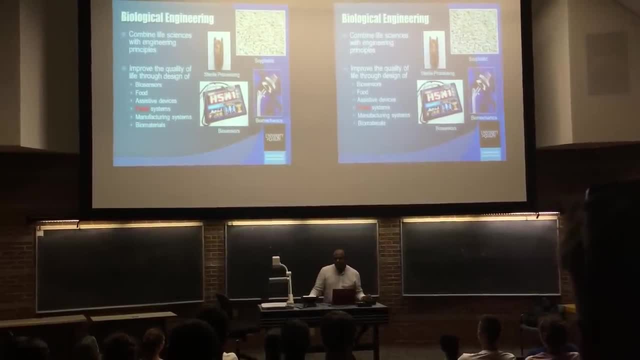 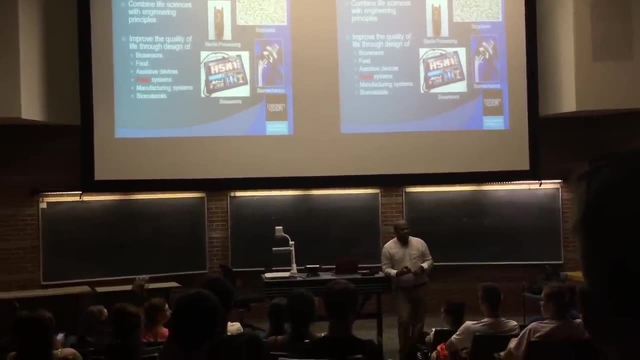 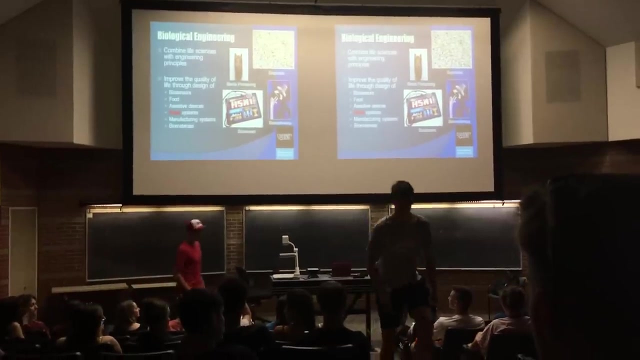 food systems, manufacturing systems and biomaterials. So how many of you here are in Biological Engineering program registered and enrolled? Good, And how many of you are in Biomedical Engineering program? That's quite a chunk, Good, good. 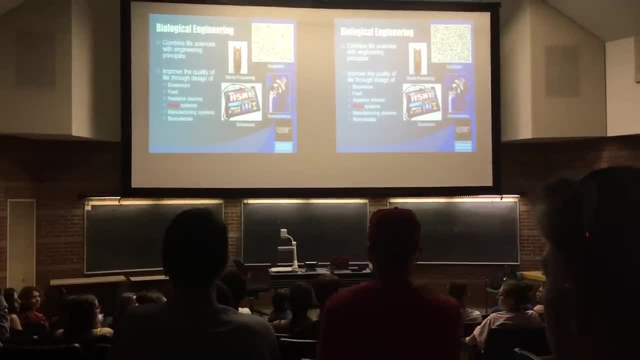 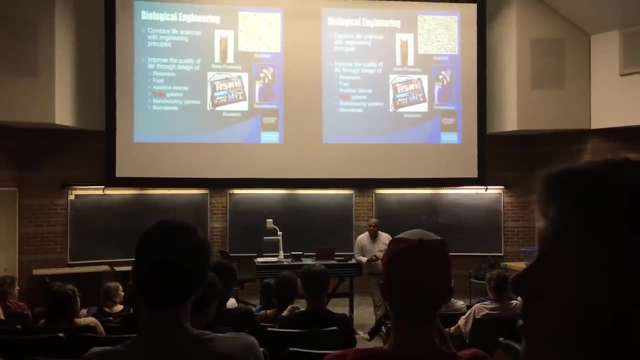 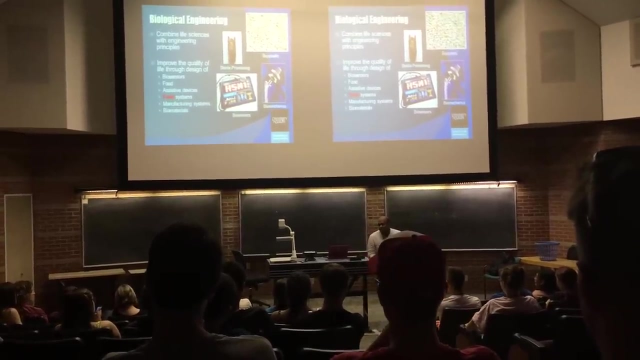 Undeclared. How many of you are undeclared? Two, three. So my goal at the end of today's presentation to convince you to take and enroll into Biological Engineering program, if not at least Biomedical Engineering program. So please consider, by the end of the day, to make up your mind in terms of enrolling. 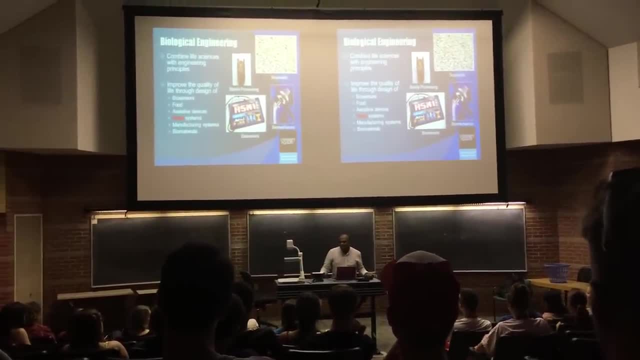 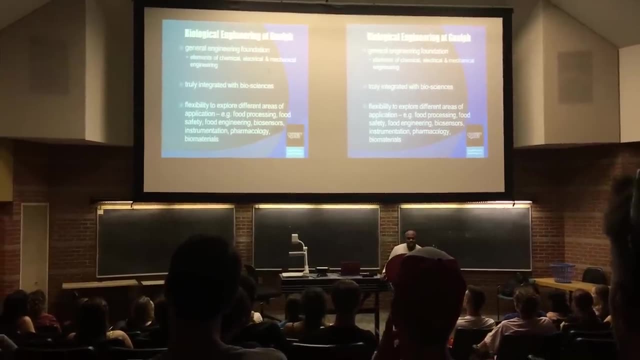 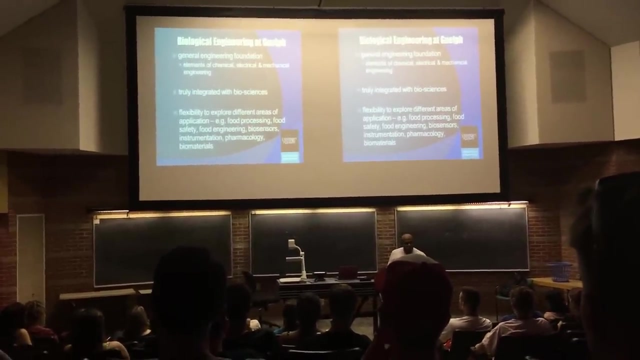 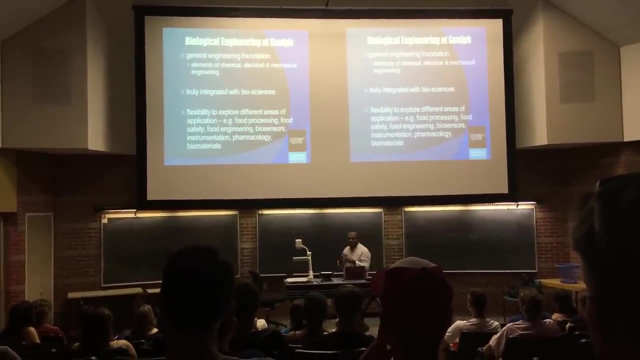 what you want to exactly do for the next four and a half to five years. So, as I said, there are four Biological Engineering programs across Canada. The uniqueness, the specialty of the University of Guelph is design. So design is a gem in the throne of the University of Guelph's engineering school. 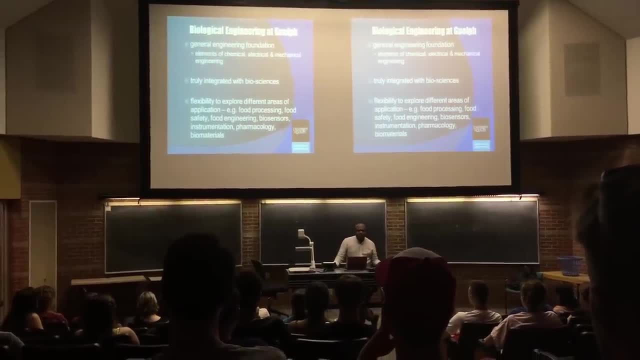 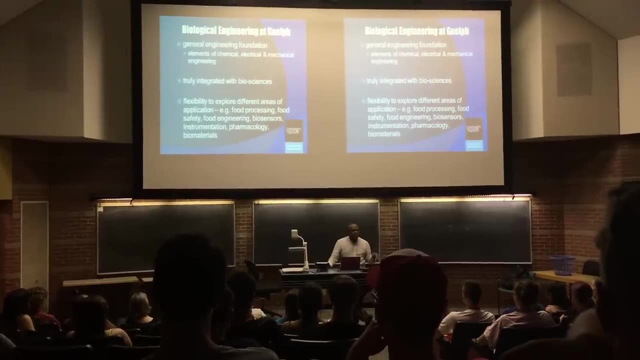 So we use design principles at different levels right from the year. one design, one design, two, 2100, 3100, 4100, which is what's in the next? In addition to that, there are a variety of programs. 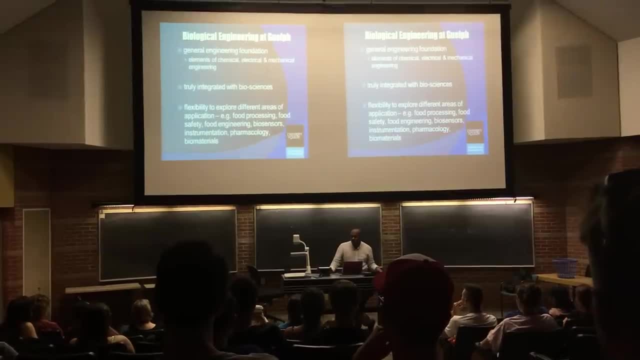 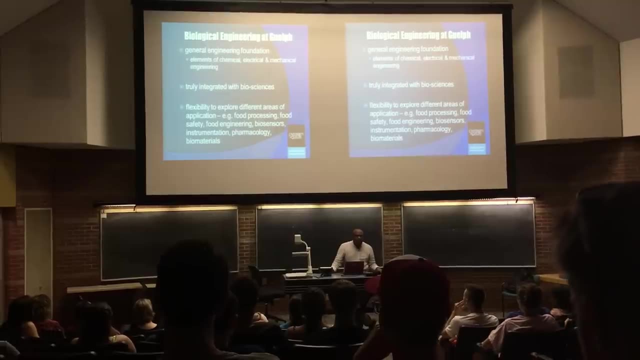 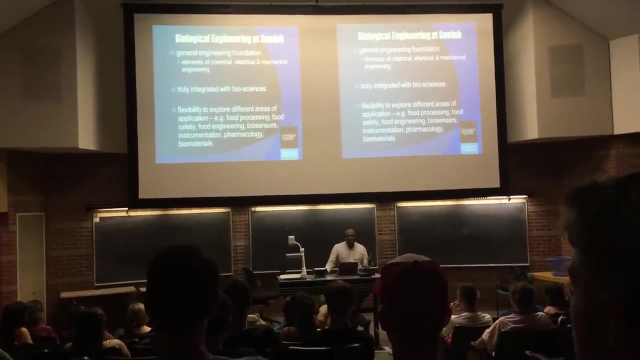 There are a variety of courses, irrespective of the streams you are going to enroll in, For example, a Bioprocess Engineering or Instrumentation Design or a Biomechanical Design. So there are specific design-oriented courses in terms of the streams you are going to take. 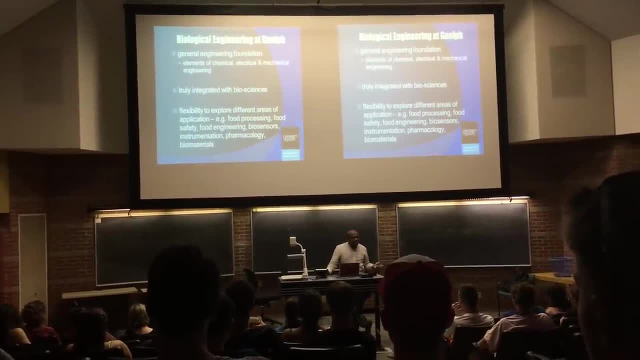 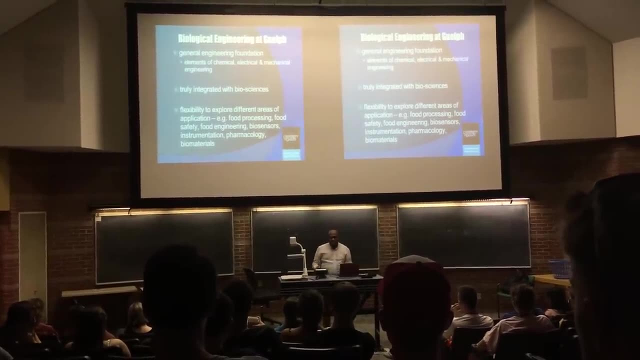 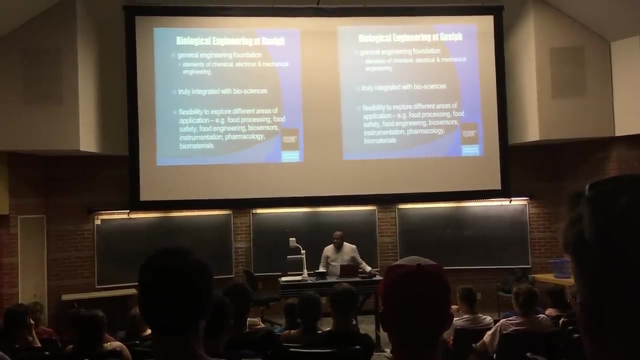 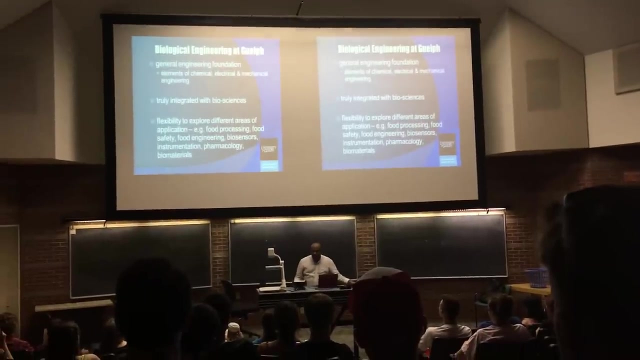 So the flavor is associated in strengthening and bringing down the unique aspects in terms of technical skills and technical knowledge, in building up the core towards the design-oriented nature. So the Biological Engineering program is truly integrated with biosciences. In the past two years we will be talking about the basic engineering concepts through various courses. 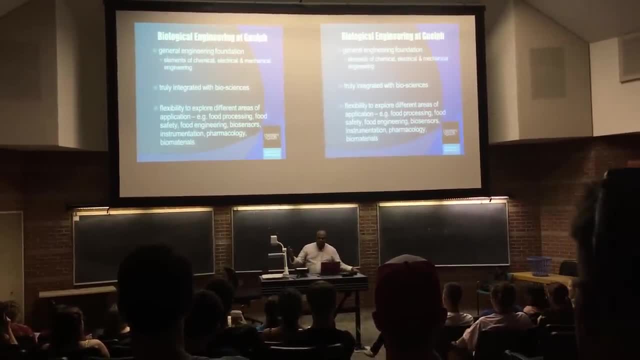 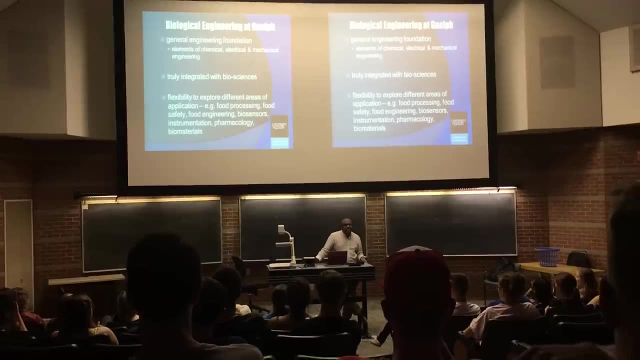 And in the upper years, third year, fourth year and probably if you are in the fifth year. you don't have a fifth-year level course, But if you are in the co-op program, you will learn more hands-on approaches in terms of solving reality. 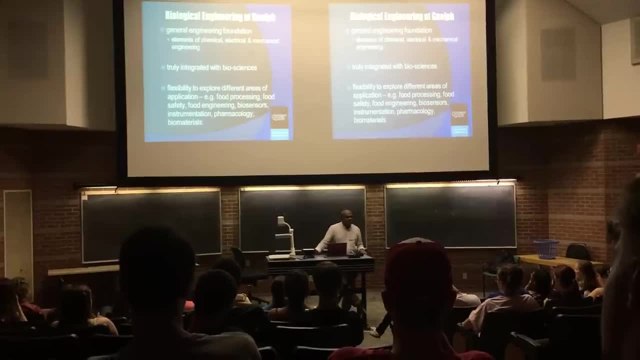 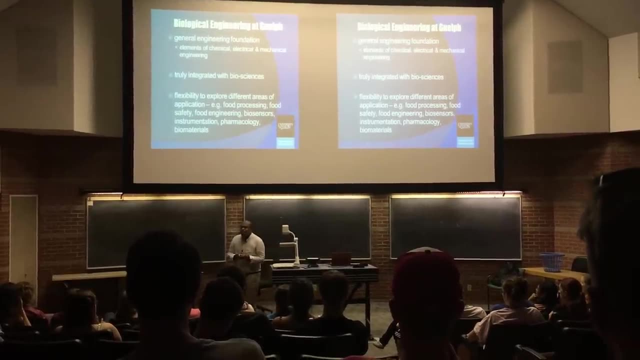 You will be able to solve realistic problems using the basic concepts you have learned in the year one and year two. So there is the flexibility. So when we look at the alumni from the Biological Engineering program, it's 1970, today is 2016.. 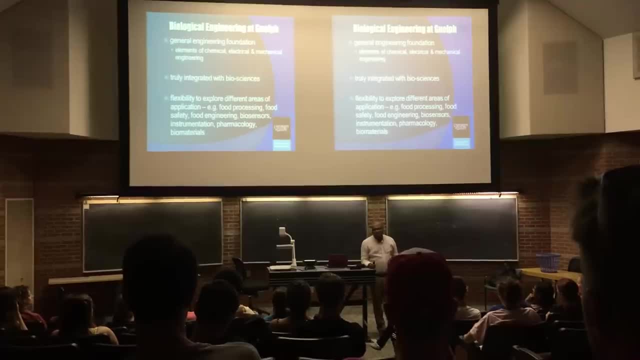 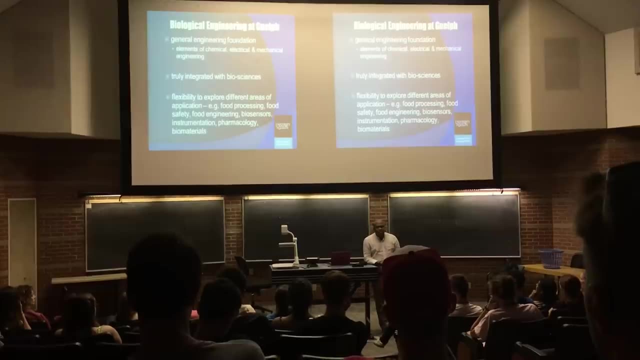 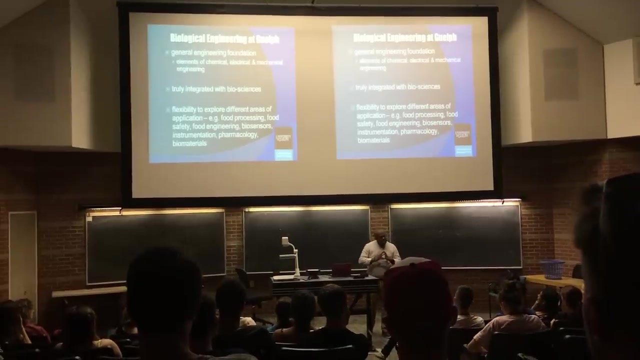 So almost three and a half decades. Our alumni are well-placed and employed at different levels: Vice President in GE to Canadian Food Inspection Agency, to different levels of private government and other sectors. So because of the unique nature they feel, more often they make a statement. 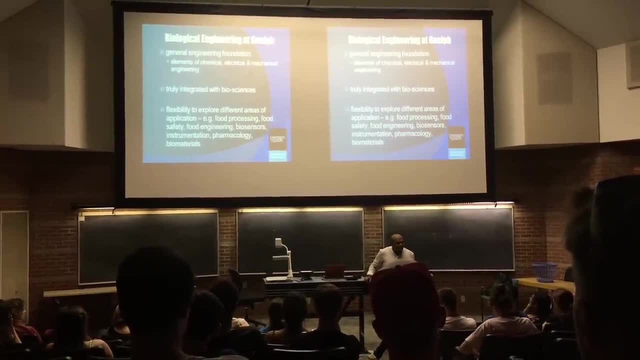 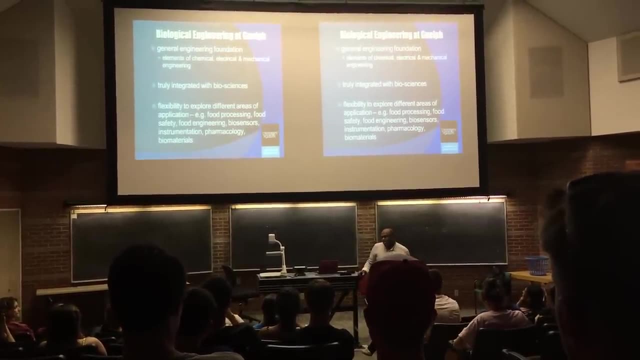 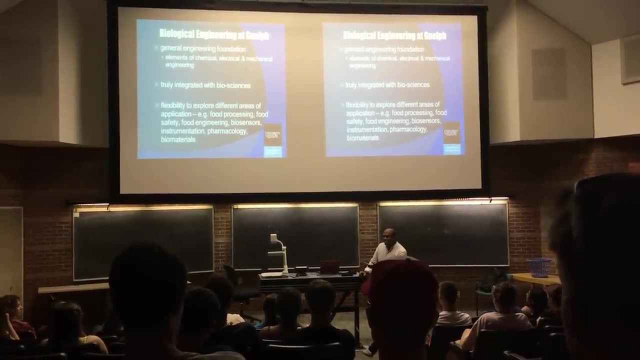 that they feel like a king of all trades or a queen of all trades. So if there is a problem in real life, if they are working as a biological engineer in an industry, when they have to have a conversation with a civil engineer or mechanical engineer or electrical engineer, 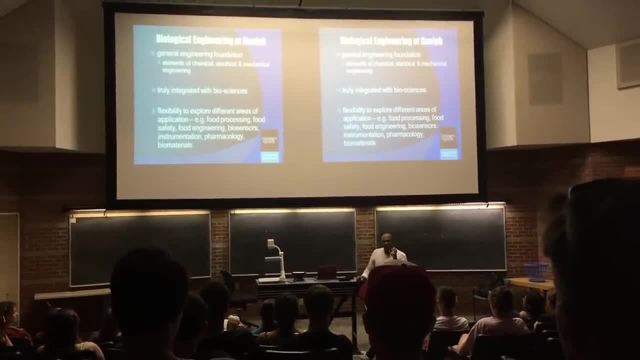 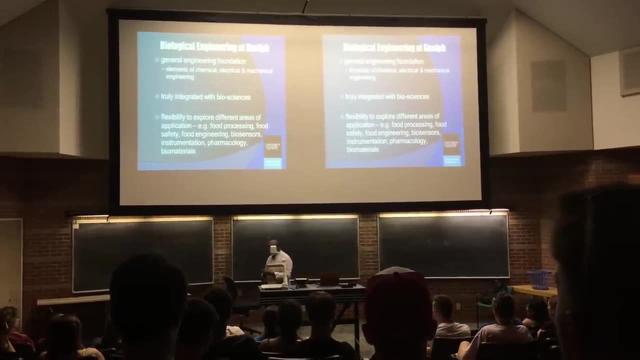 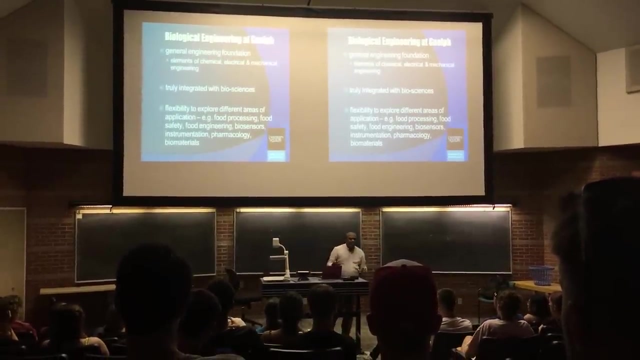 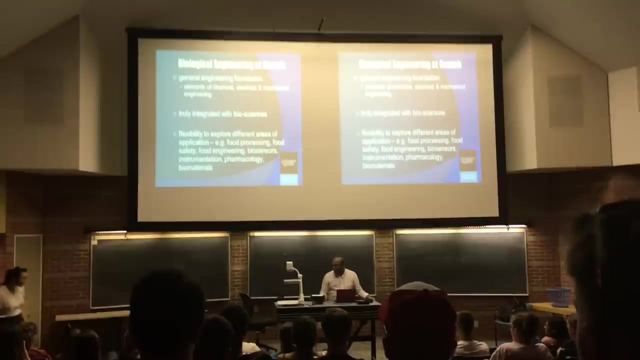 because specific elements of each and every of these different expertise is built into biological engineering programs. So they have a better appreciation of the type of understanding in terms of how to solve problems using a variety of engineering solutions and approaches. So the flexibility to explore different areas of application. 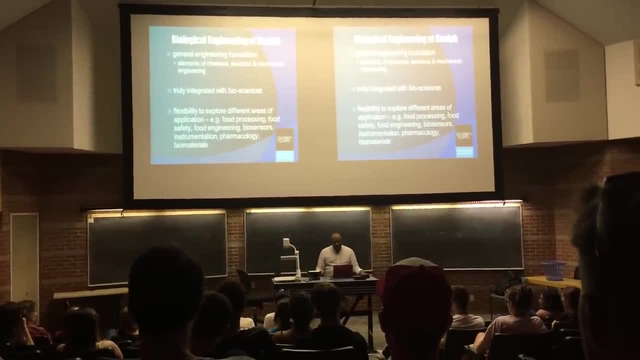 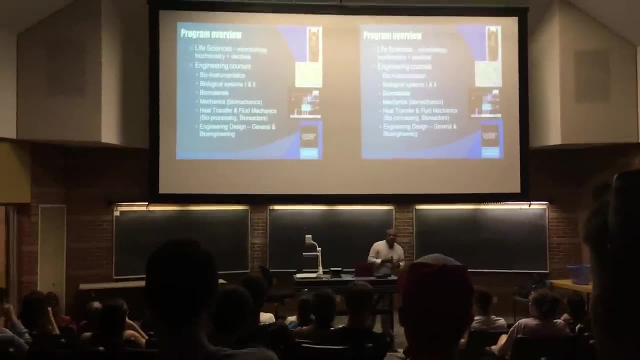 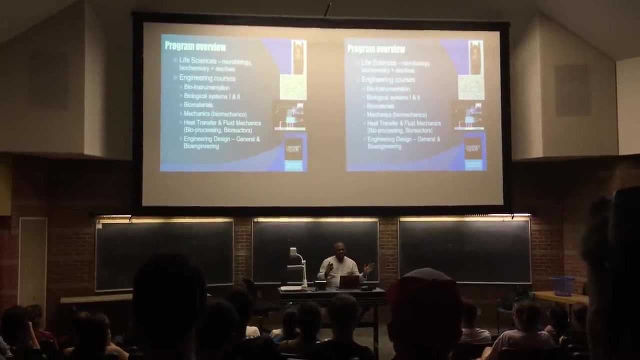 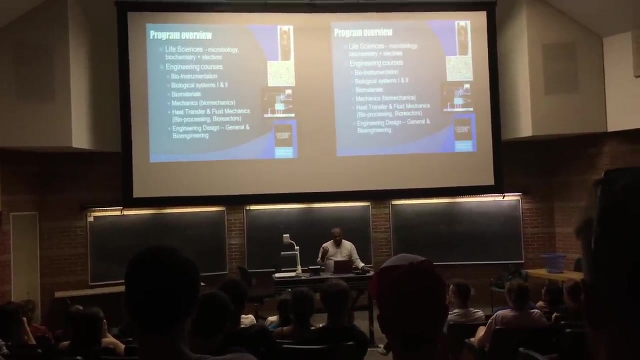 food processing, food safety, food engineering, instrumentation, pharmacology and biomaterials. A very brief overview of the program in terms of the biological engineering. What differentiates between biological versus biomedical? The majority of emphasis of biological engineering is on biochemistry and microbiology. 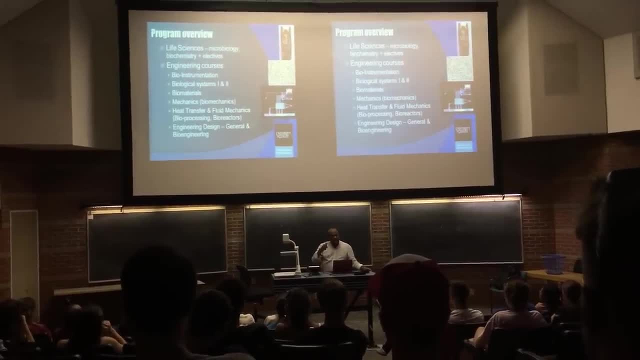 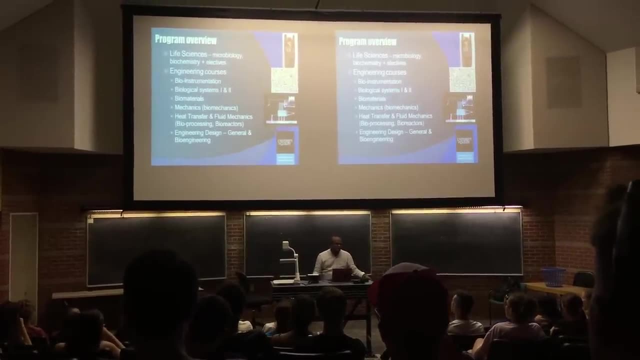 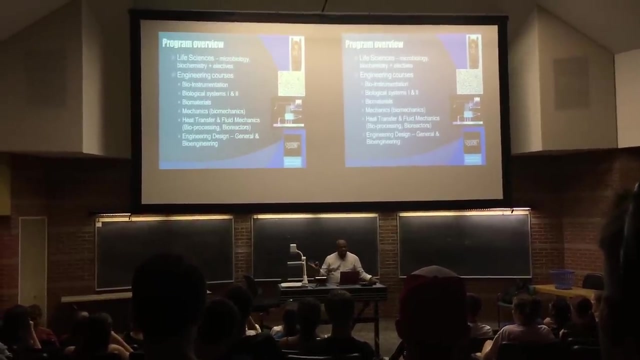 and there are some specific electives associated to it in the first and second year, But as you build on, you have the option to choose a specific stream in terms of food engineering or in terms of biomechanical or bioinstrumentation related focus in developing your skill sets. 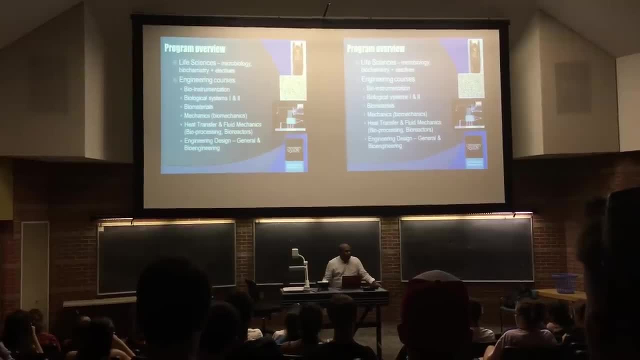 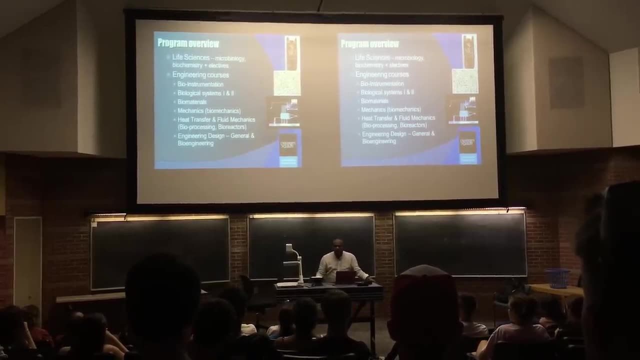 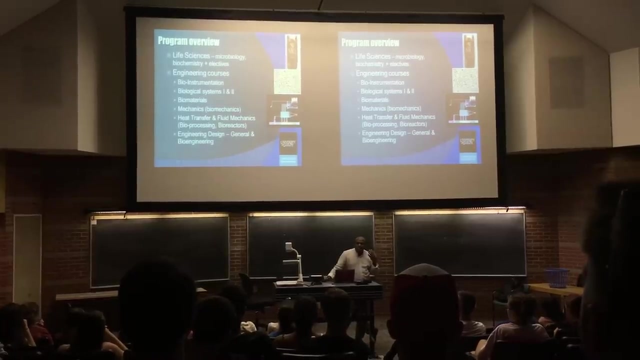 So the key courses under the umbrella of biological engineering program includes bioinstrumentation design, which is a fourth year course, biological systems one and two. So, for example, when I drink water, how does the water in my system converts into perspiration as I sweat here? 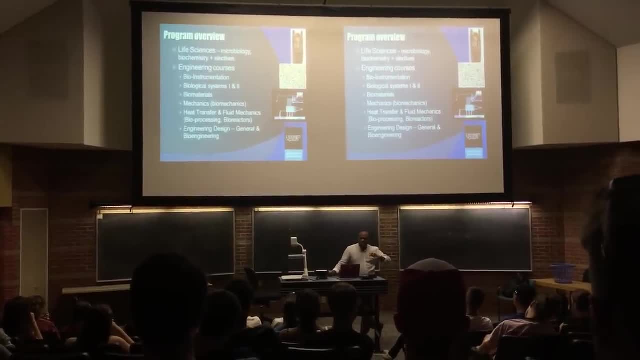 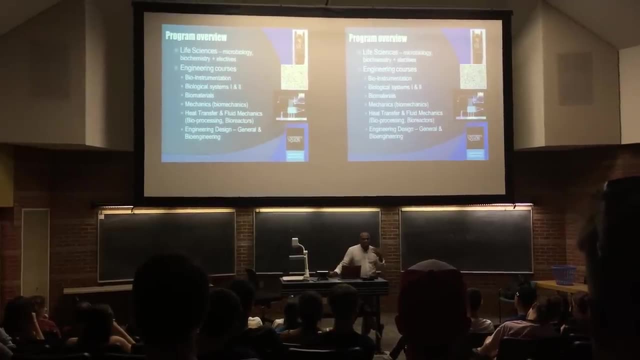 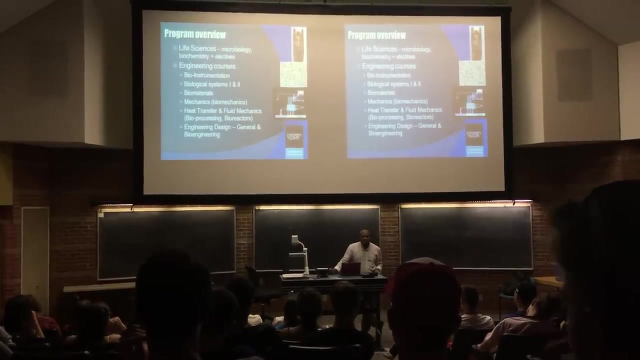 And then when you urinate, how much of water you intake becomes transformed into urine And how does the whole process happens. So the fundamental understanding, the cell uptake, the conversion processes and the mechanisms, the fundamental principles, will be taught in the biosystems one and biosystems two. 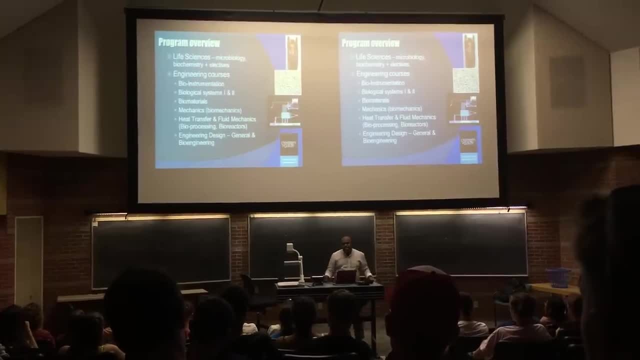 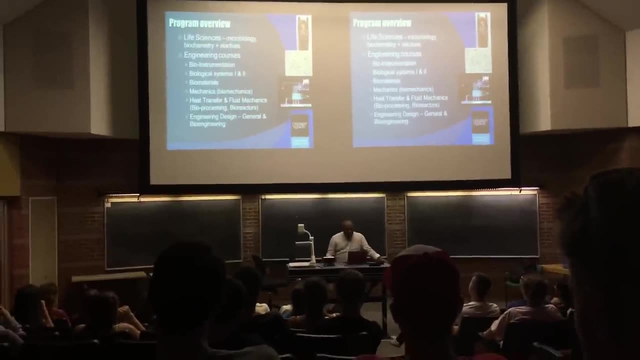 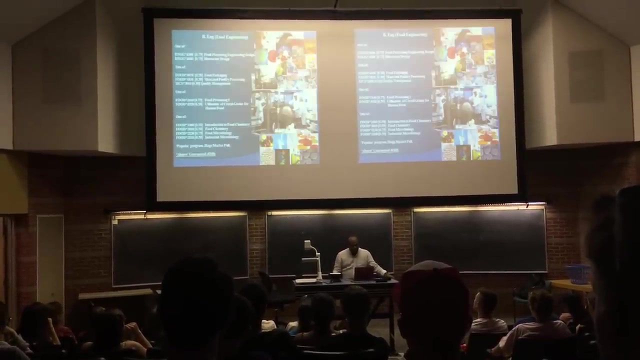 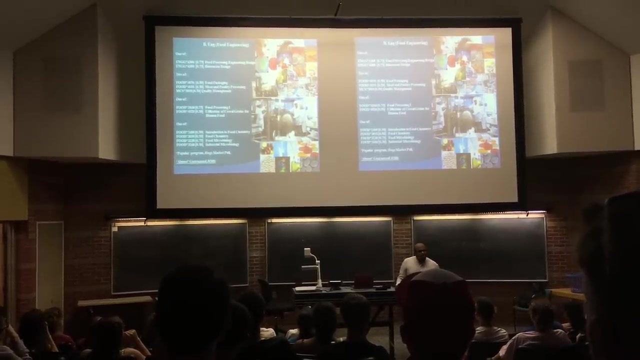 through mass transfer, through heat transfer and other related technical skill sets and concepts associated to biosystems, Biomechanics engineering design in terms of general as well as more specifically into bioengineering design. One of the popular option is food engineering: minor in food engineering. So you get a K-5 to four courses in the department of food science And in addition you also take about three to four courses here within the biological engineering program. So you get a major in biological engineering with a minor in food engineering. 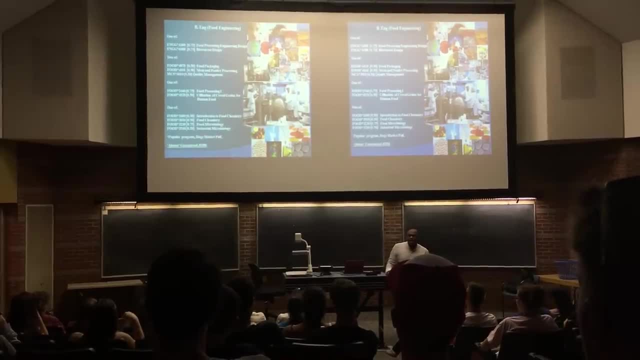 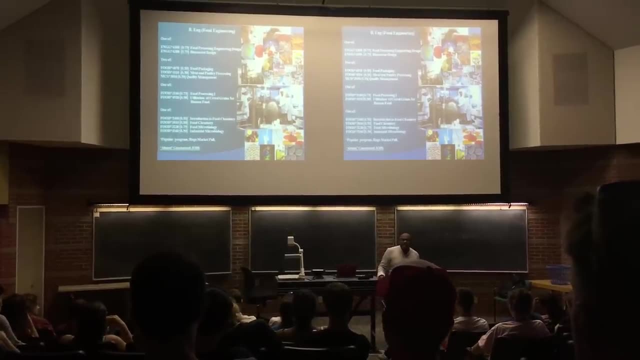 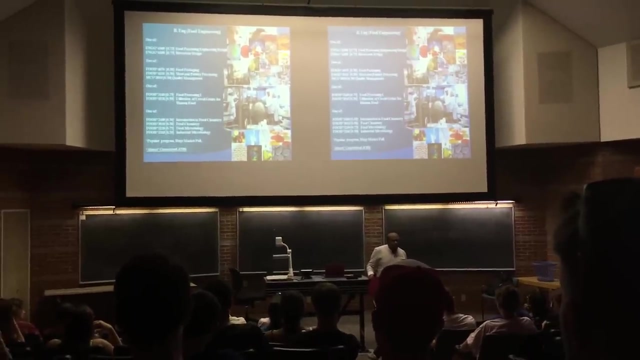 which is very popular. Main reason is your job is almost guaranteed. If you want to work in a food industry, food processing industry or a food safety related industry or a government job, then this is the better option to enroll here Today yesterday. 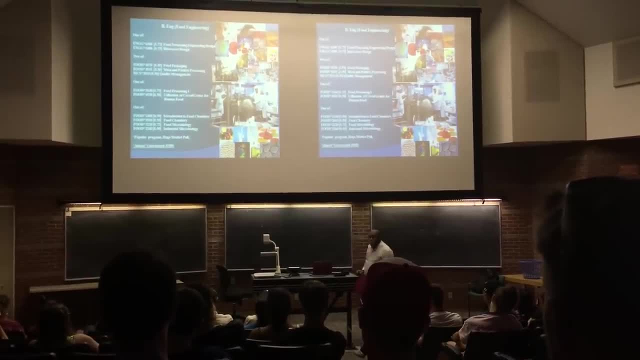 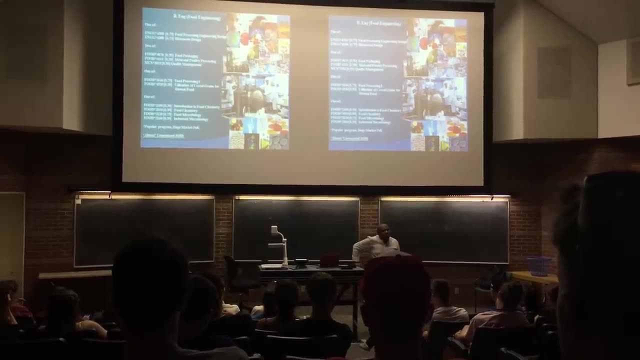 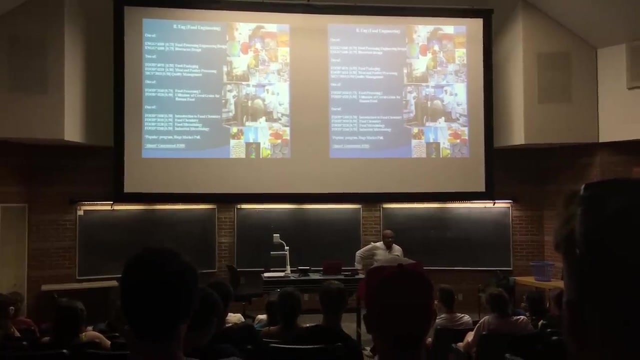 the Minister of Science Duncan announced in Waterloo that University of Guelph has been awarded $76 million. $76 million for food related activities, teaching and research to the University of Guelph. So that is a bigger funding which means that we get translated into different levels in terms of reviving. 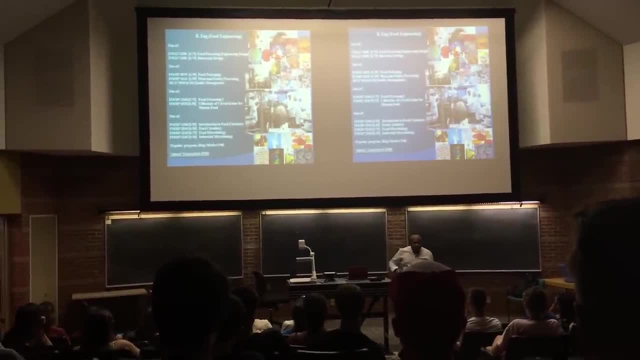 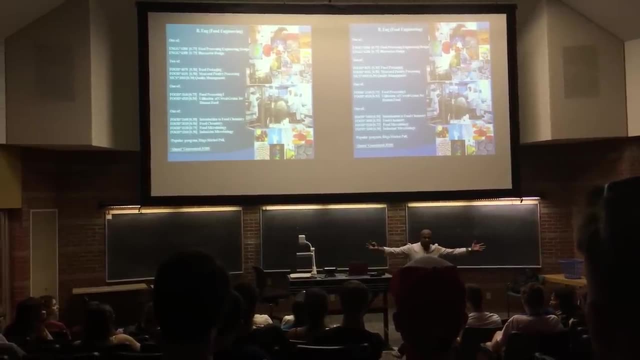 in terms of rejuvenating, bringing up the food engineering, the food engineering program within the school of engineering. So again you look at a big country. Canada is the third largest country by area in the whole globe When we look at Southwest Ontario. 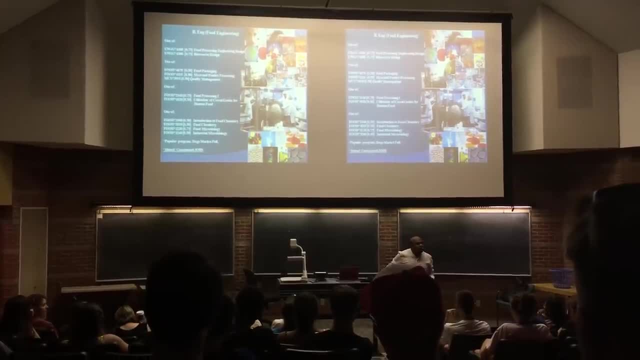 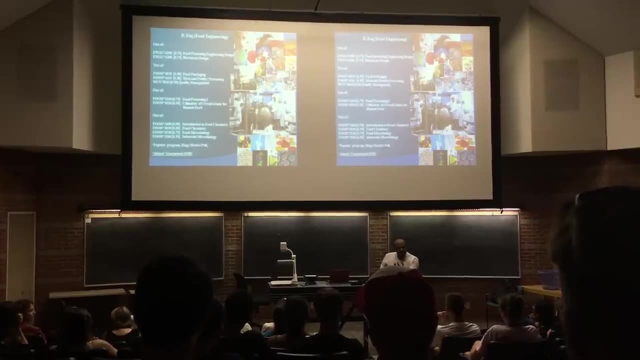 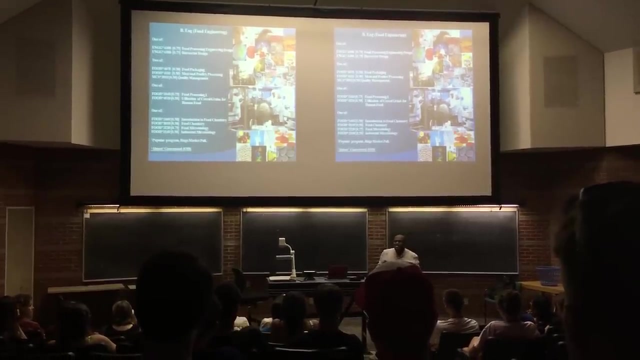 we have about almost 800 food manufacturing and food processing industries within Southwest Ontario. It is the hub. When we take Guelph, the city of Guelph, we have about 55 key scientists, national and globally recognized, highly achieved scientists, within the city of Guelph. 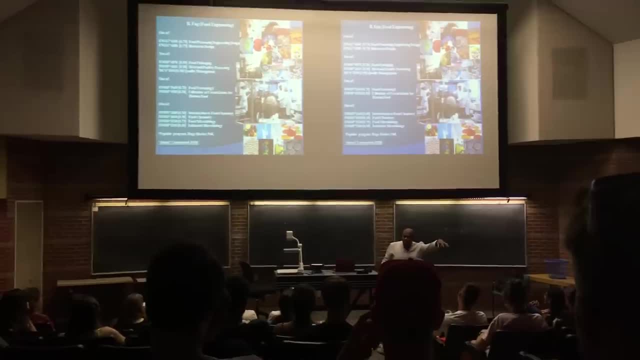 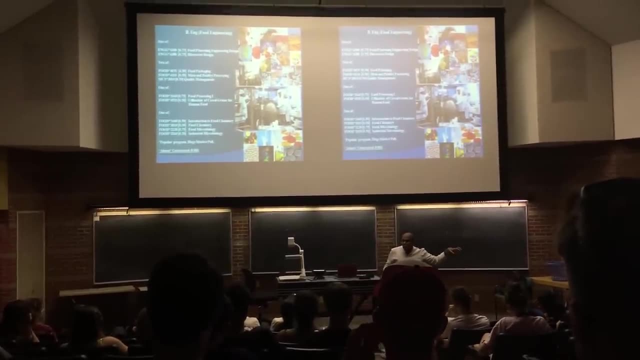 So not only within the University of Guelph, we have Agriculture and Reef of Canada, Guelph Food Technology Center and the OMAPRA Ministry of Agriculture, Food and Rural Affairs. So there is a very much high level expertise available within the city of Guelph. 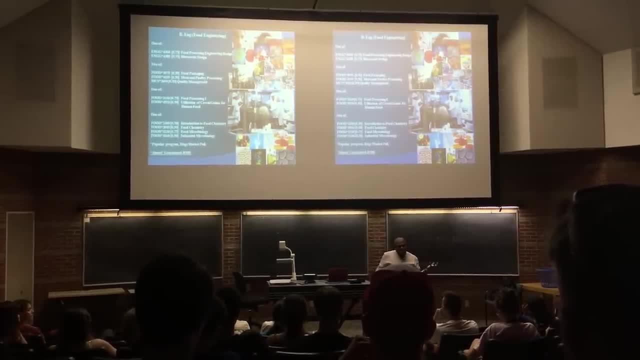 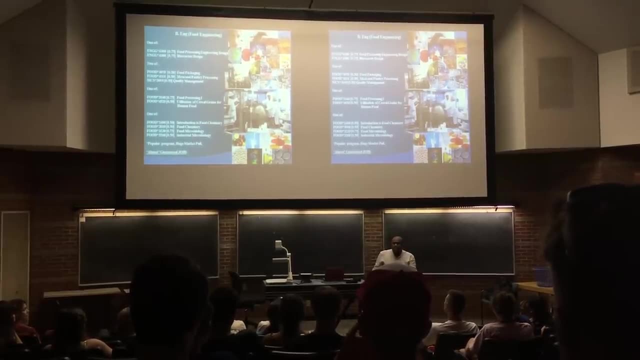 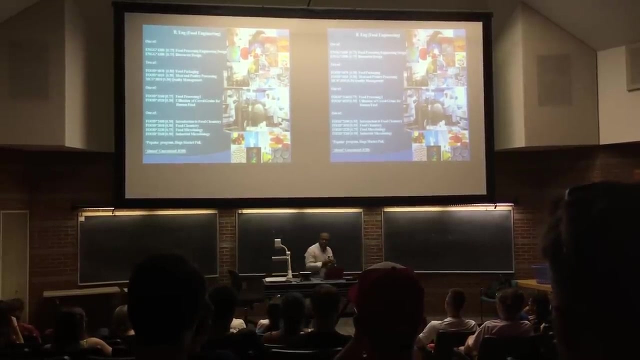 which you will never find in any other parts of Canada. So the city itself is designed in such a way to offer novelty, to project itself as a hub for food engineering, food related research. So, the three undeclared folks, you may want to consider enrolling into food engineering. It's very popular because of the type of courses you will be taking in food science department. You will be actually dealing with a variety of foods: ice creams to cheese to what not. There are 3D food printing and so on and so forth. 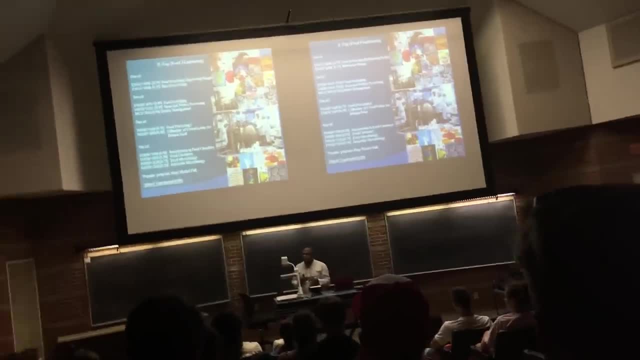 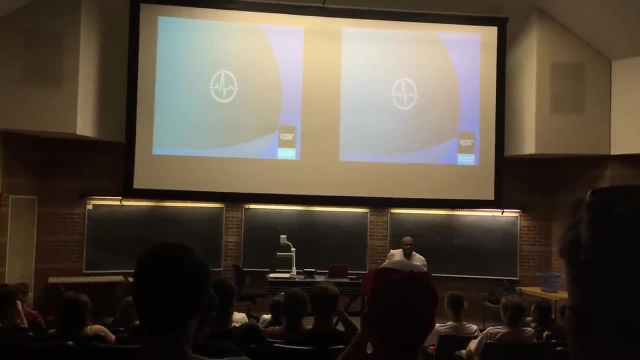 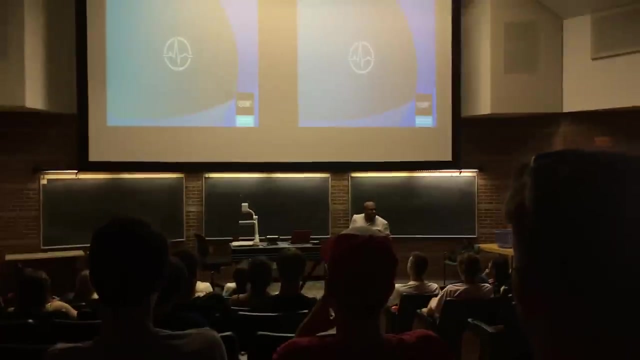 So there is a lot of infrastructure, a lot of new avenues available in the food engineering option. You can see the logo here. This is a biomedical engineering logo. What exactly is this? What is that? Yes, Electrocardiogram, Cardiogram- yes. 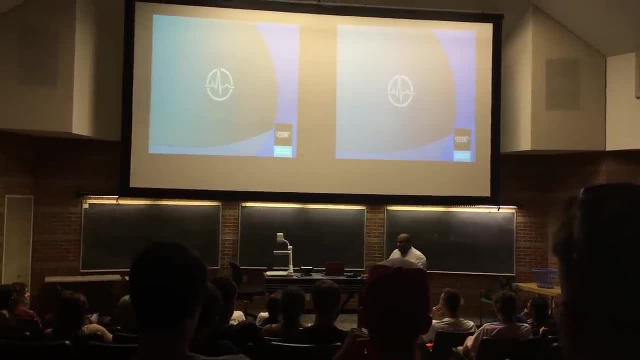 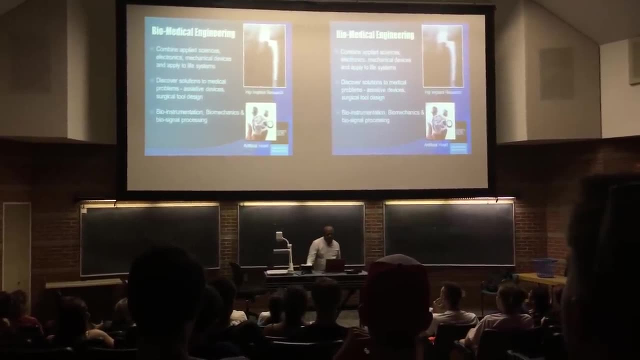 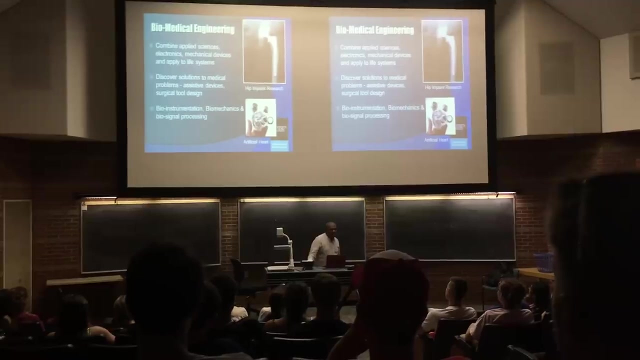 So it could be a signal output from an ECG or EMG Cardiogram could refer more closely. So the biomedical engineering program combines applied sciences, electronics, mechanical devices and provides solutions to life sciences. So when we look at the whole bigger umbrella of biomedical engineering, 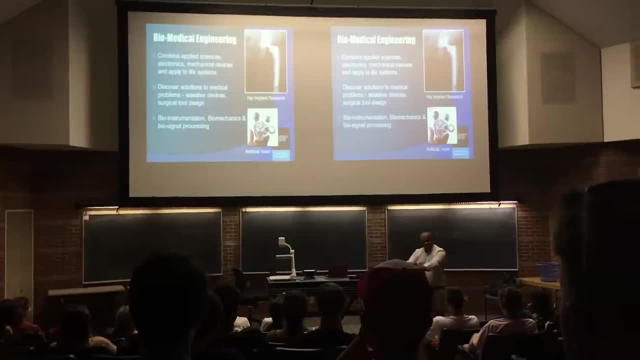 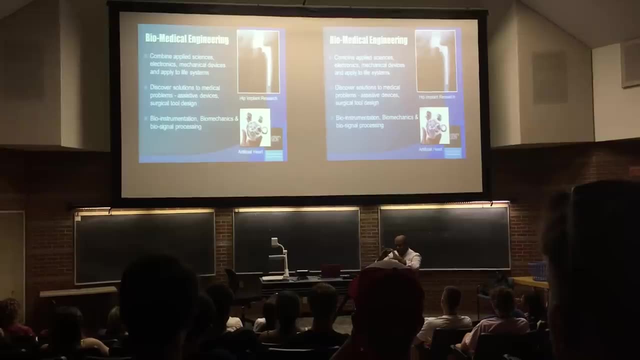 we can divide it into two units or two sections Stream: one primarily electrical oriented. So when we list the courses under electrical oriented, we have medical imaging modalities, signal processing, instrumentation, design. These all come under electrical oriented, These all come under the electrical oriented courses. 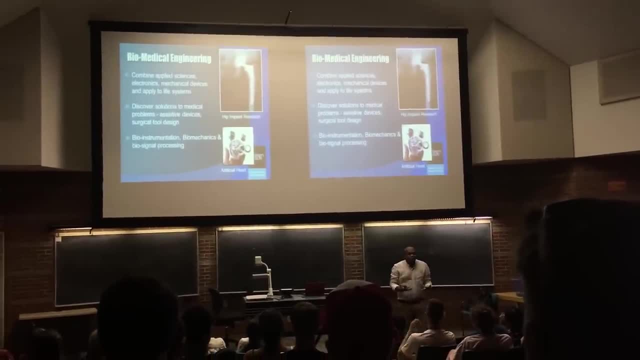 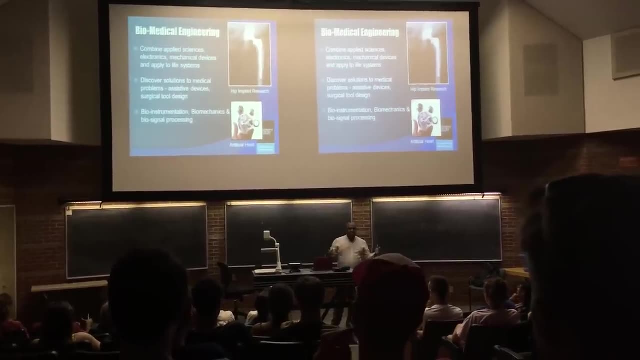 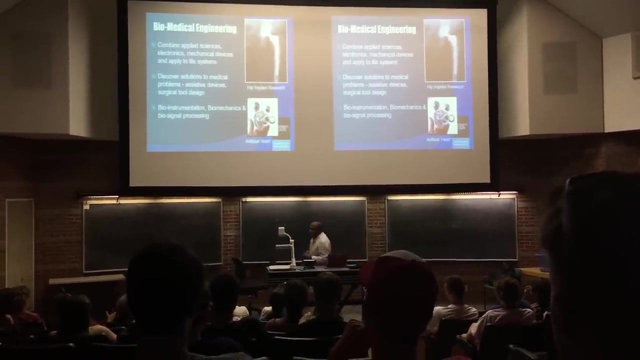 When we look at the mechanical oriented courses, we have the biomechanical, biomaterials, mechanics two and so on and so forth. So we can generally divide, but also there's a little bit of chemical aspects to it, If you happen to take additional electives related to biochem. 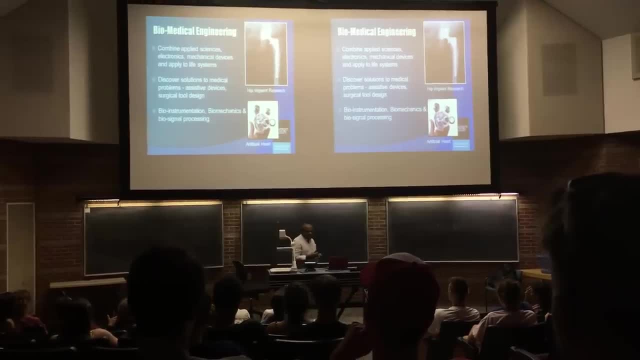 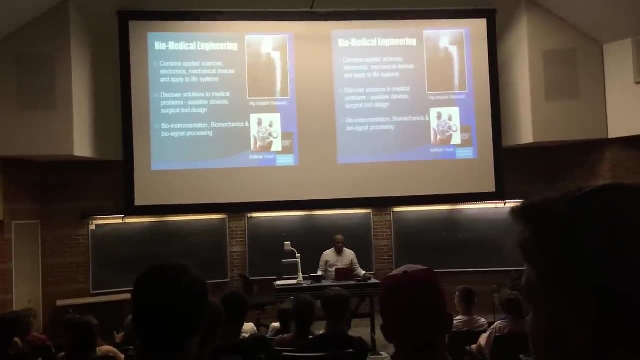 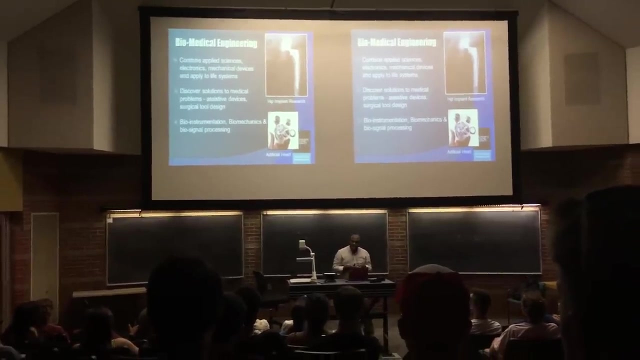 then you also get to have a flavor of chemistry or biochemical related knowledge and technical skillsets as you build on to become a biomedical engineer. So bioinstrumentation design, biomechanics and biosignal processing- These are the top three courses in terms of the flavor. 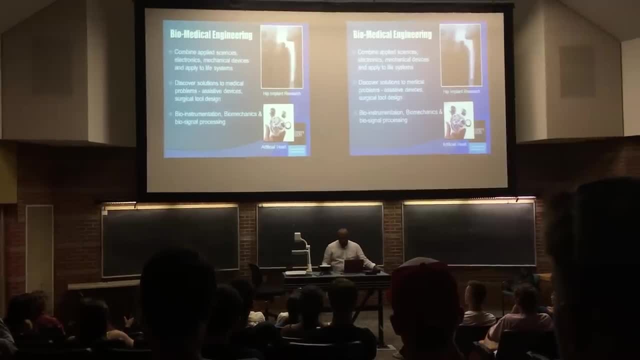 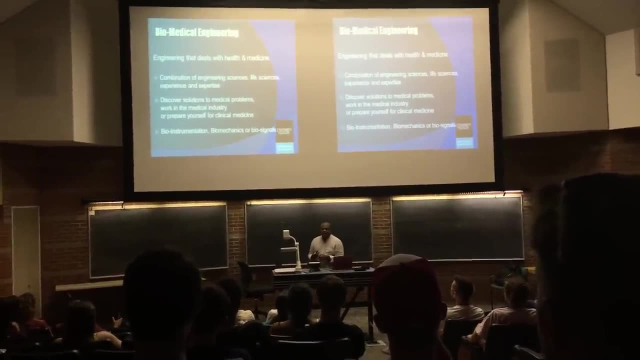 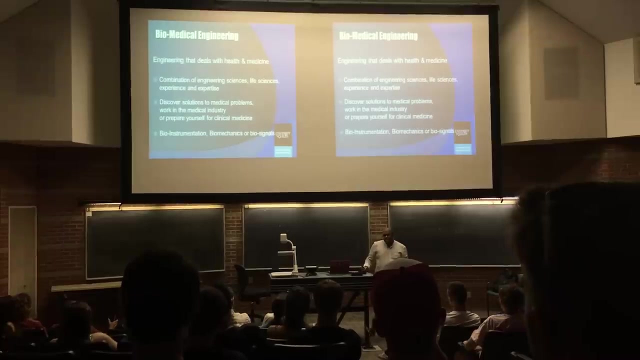 that is being provided in the biomedical engineering program. So once again, it's a combination of engineering sciences, life sciences and experience and expertise. Because of the very heavy focus on design aspects, we are going to see a video at the end of today's presentation. 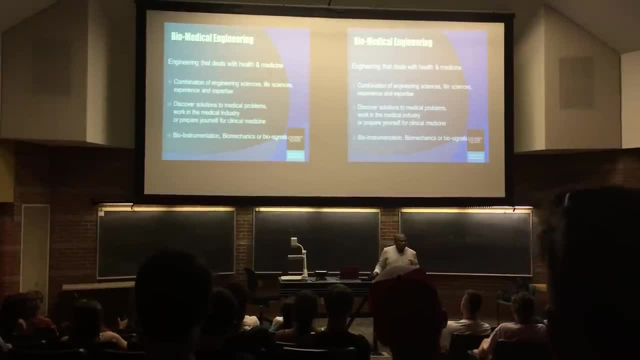 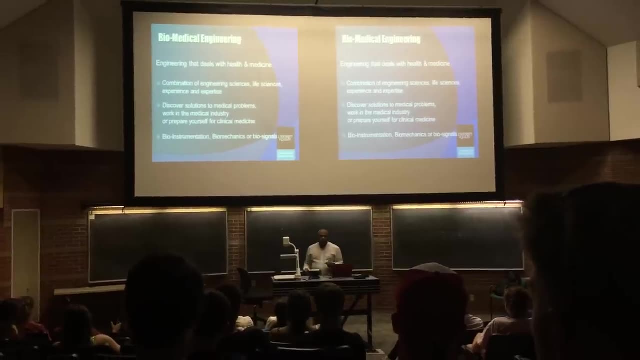 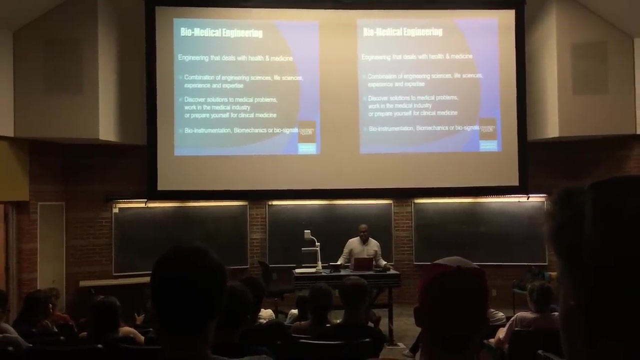 just to have a glimpse of the type of project students do here as they move on during the third and fourth year of the biomedical engineering program. So they do solve real life problems using the concepts they learn in the courses, For example in the third year level. 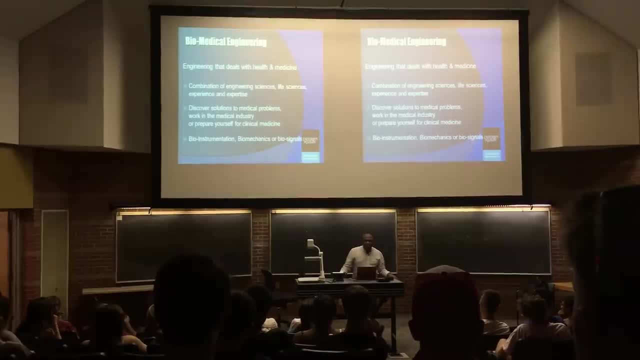 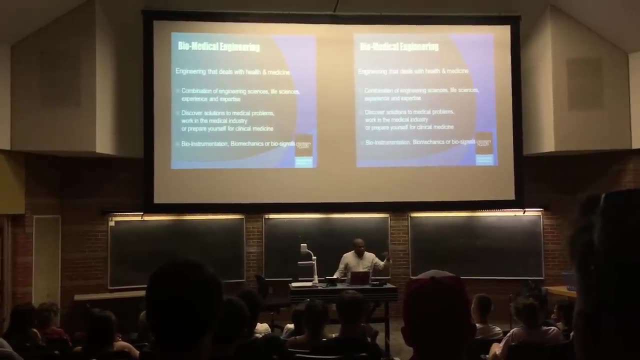 biomechanical engineering design. a couple of years ago we invited a high commissioner and the Ministry of External Affairs from the Italian Trade Commission to come and judge these students' projects. The students were actually given prizes. They were really really good prizes. 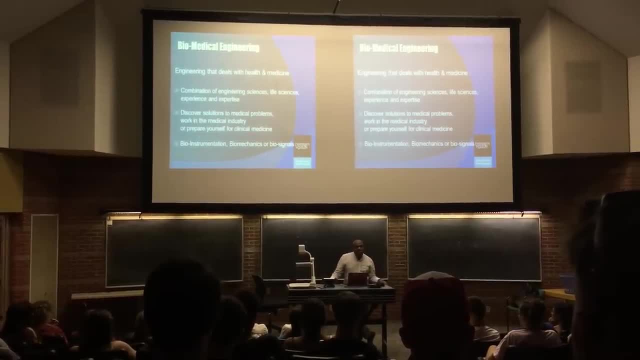 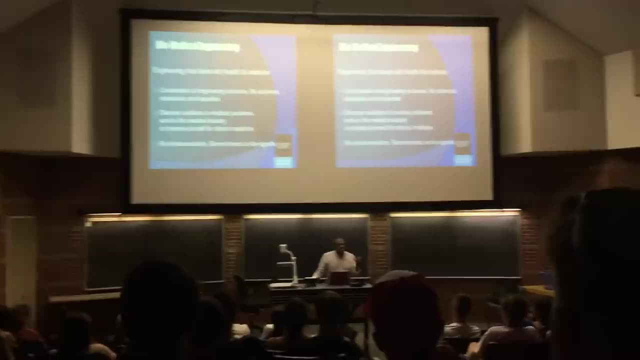 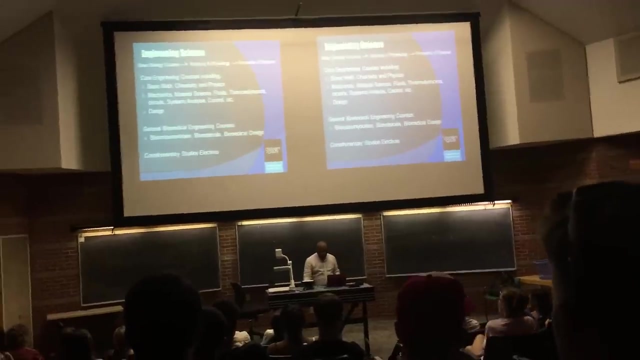 I think it was $3,000 cash for the first prize, followed by $2,000 and $1,000 cash. So they do get recognized because of the ability to solve problems in the reality and to solve problems in a realistic manner. So in the first year, engineering science. 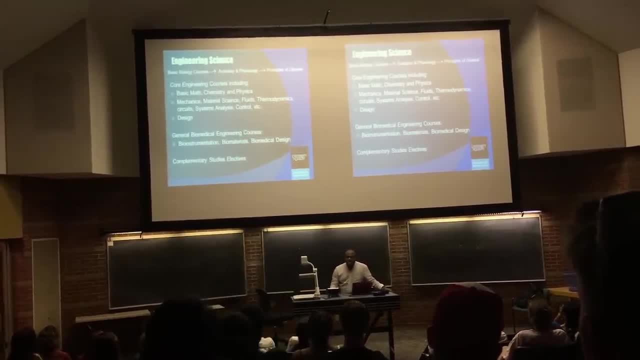 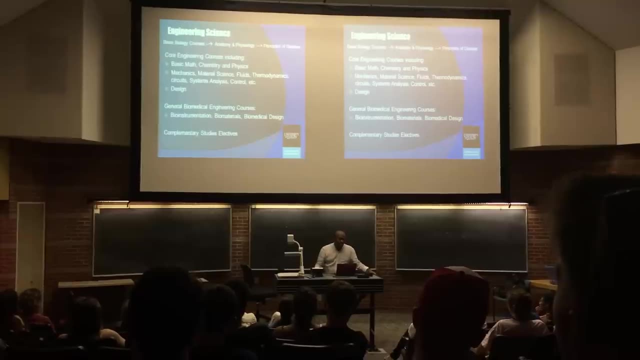 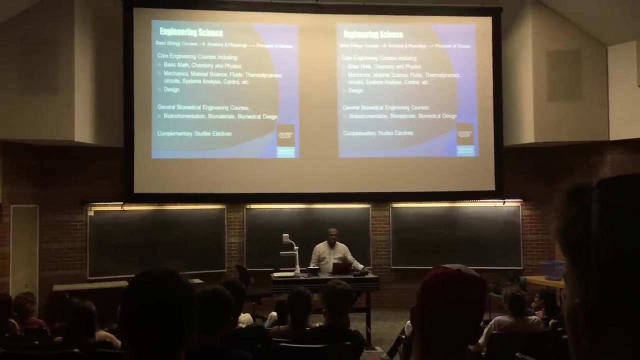 basic biology courses. For example, you get to take anatomy and physiology in the biomedical sciences department, which comes under the Ontario Veterinary College umbrella, So you get to have a flavor of how does the human body work. You do indeed really have a chance to see a cadaver. 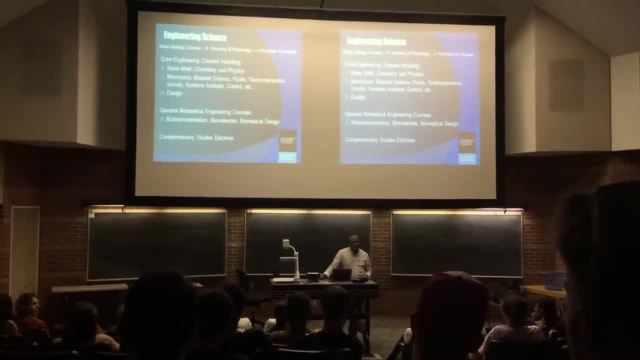 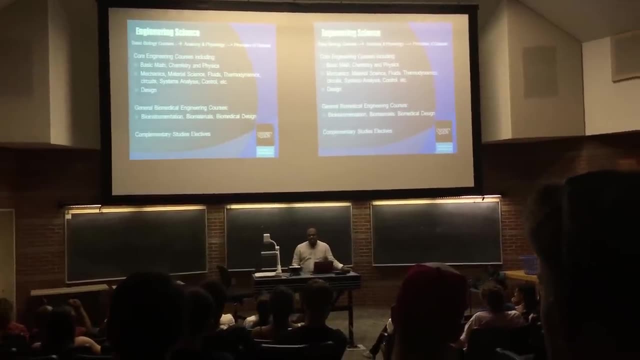 a dead body during one of the lab conferences and you are very confident as you take one of these courses. And what is the principles of disease? How does dis-ease occurs? When the body is at ease, it's ease, There is a dis-ease. 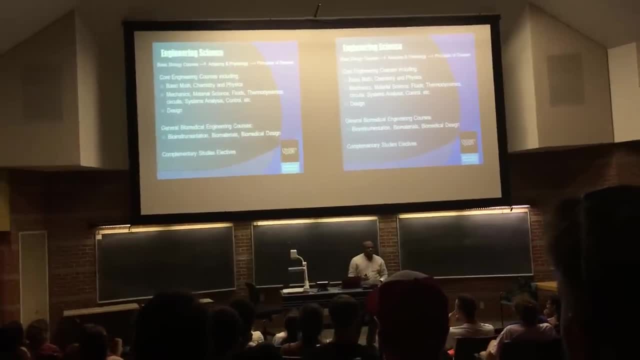 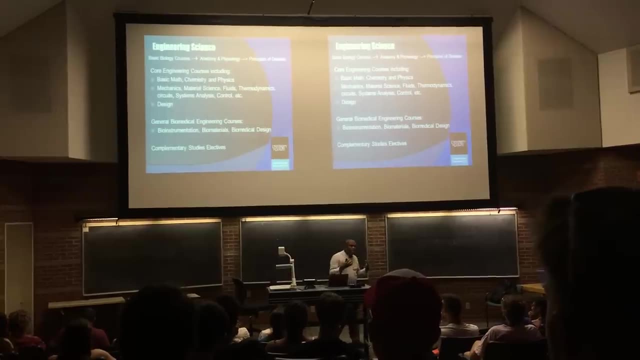 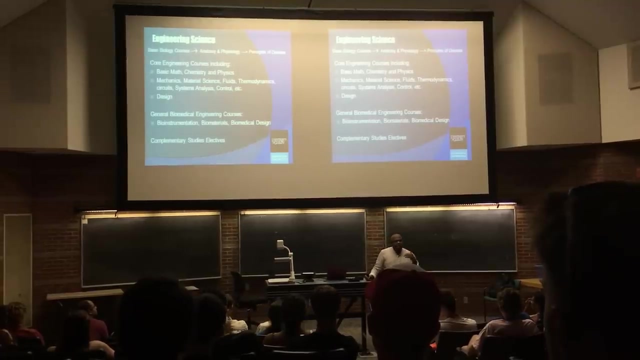 How does it happen? What is the principle behind it? What is the cellular mechanisms and the changes that occurs in the human body. So the main reason: these courses are designed strategically in such a way that by as soon as you graduate, you have a better probability. 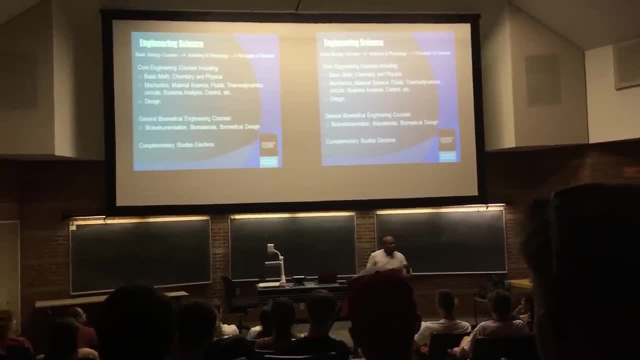 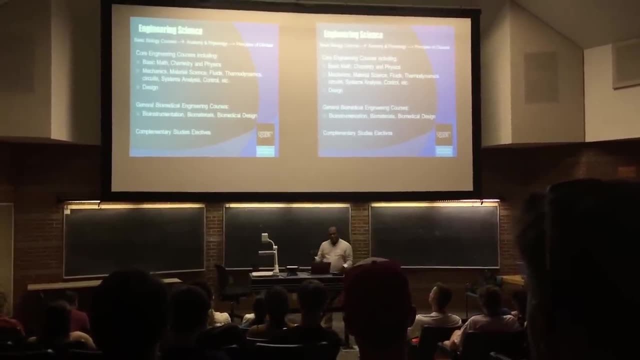 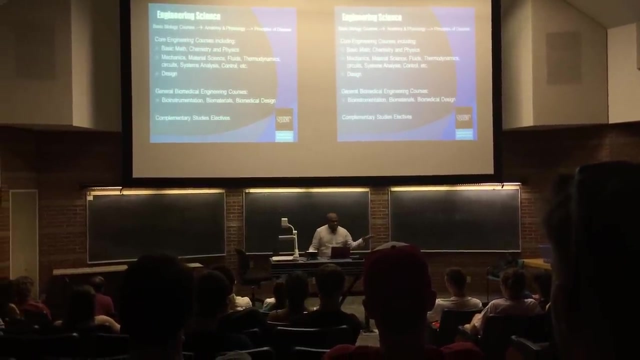 a better chance of getting admitted into a medical school, Those who have aspirations to become a medical doctor. we have quite a few folks. every couple of them, they do get admitted into medical schools. Largest dedication and sincere efforts are needed over the period of four and a half five years. 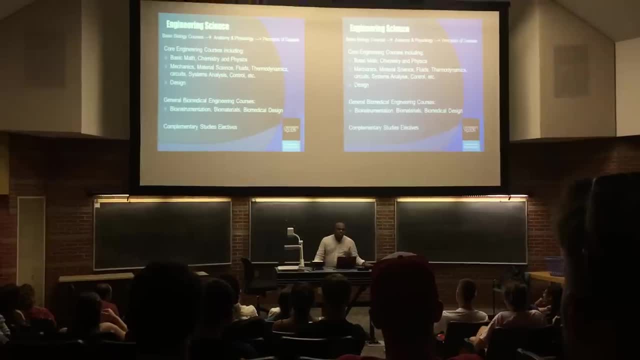 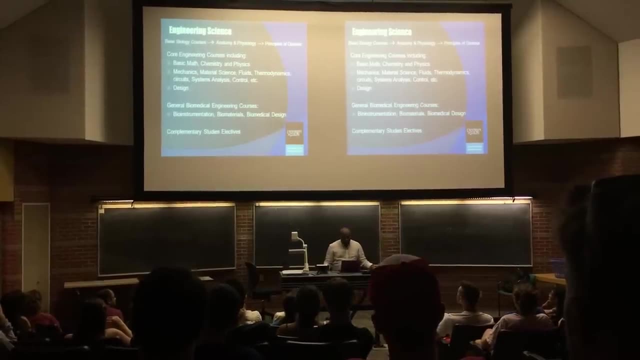 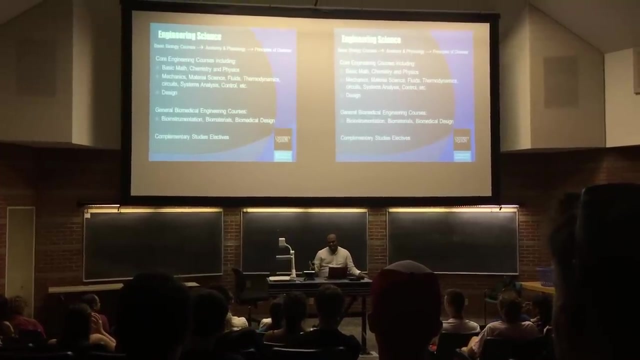 to be able to accomplish an admission into medical school. In addition, you also dedicate courses such as basic mathematics, physics and chemistry, mechanics, fluids and thermodynamics. So these courses are common in the first year level as well as second year level for all the seven programs. 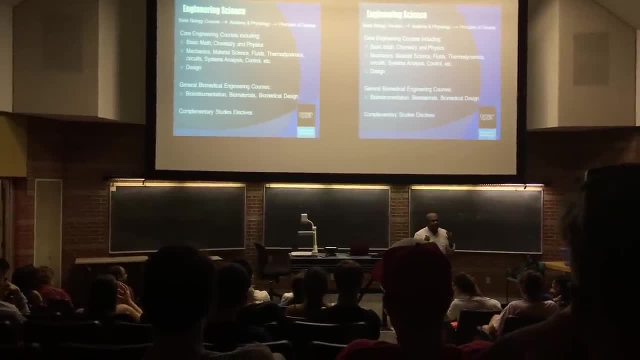 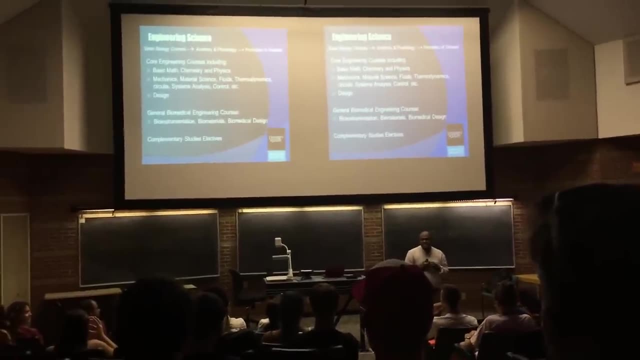 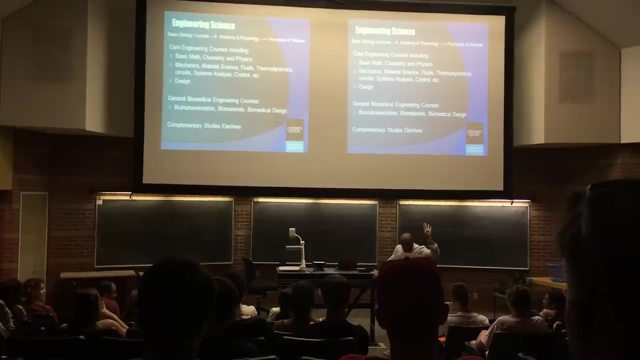 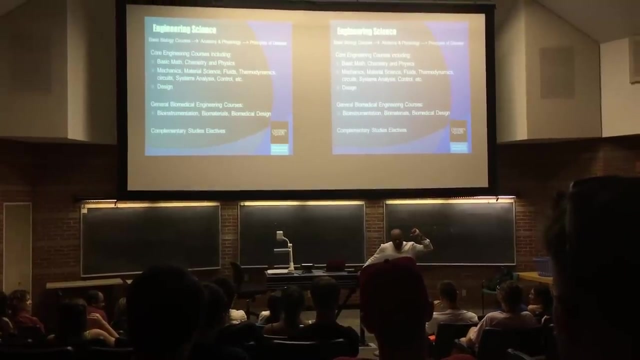 So can anyone list me or name me the seven programs within the School of Engineering? What are they? Can anybody list the names of the seven programs within the School of Engineering: Biological, biomedical, environmental, water resources, mechanical, computer engineering and there's something with the EEC. 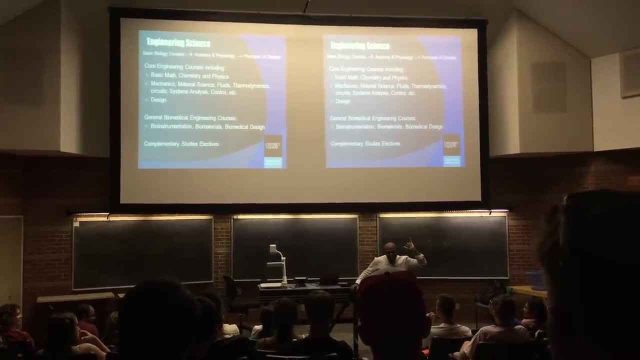 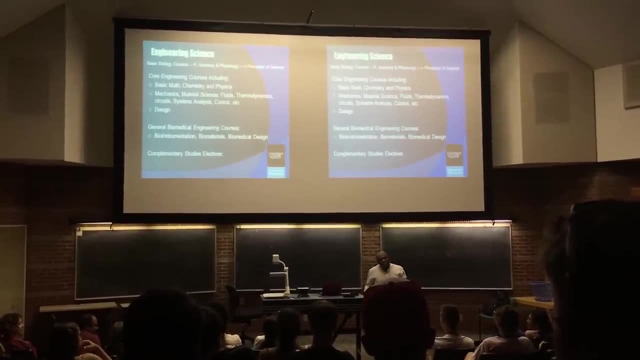 Yes, that's a weird one. yes, Engineering systems and computing. It's kind of similar to electrical. yes, So that's correct. Software right here, Computer engineering is more of a software engineering, But we don't have software engineering. 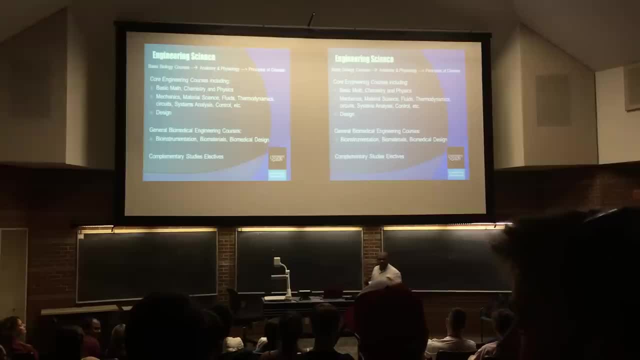 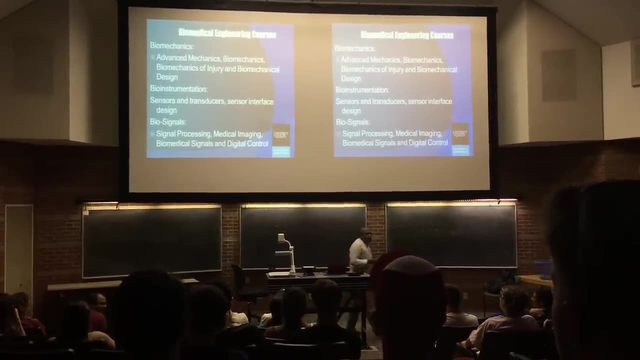 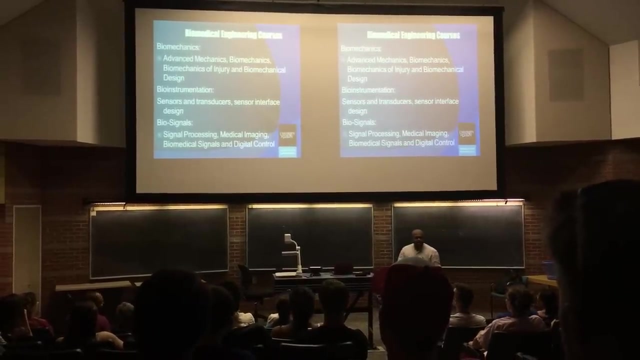 that does that It does not fall under the umbrella of School of Engineering. That's another weird program. So again, electives. So you are not. there is no restriction in terms of the electives. Please correct me, Kim. So you have a choice as you build up. 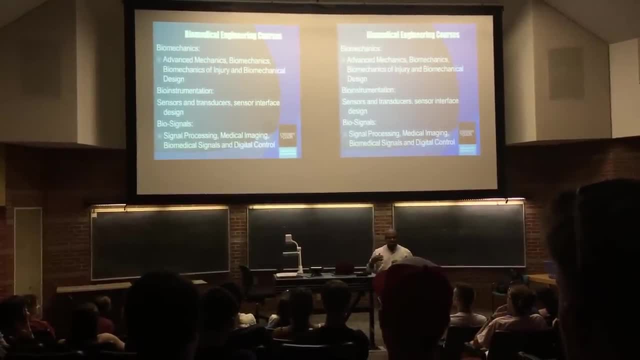 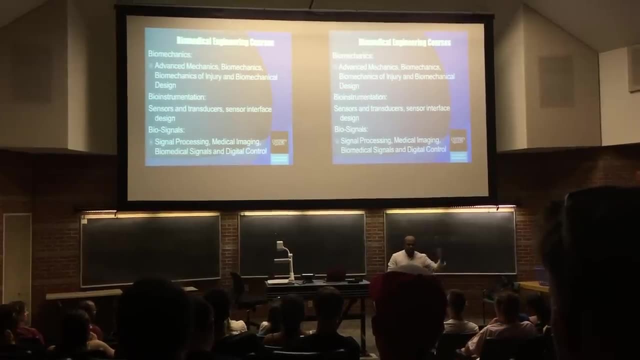 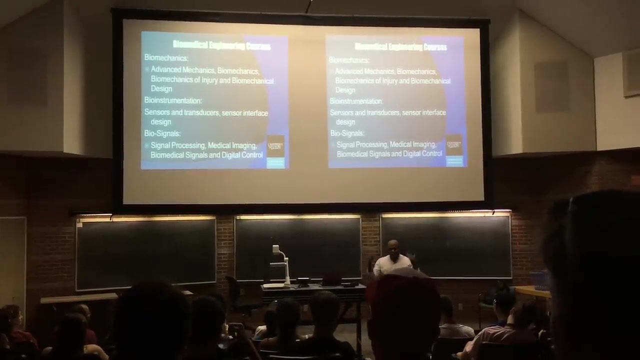 in terms of meeting the course requirements towards your degree completion. You can take additional electives if you have a specific interest. Go and take philosophy, or go and take history. go and take biochemical, For example. electrical and mechanical are the two major flavors within biomedical engineering. 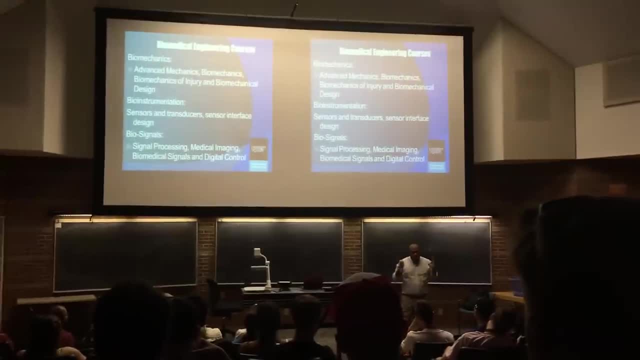 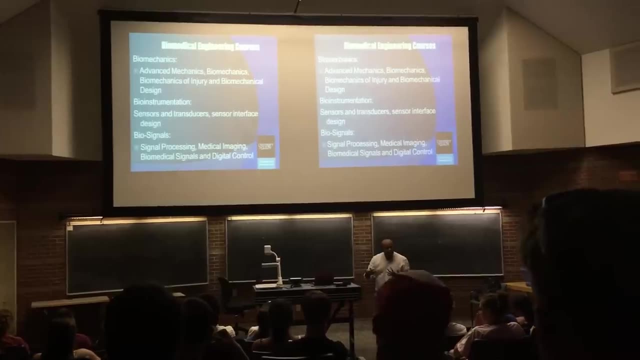 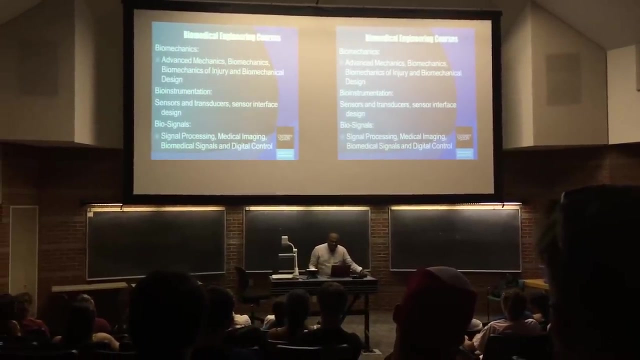 But you do feel that you want to build up a chemistry flavor to it, then you go and take courses in biochemistry or the Department of Chemistry to build on, as long as you meet the prerequisites for the particular course. So biomechanics, advanced mechanics. 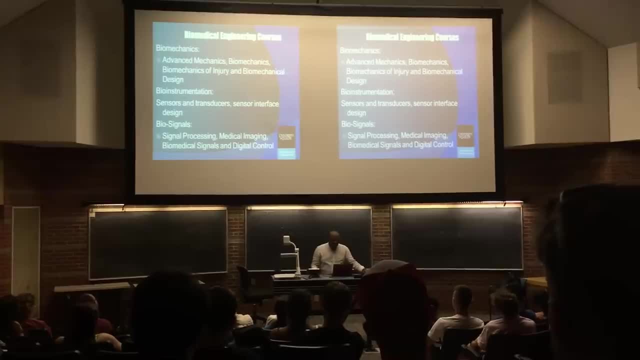 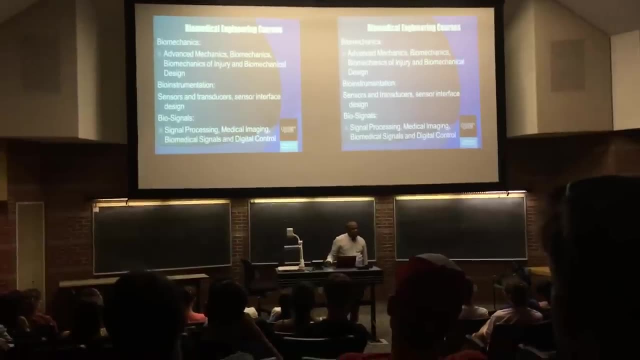 biomechanics deals with biomechanics of injury and biomechanical design. In terms of bio-instrumentation, the course talks about designing real-time sensors and transducers. sensor interface design, For example, can you be able to build a sensor? 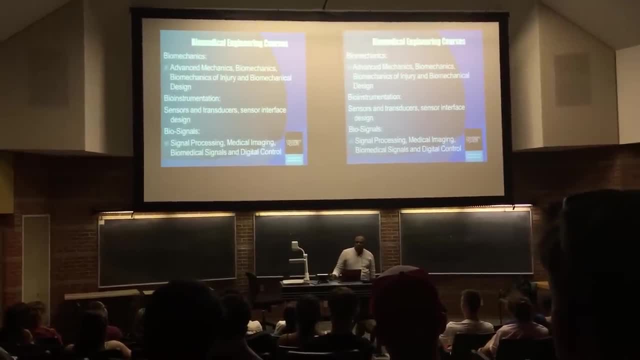 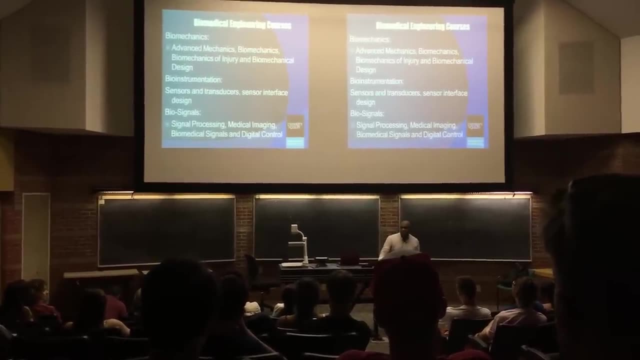 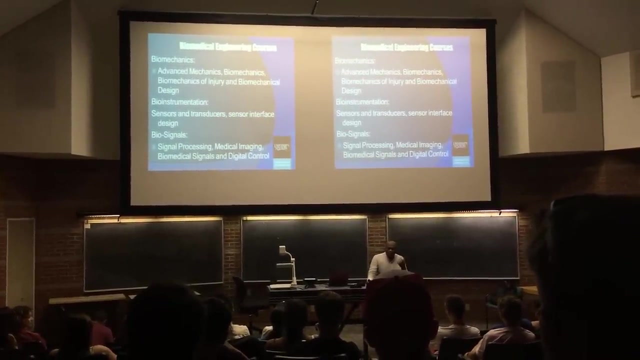 to predict breast cancer When you become 18, the female. so the Canadian healthcare system allows every two years to legally check for breast cancer. But the common technology is mammogram. but can you build a mammogram and be able to predict it just from the droplet of blood? 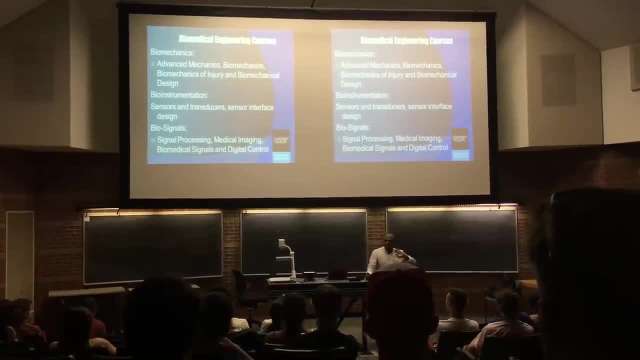 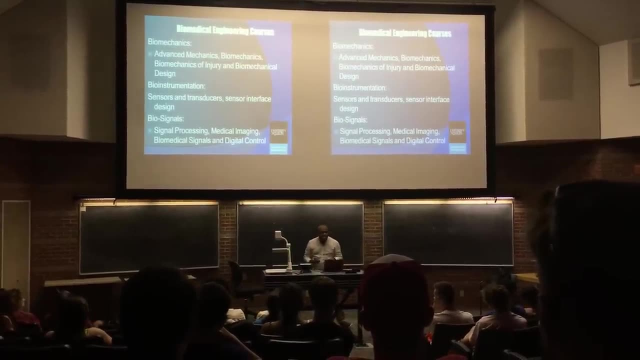 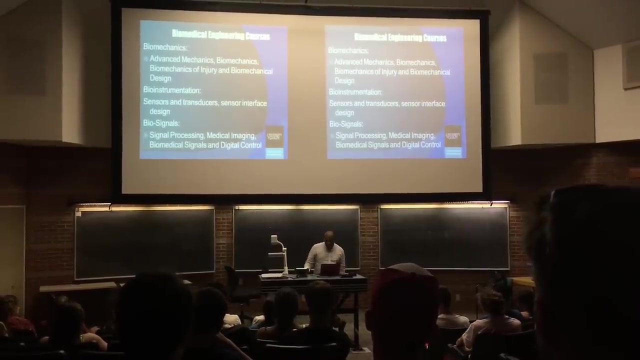 So how do we go about building a sensor to be able to predict even before it occurs? Those kind of fundamental concepts are inbuilt and integrated into the bio-instrumentation design course: Biosignals, signal processing, medical imaging, biomedical signals and digital control-related courses. 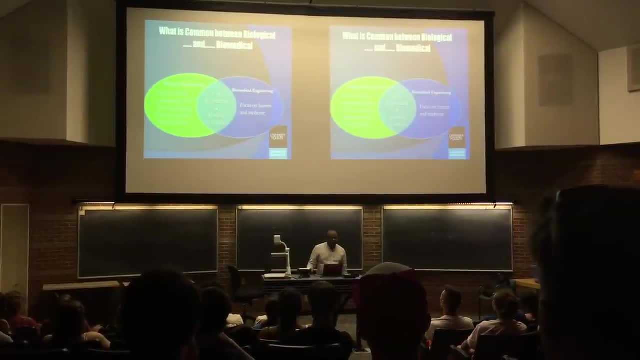 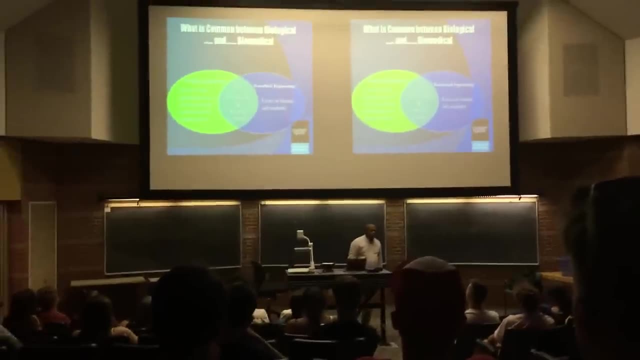 you will be taking in the upper years. So what are the common items? There is a variety between the biological and biomedical engineering program. Biological, again, is much more focused on food engineering, food safety and processing a little bit of pharmaceuticals. 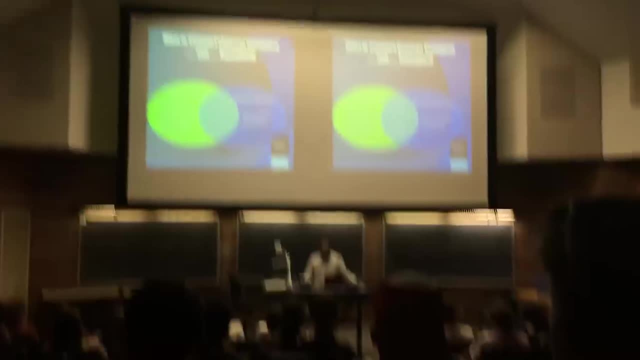 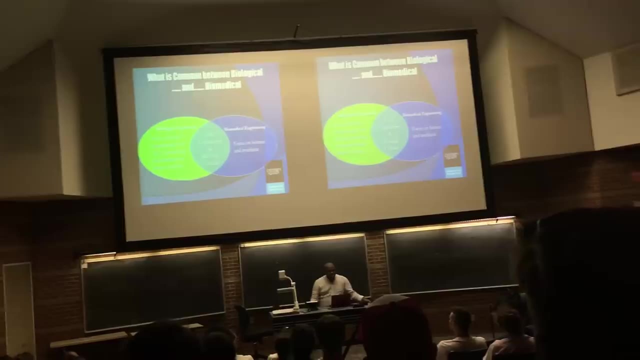 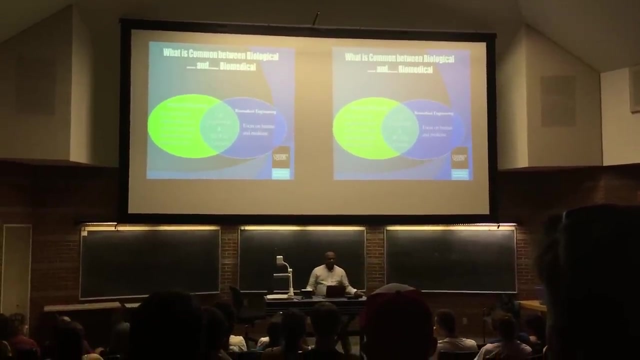 and biomaterials and human systems, While in biomedical engineering it's more focused on human health and human-based medicine-related technology. The first and second year you tend to take many, many courses similarly, Then also the third year: thermodynamics and fluid mechanics. 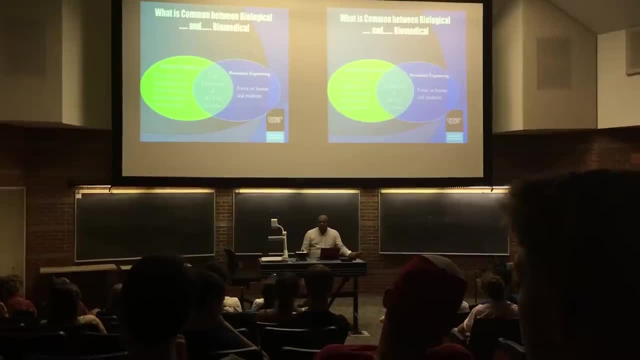 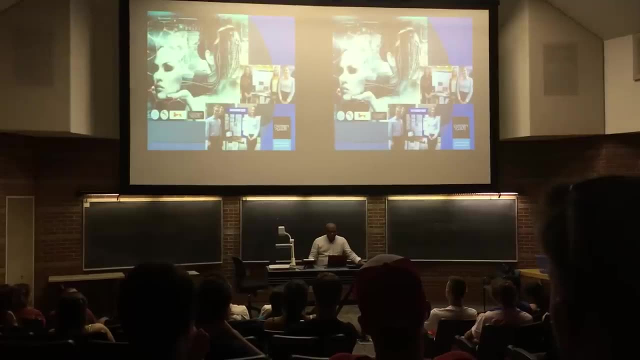 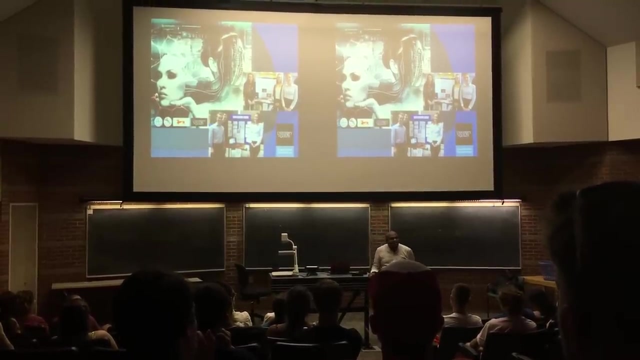 these are all the common courses you will be taking, irrespective of the type of program you are enrolled in. So where does our alumni work? They are being placed in a variety of industries- GE is one, Canadian Food Inspection Agency. different government sectors. 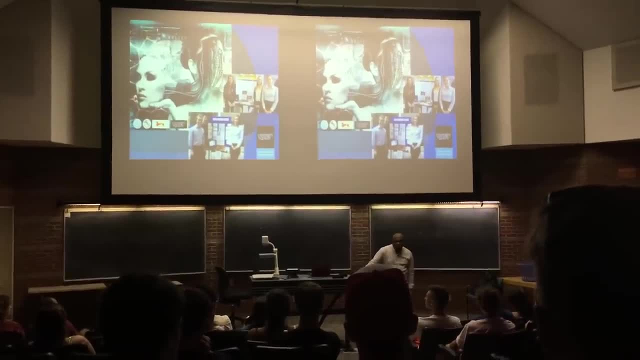 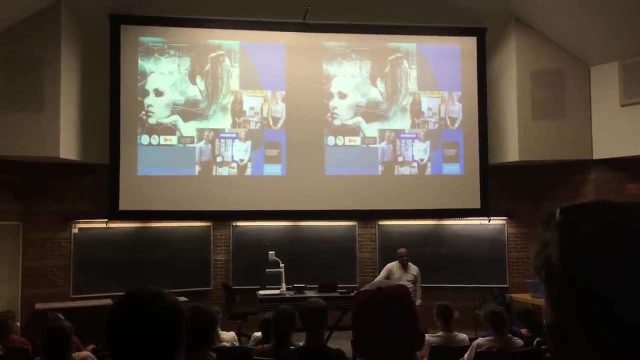 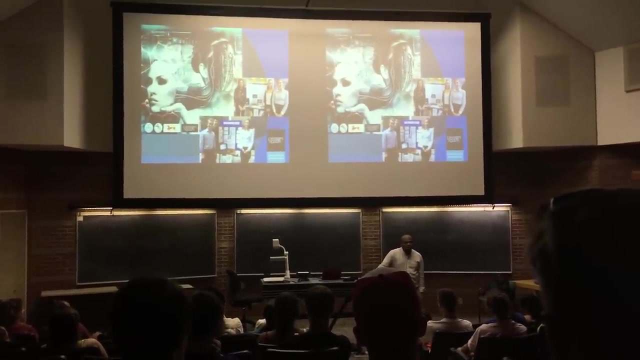 some have gone- and even you know- to medical schools. some are in graduate schools. The employment prospect and success rate is much, much higher compared to the other programs. Maybe it's a little bold statement, but it is true, mainly because the department 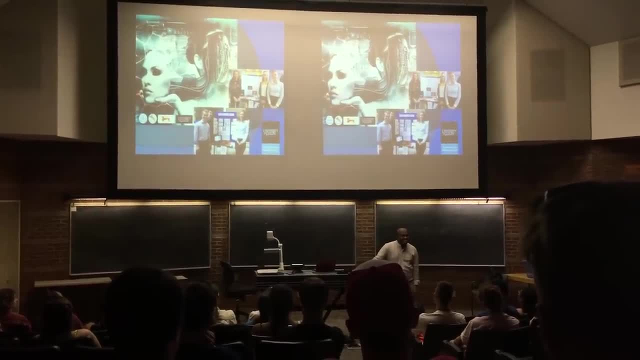 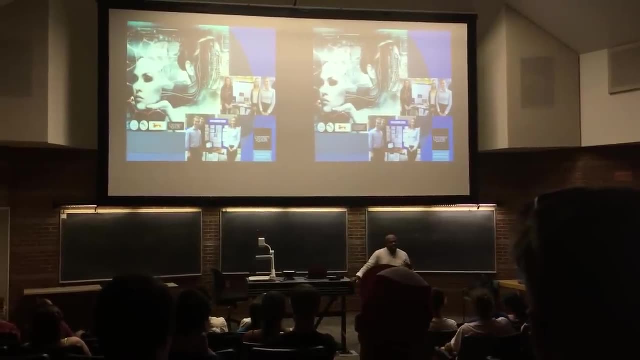 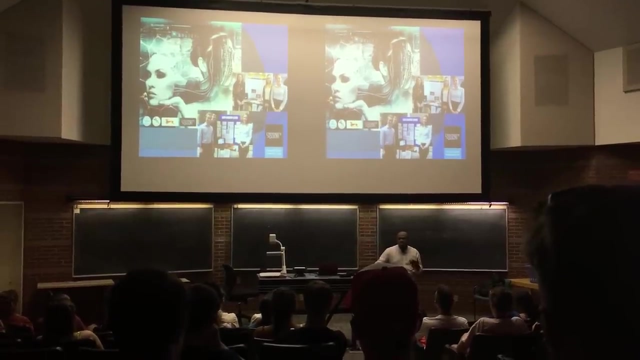 the School of Engineering was started in 1970 as a biological engineering program. So because of the long history, several hundreds of alumni are then placed at different levels. So the prospect of job and the employment is much, much brighter for biological engineers. 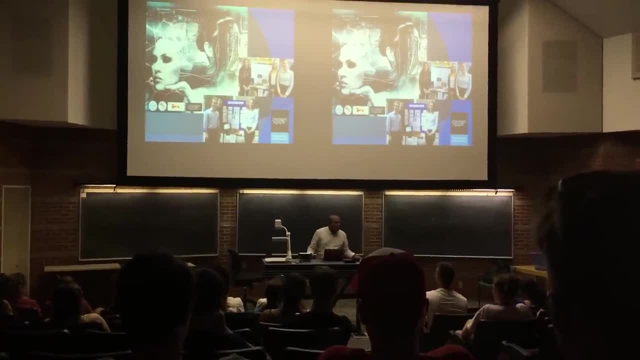 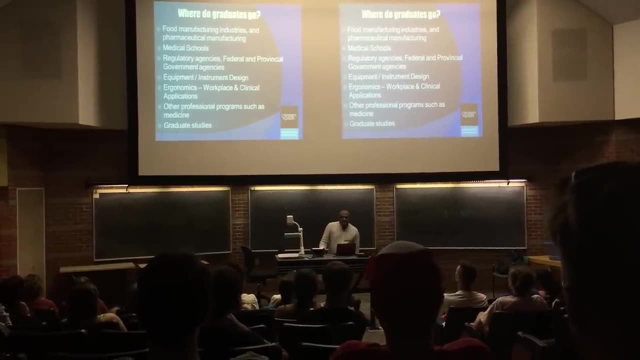 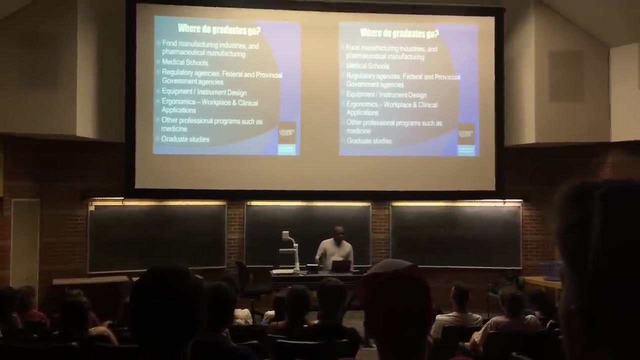 and they are employed in a variety of sectors and a variety of industries. So some are in regulatory agencies, like watchdogs, and some are in federal and provincial government agencies. Some do design, for example, Atelika Health, which is a company. 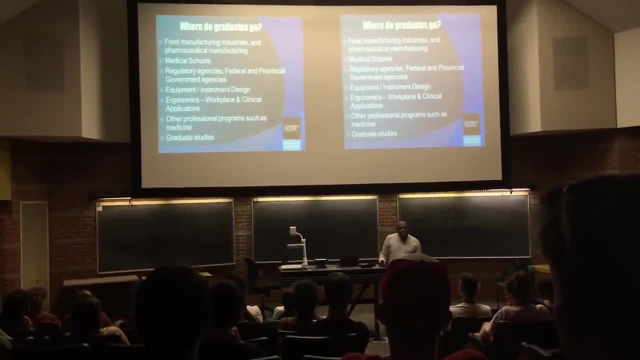 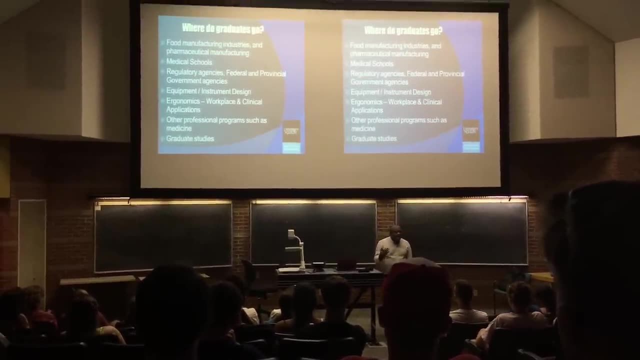 based in Waterloo. There are also a company based in Chicago. Some people do move to down south to work in private industries, startup companies, to be able to bring realistic solutions for the society. Some do work in ergonomics and other. 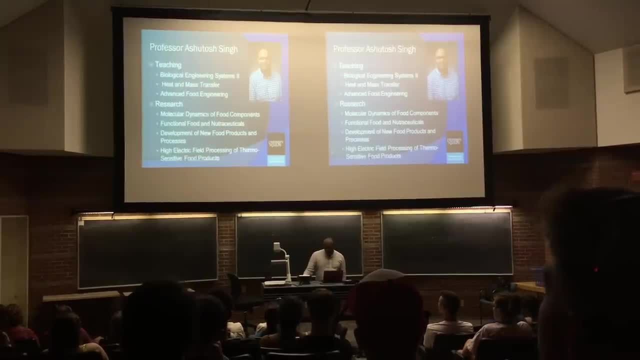 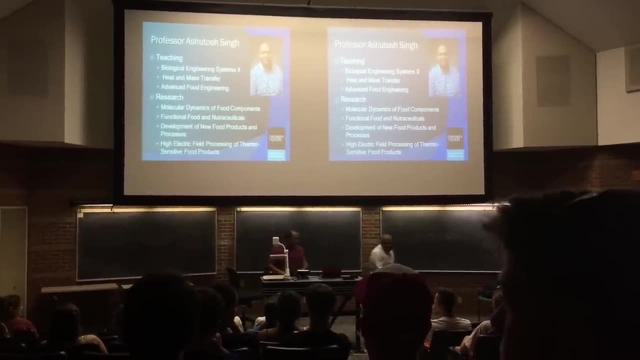 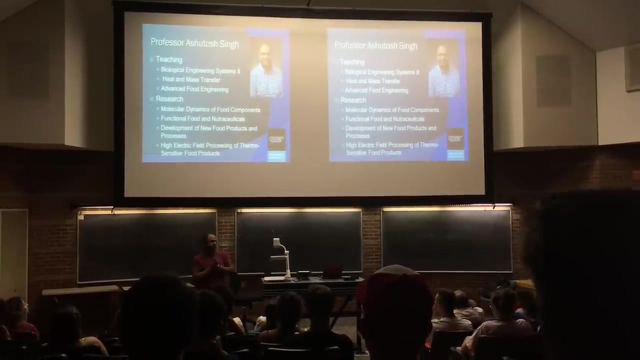 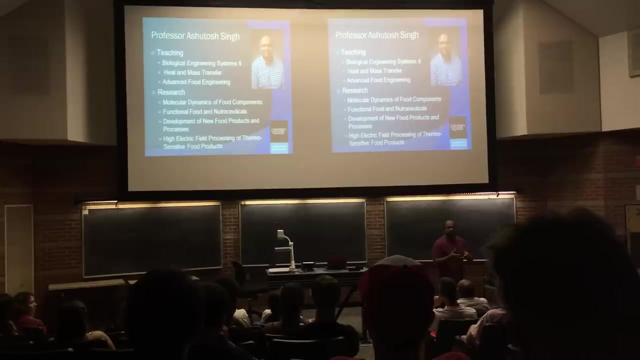 move on to other professional programs. Okay, I'll be quick. My name is Ashutosh Singh and I'm one of the biological engineering faculty here. Mostly, you'll be interacting with me in your third year, where you'll be taking the courses. 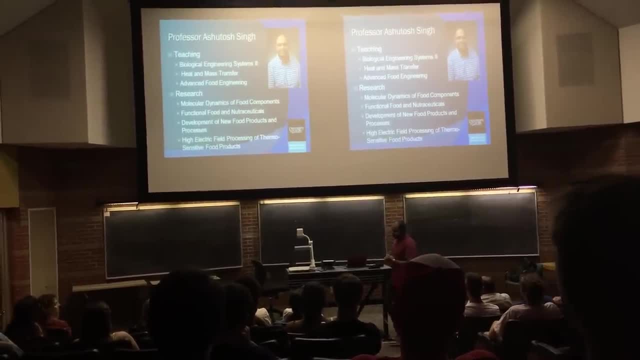 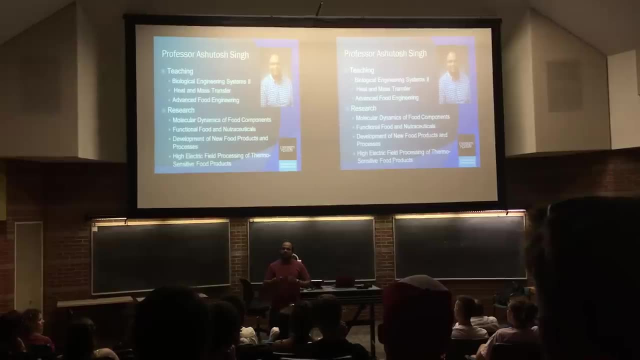 in bio-systems engineering. so bio-engineering, systems two, and also your heat and mass transfer. That's a core course. That's a core course for biological, biomedical, mechanical, any field. Now, as Dr Puresh has already explained to you, 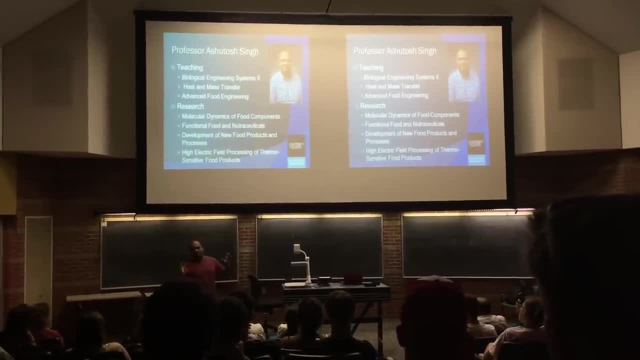 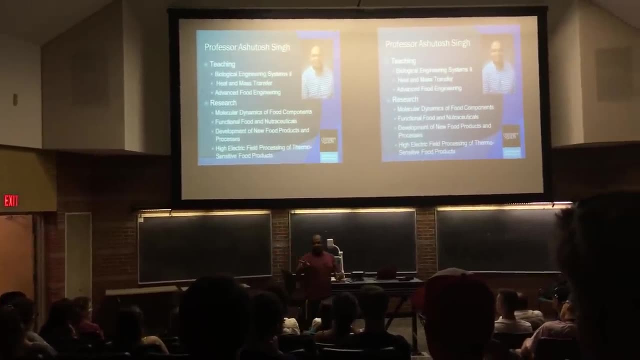 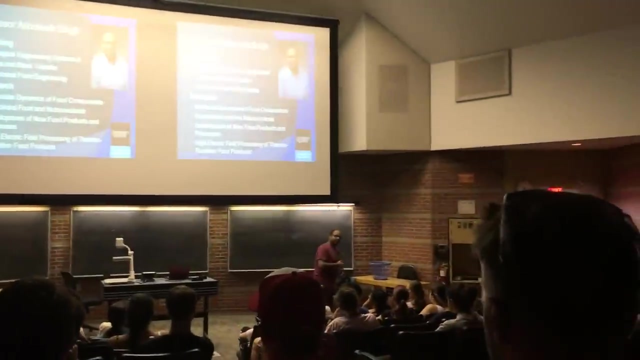 on what exactly biological engineering is. I'm much more biased towards it. Biomedical, biomedical faculty will explain to you Biological engineering and the two on the left. please join us. Biological engineering is not just food. In bio-health, you have medicine. 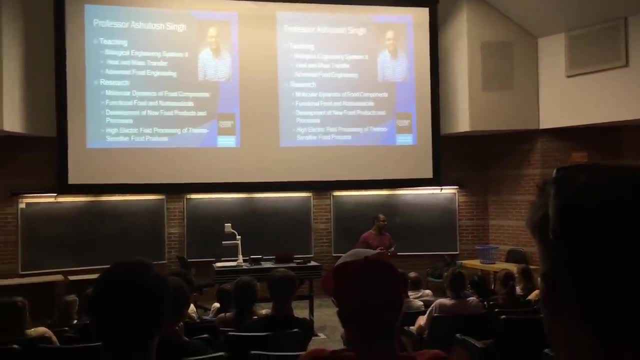 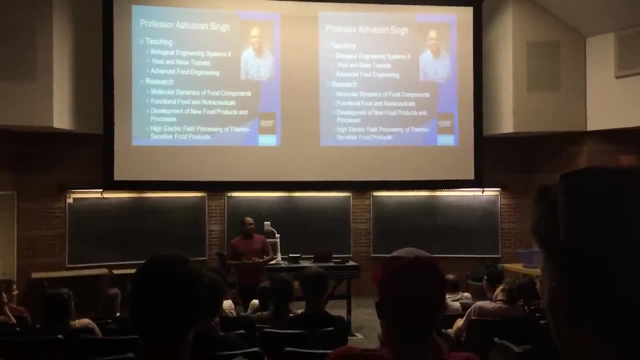 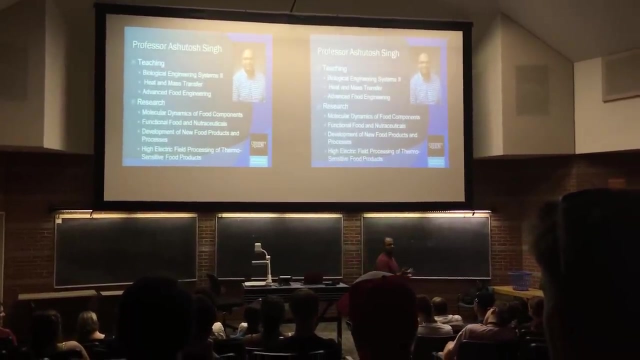 you have any other field, I'm just saying Chemical you have. So the biological engineering is everywhere. It's the mother of all the changing things. That's the way I see it, Except for mechanical, Because biological is not defined. 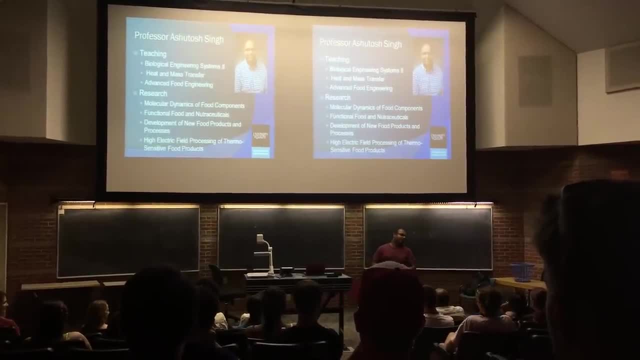 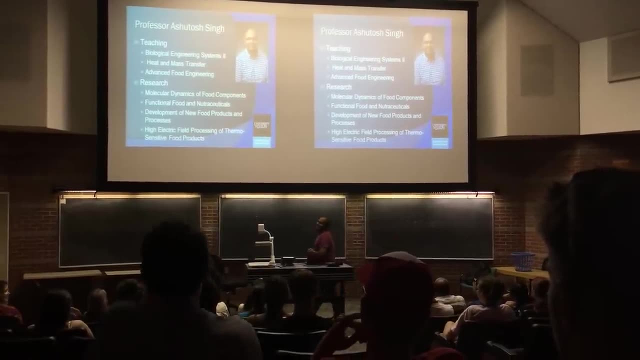 Mechanics, machine. Biological is the muscles. Just take that. I said it, you believe it and we will progress on. So that's the way. that's the way we interact with you, That's the way we'll be interacting with you. 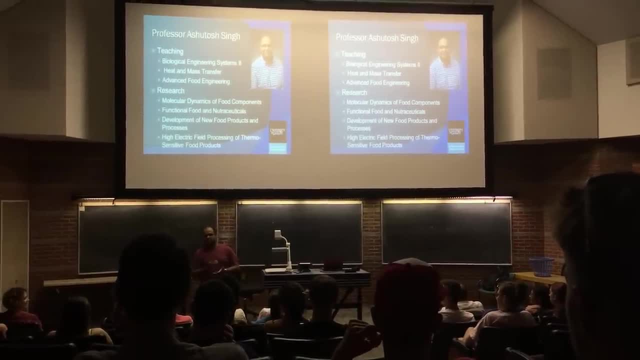 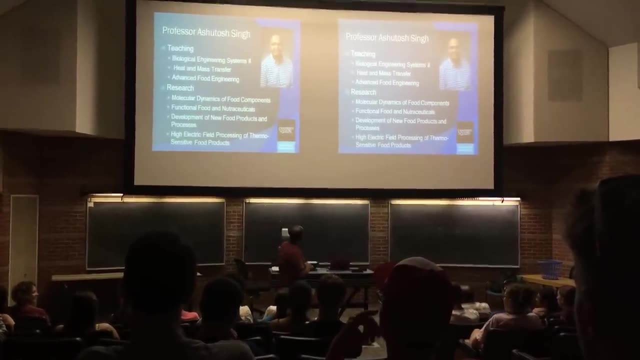 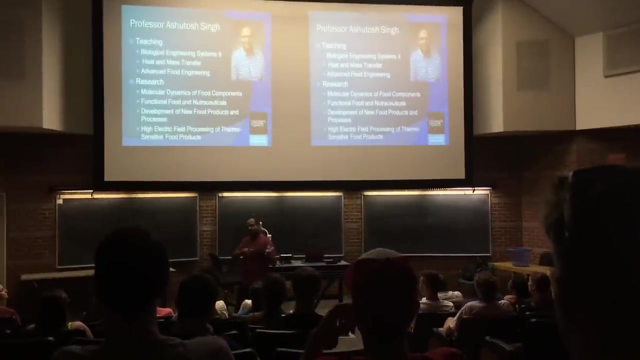 throughout your four years here. It's a school and we have a program like preparing you for the market right, So need a master Advanced Food Engineering. that's a graduate course that I teach Several of us undergraduate students from the previous 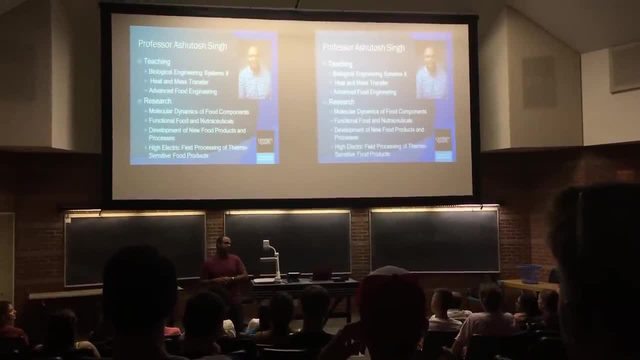 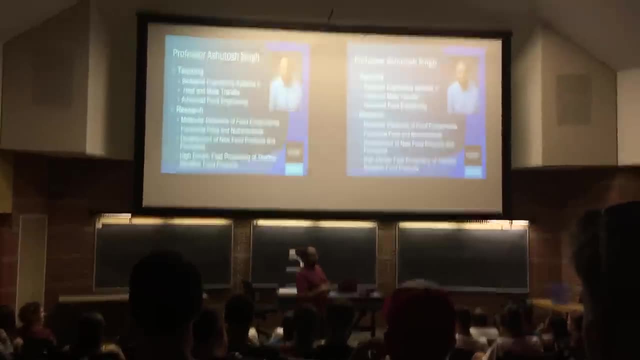 that do work in my research group And some of the undergraduate who have graduated now are my graduate students. I will be interacting with you a lot. if you want to work with me, You can talk to me later on. Research-wise, I work on. 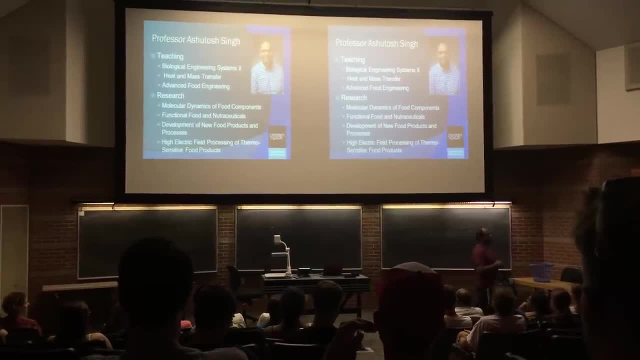 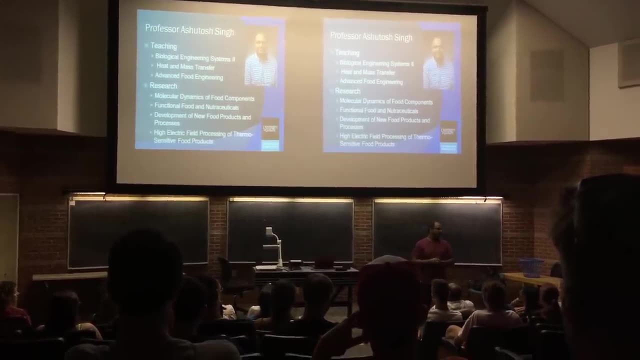 diet and food components. So this is more related to biochemistry, Food chemistry, how proteins? you have heard about proteins and carbohydrates. So when you put something in a microwave or if you're frying something, how does it change the component? 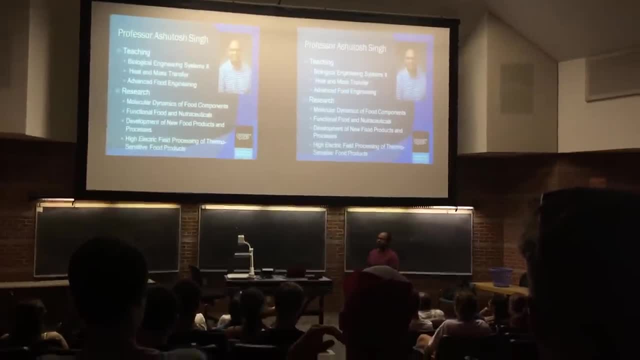 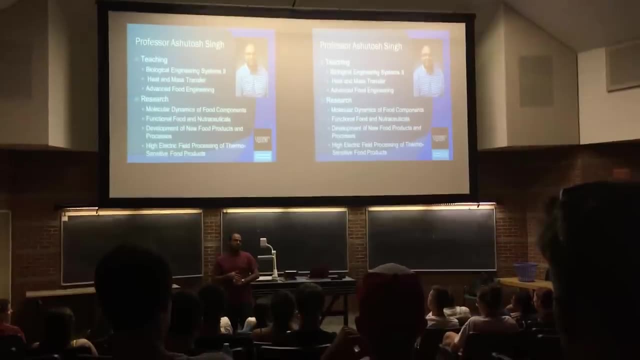 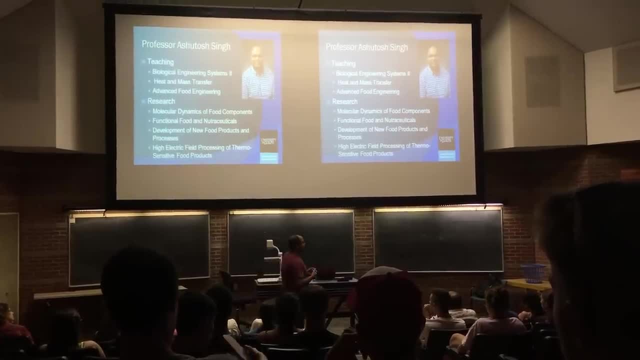 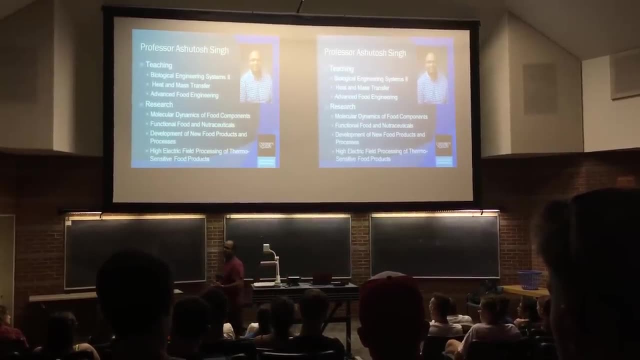 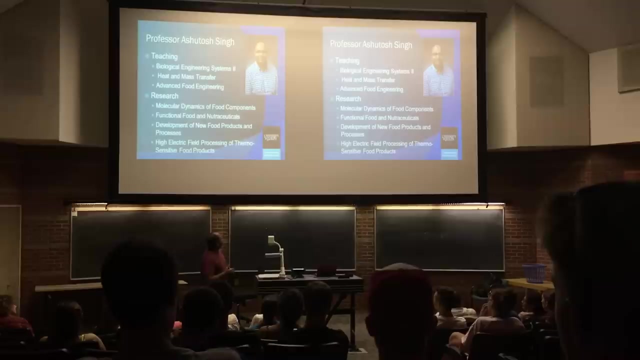 for you, for you, for you. I also designed new processes or modified processes to be applied in different other applications of food, And one of my expertise is with respect to high field processing. When I say high field, I'm talking about 30 to 60,000 volts. 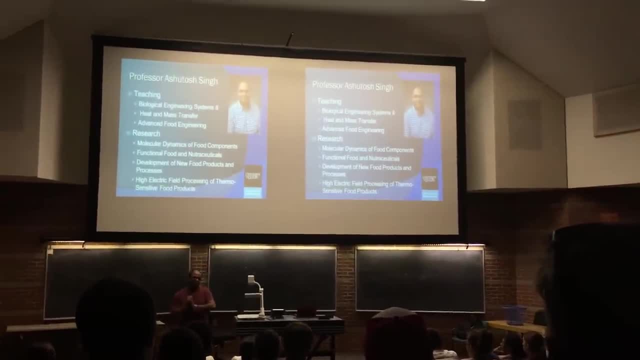 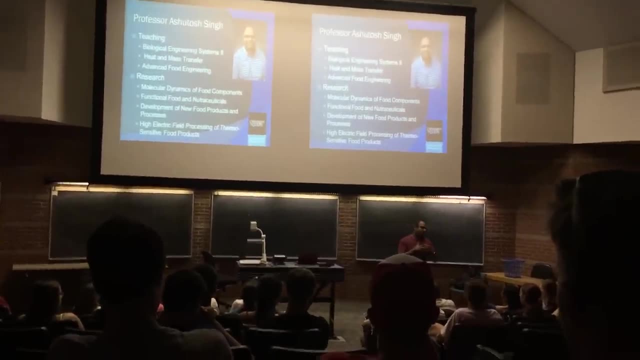 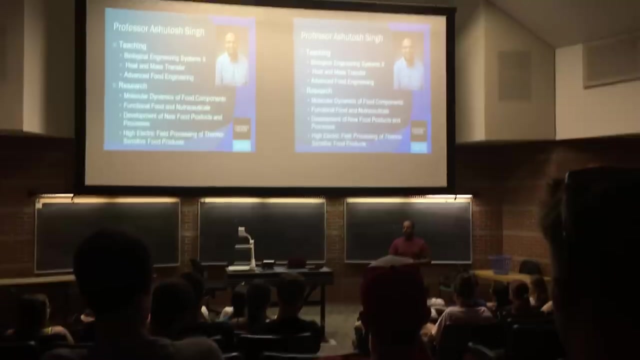 You don't have really better future equipment and you will remember it for a long time. But we use that voltage to develop a non-certain food processing system. So without heat you can process the food, kill the bacteria and food is good enough to eat. 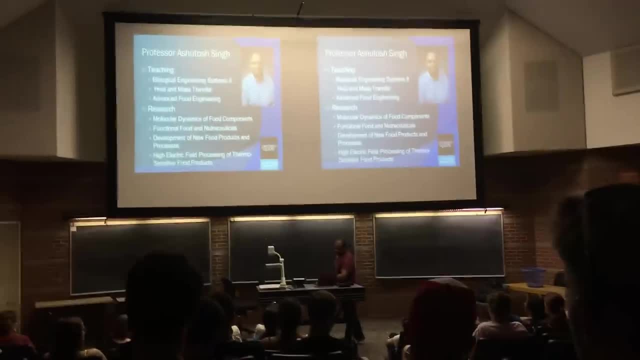 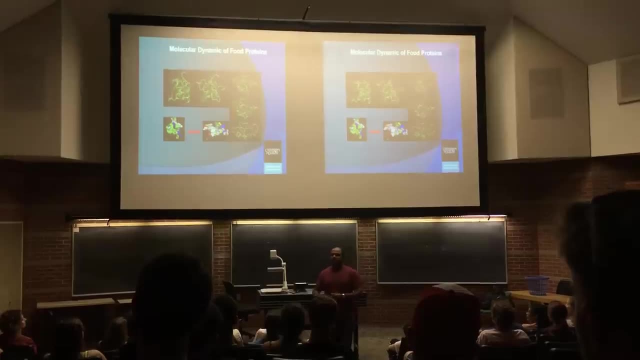 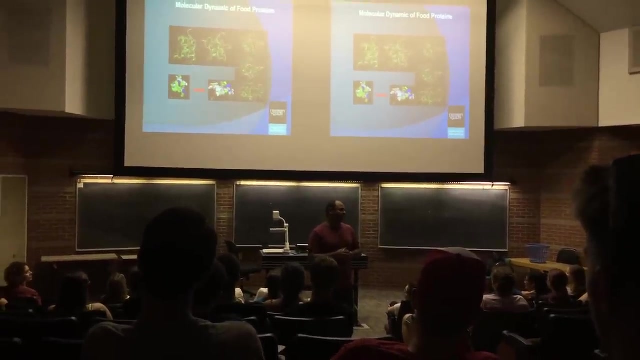 So those are the type of research which we do And that's molecule modeling of a protein. so I just wanted to show you a diagram of that So you will see, on the very left on the top, that's the structure, the 3D structure of a protein. 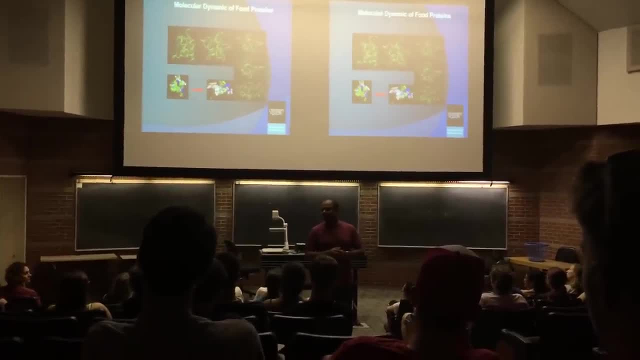 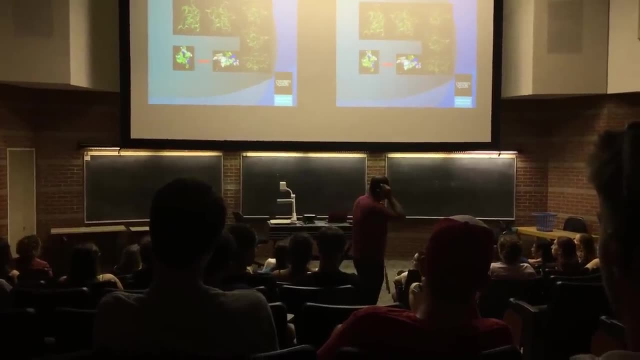 Do you know about the 3D structure of a protein? If I'm mistaken, that's a tertiary structure of a protein And that is under a microbe. So you see how the protein denatured or it opens up, right. 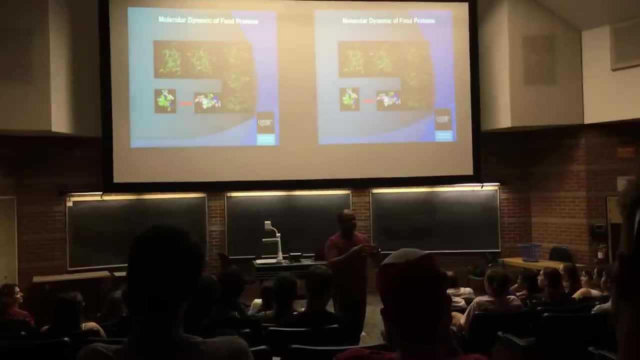 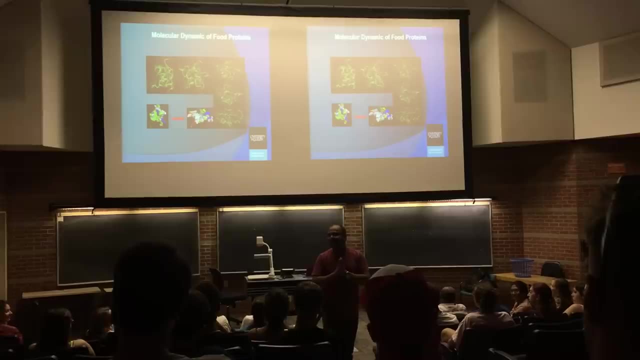 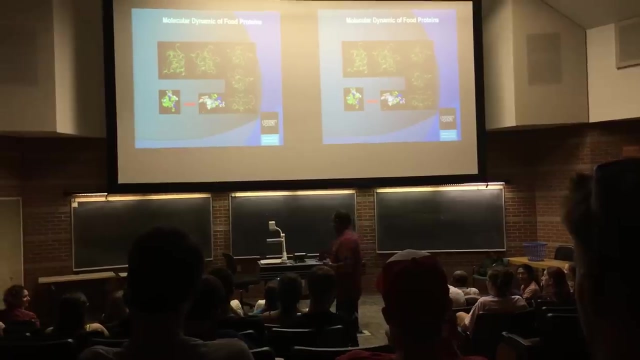 But you cannot see that being good or mean growth inside your microbe. Can you see it happening? Can you see the protein opening up? You can't. How do you visualize it? That's where we brought in molecule modeling. Molecule modeling is a tool to do this. 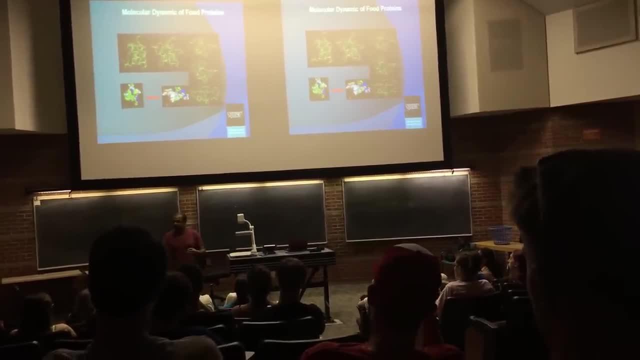 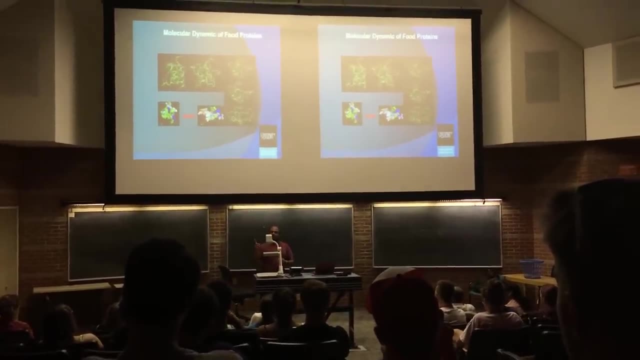 And it also gives us a lot of information from the monitor atomic point of view, so we can design the processes in such a way to get what we want. That's why I said biological engineering can do anything, Because, whatever we do, if your mom asks you to do something, you do it right. 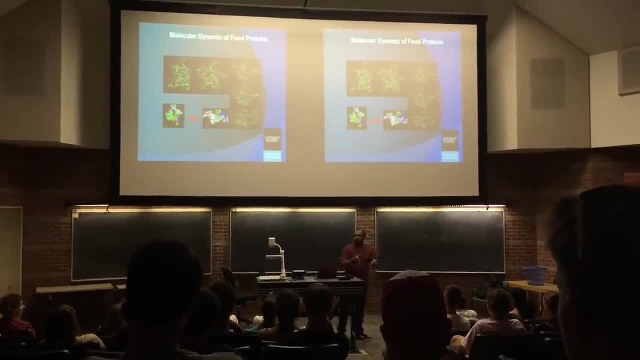 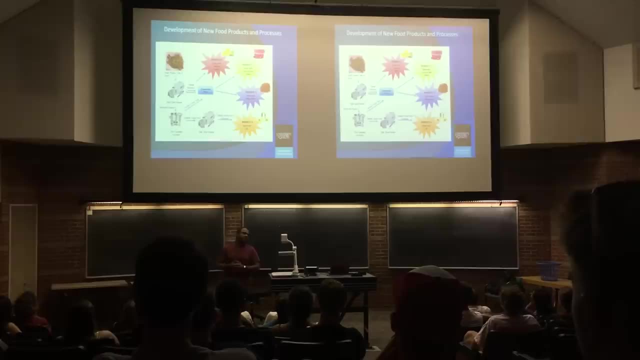 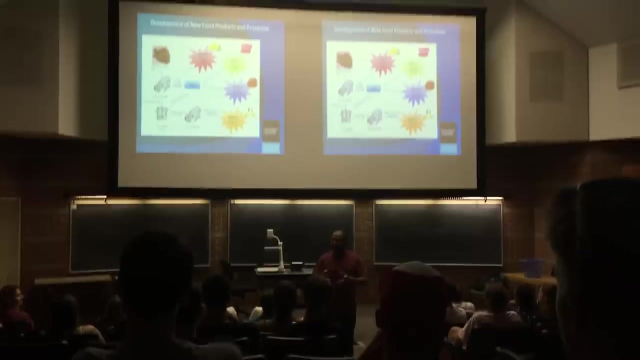 Biological engineering can do anything. Biological engineering gets at you Then new product development. What you see in the hands is a great bonus, After the white wine. how do we produce the white wine? We cut the grapes, we squeeze, we take out the juice, right. 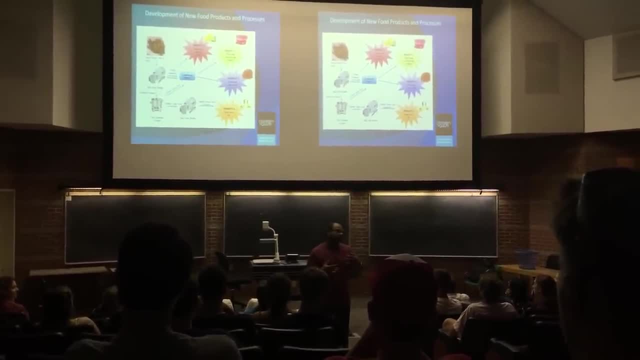 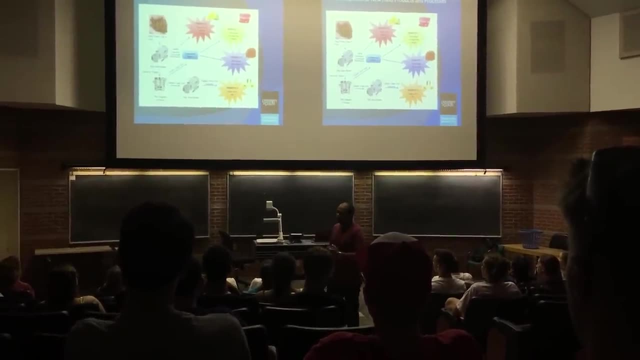 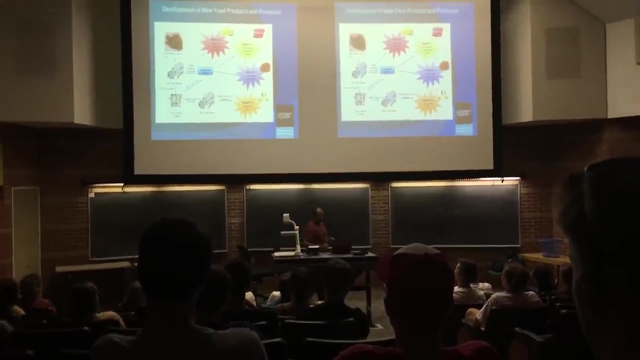 Whatever is left is a waste. That's why I said biological engineering also works for the environment. This waste is converted into new food products. We extract anti-oxidant products And we use 45% later on, So different methodologies we can use to do so. 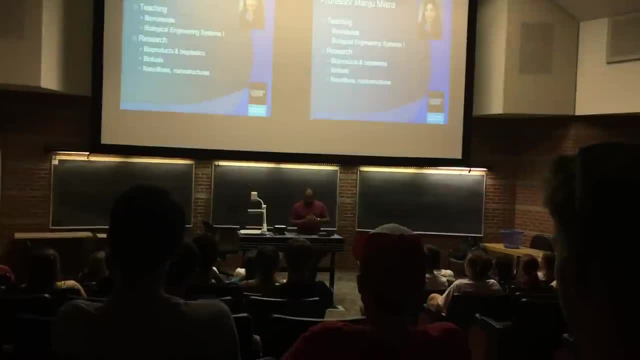 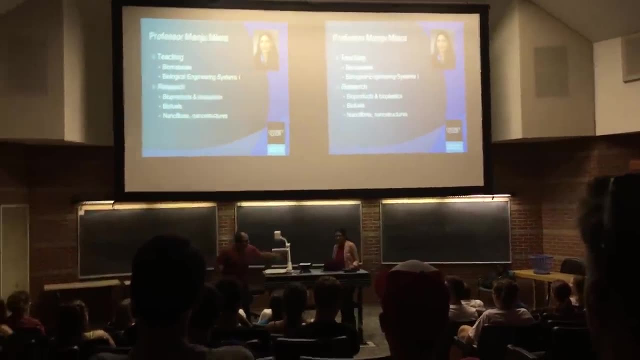 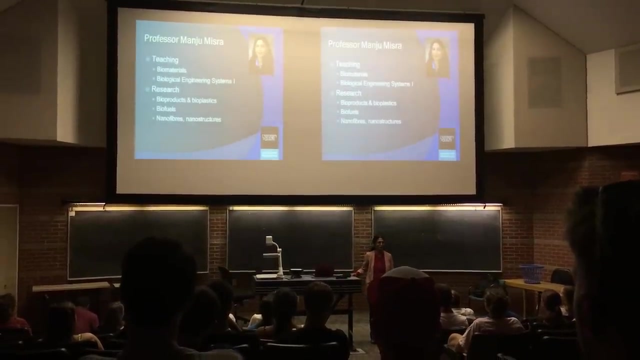 So those are the things which I do, And then I will let Dr Manjushree say a few words. Thank you, Okay. good morning everyone. You can see my name, Manju Mishra, And you can call me Manju. 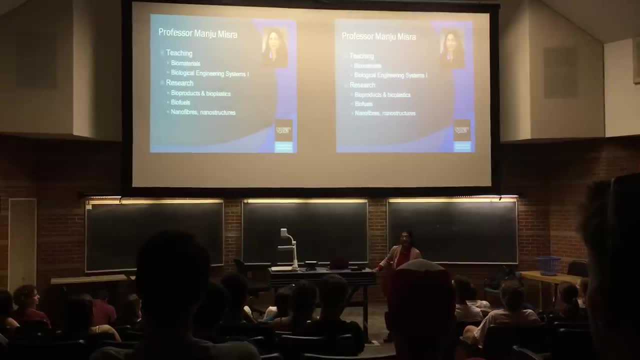 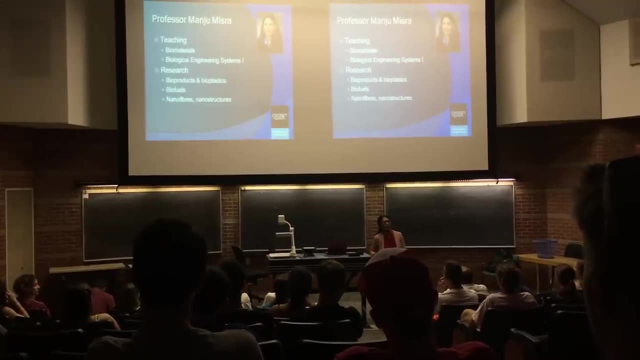 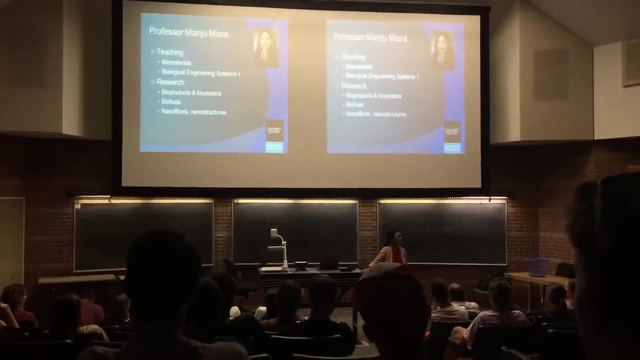 And, as you can see, I will be teaching in your fifth year The course that Professor Mithirajan told you about Biosystem 1., Which is Biological Engineering System 1. And which will be dealing with your application of engineering principles to the biological system. 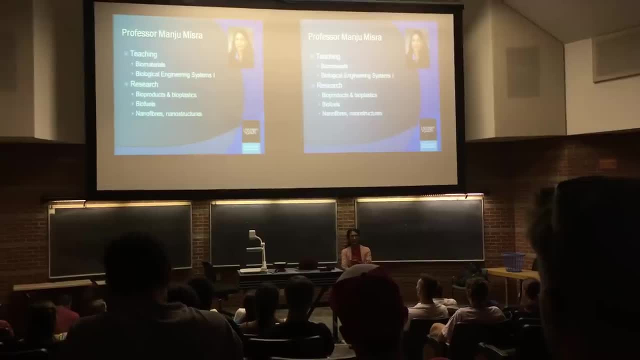 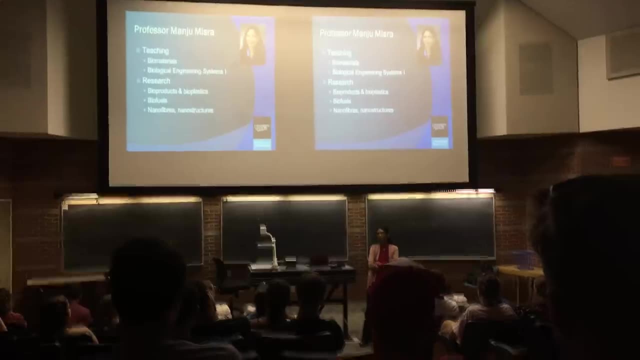 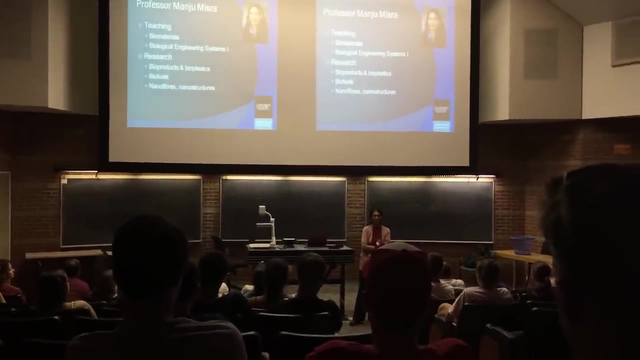 And that can go to various applications in industries like food, in medicine, in manufacturing. It can go to different applications And some of the examples, as you know, that you use, like food grade alcohol, Which is for wine, for beer and the several kind of that. 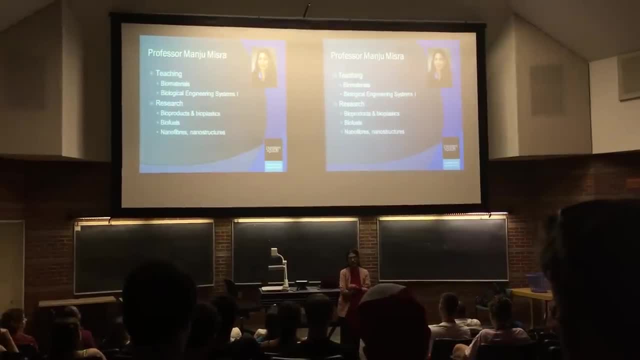 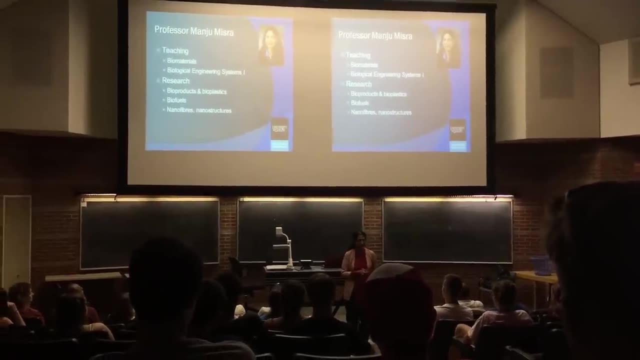 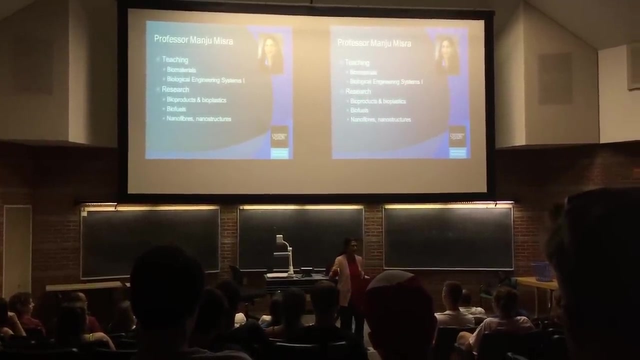 Or you can have the alcohol which is the industry grade. That means you use it for other purposes, along with in your vehicle. So if you go to certain like end of Husky, If you have filled your gasoline tank in Husky, You can see that this is always with 10% gasoline. 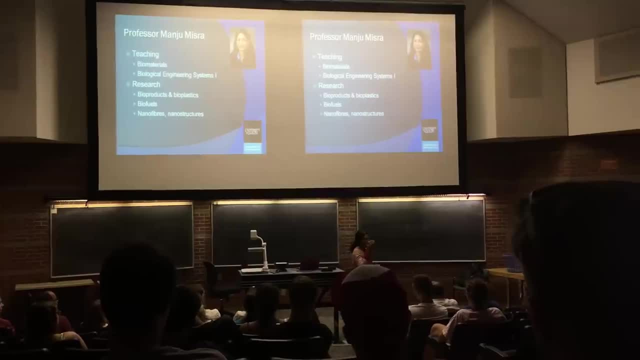 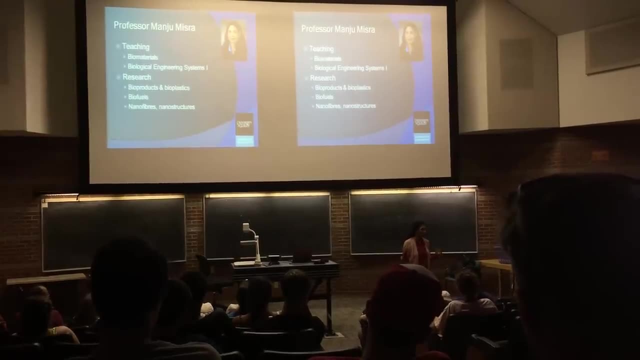 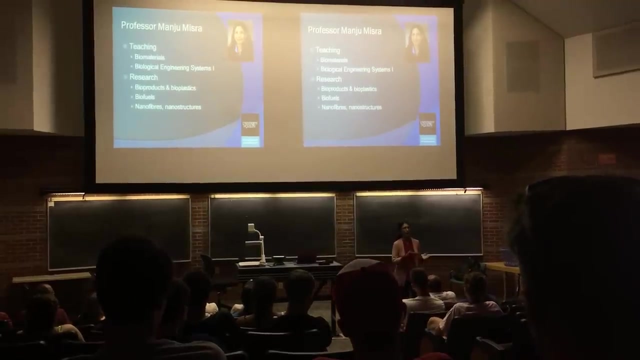 As a green symbol is they are with 10% of your bio alcohol, And this whether it is bio alcohol for food grade or for the, your petroleum grade. All these are obtained through the process from the your sugar fermentation From the natural sugar. 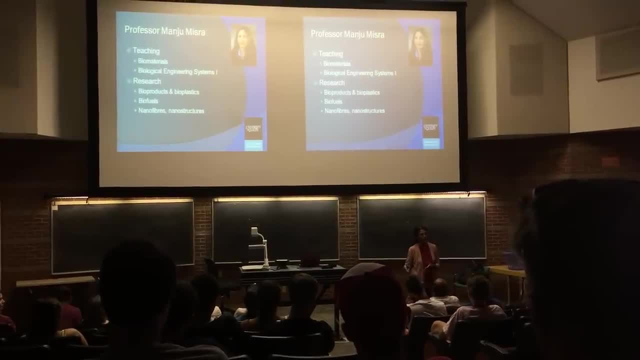 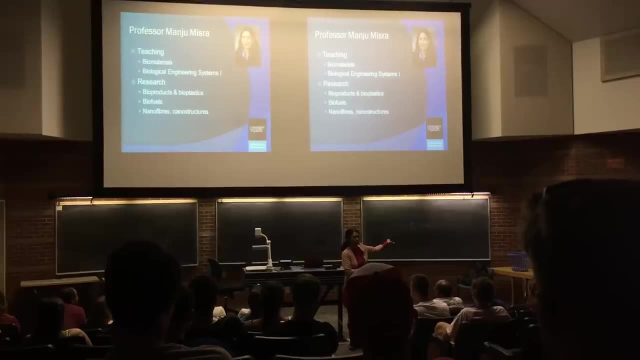 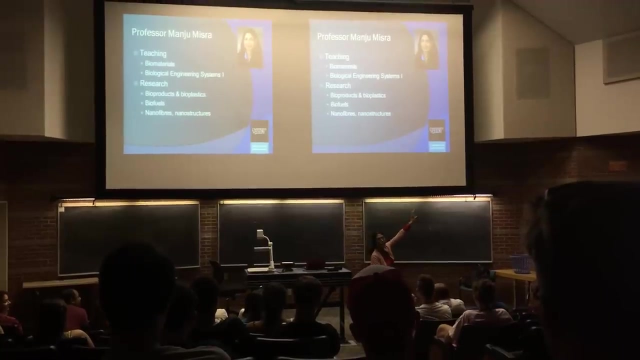 Through the process of addition of enzymes as well as Addition of The fermentation goes through in different industries. One of the industries is here: the slim and brewery. How many of you knew? slim and Slim and okay, So these are like they convert that from barley to beer. 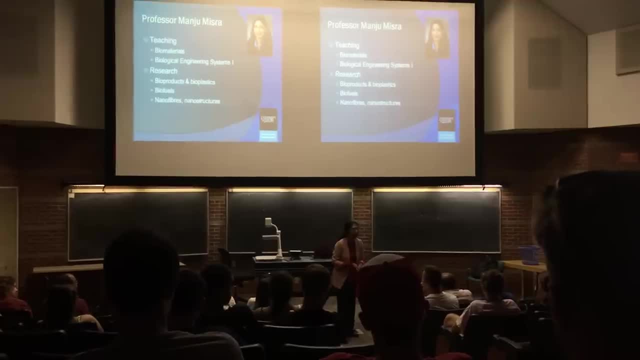 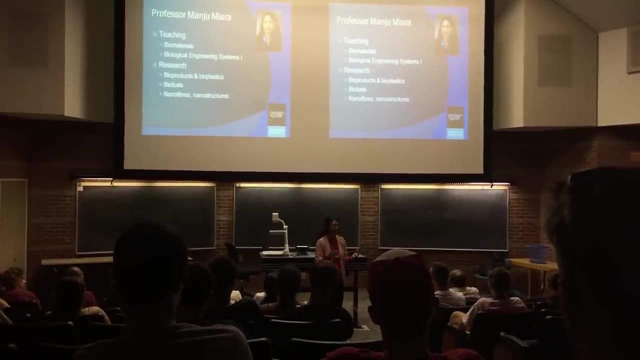 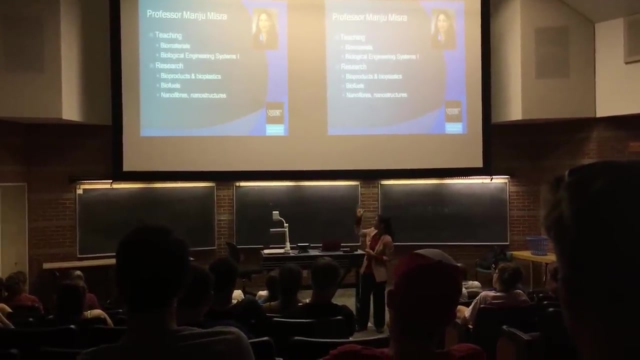 So, similarly, many of the students from this class are already engaged in different brewery In different parts of Ontario and throughout the Canada and other places- Some of your seniors. So that is what like. That is the biological system one. So I will meet with you. 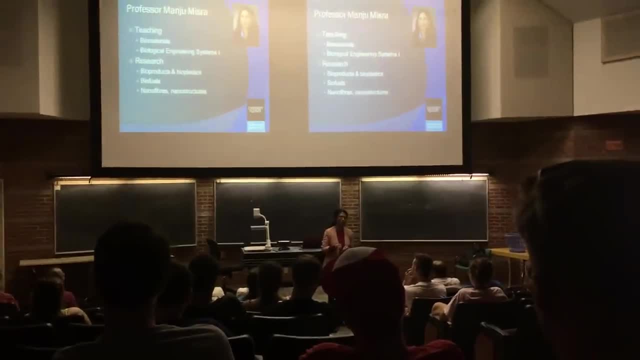 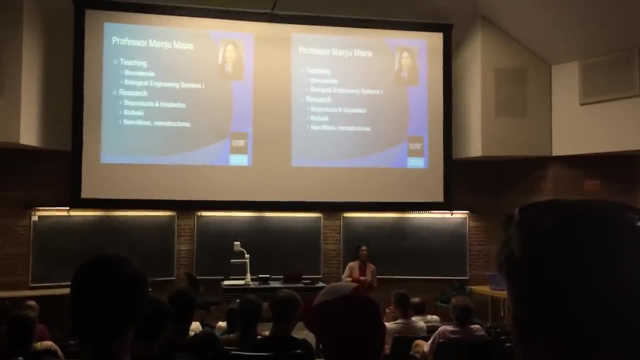 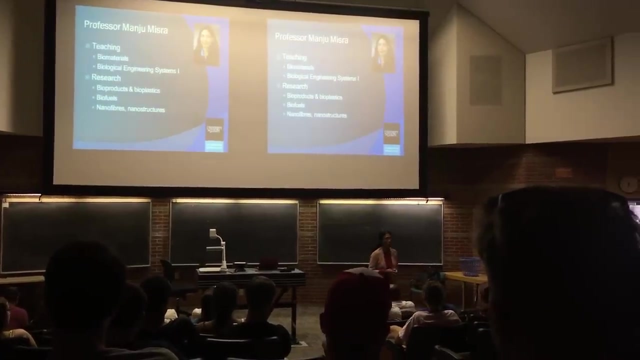 Registered for the course Next year in winter And besides that, I teach the bio material course in the graduate level, Where it deals with different biological processes along with manufacturing, Starting from packaging to Automated parts, as well as electronic goods, Depending on the nature of the 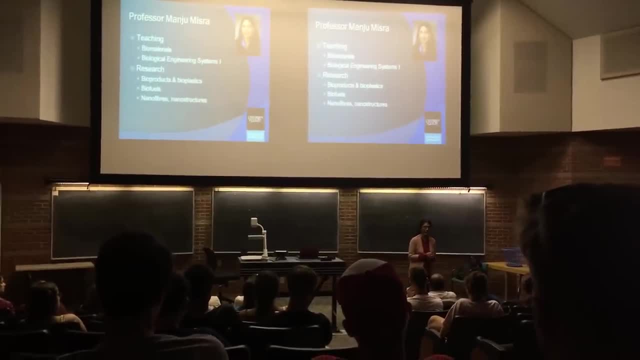 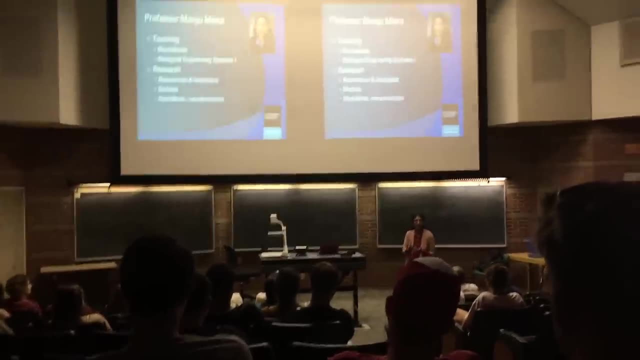 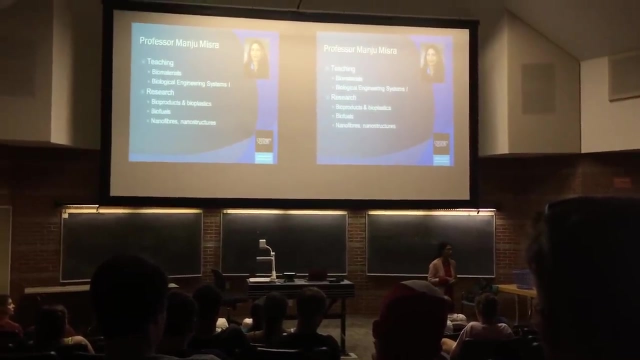 Your application or the funding agency. And coming to my research, I do with bio products, Which is the kind of general term, Or bio refinery. So how many of you knew What is GHG? GHG, GH as in go. 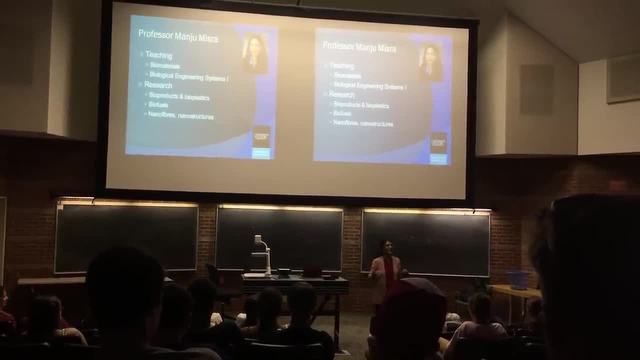 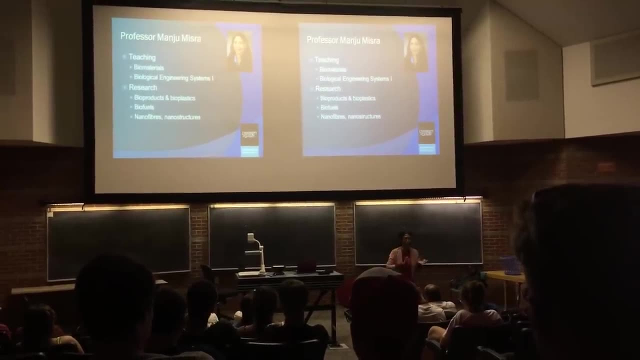 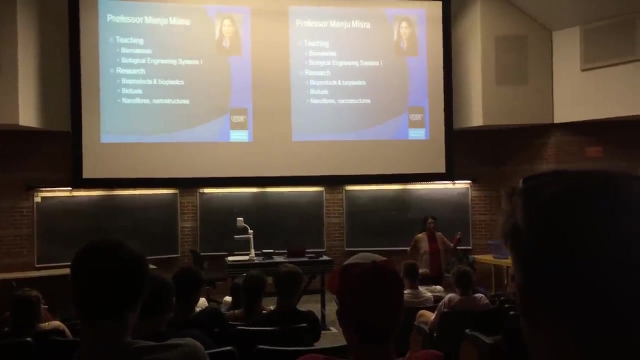 H as in horse And G as in go Is greenhouse gas. Okay, You are dealing with greenhouse gas every time. That is why today, On the 7th of September, We are like so hot outside And the warm, And this is coming from global warming. So this greenhouse gas emission, Meaning emission of carbon dioxide, Sulfur dioxide, Ozone- All these are coming out of our energy production, As well as our production of Where from they are coming. We are producing energy, But every day. 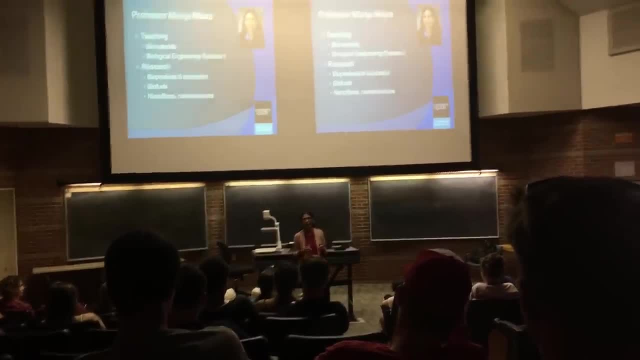 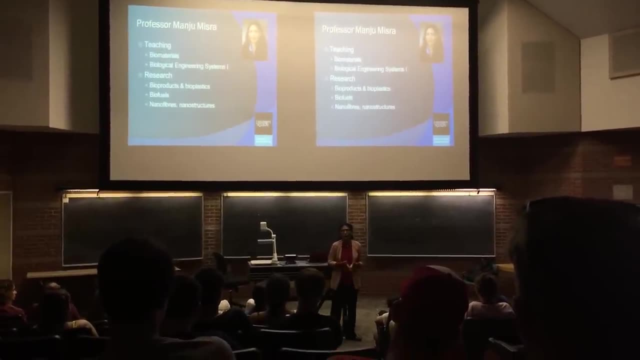 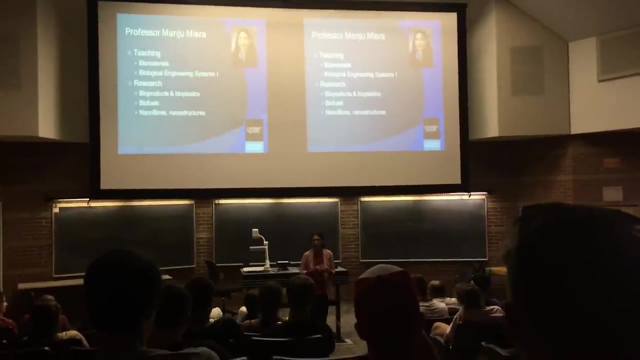 You get lot of greenhouse gas coming out In terms of carbon dioxide, Sulfur dioxide, from your vehicle, From burning of the gasoline, Burning of diesel. So all these things Are becoming really concerned Throughout the world And my research is dealing with. 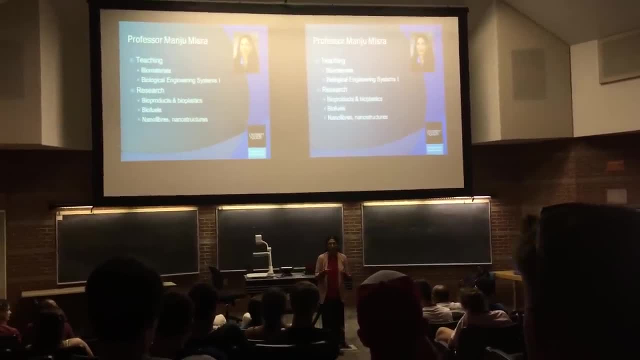 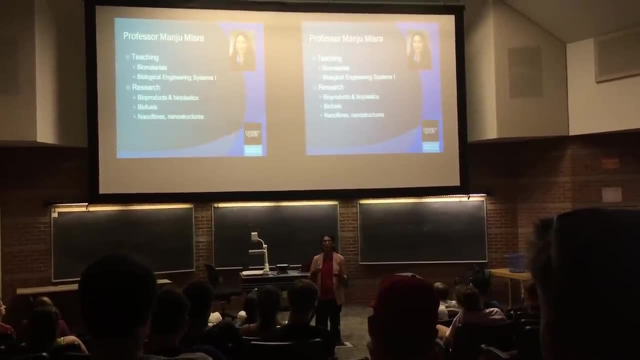 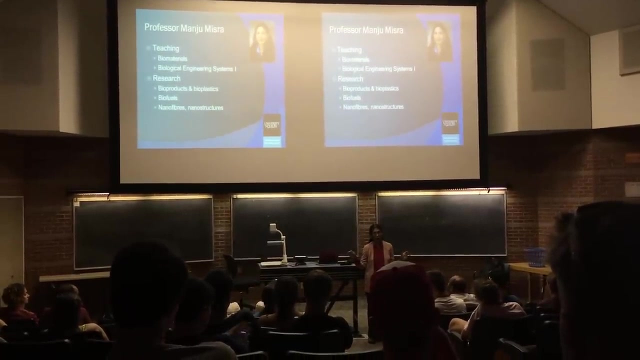 How we can take little step To reduce the emission of greenhouse gases, To reduce The impact of global warming, As well as to reduce The uses of petroleum. So with This, one is coming under a concept Called circular economy, Where the circular economy 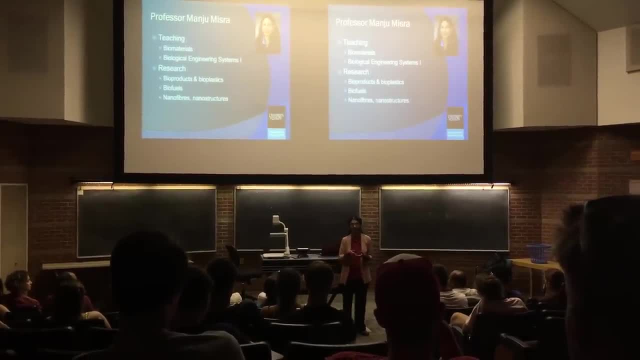 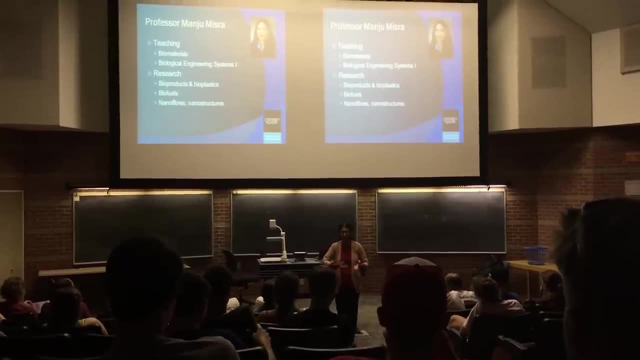 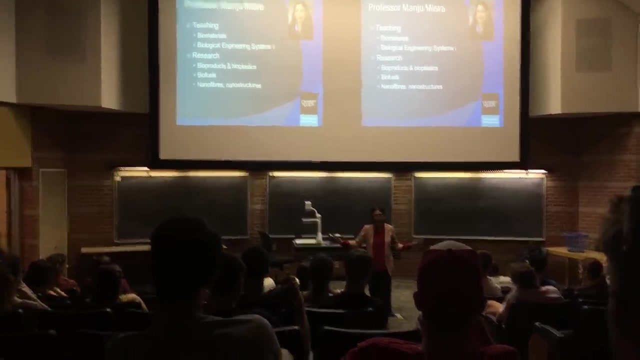 Is dealing with. You have to reduce And reuse Remanufacture. So that is the basic. So you cannot take, Make something, Make a bag Or make a bottle And use it and throw. That is called your linear economy. 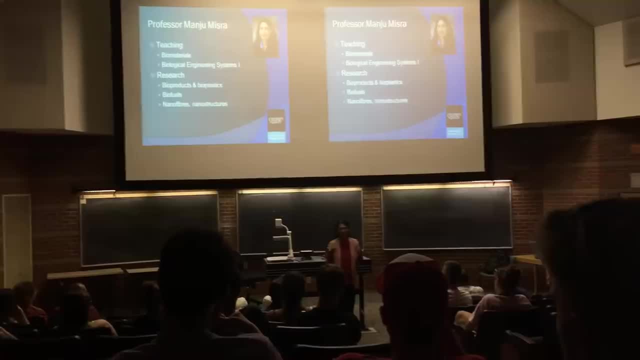 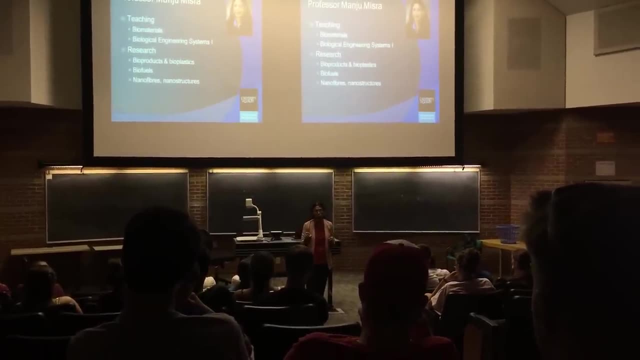 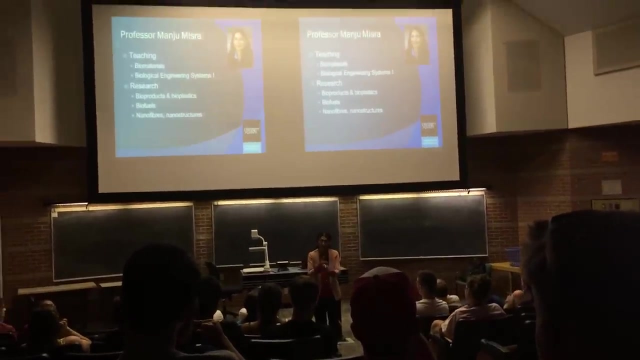 So, as you Pass out from the Your school And you get out for the jobs, You will be dealing with the circular economy, That is, the closed loop, Meaning no waste From the basic, From the starting, from manufacturing, design And with intention. 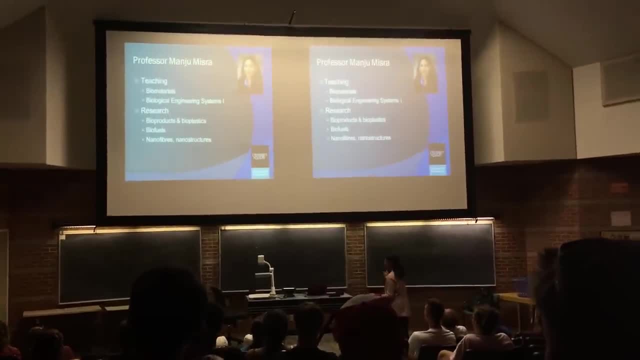 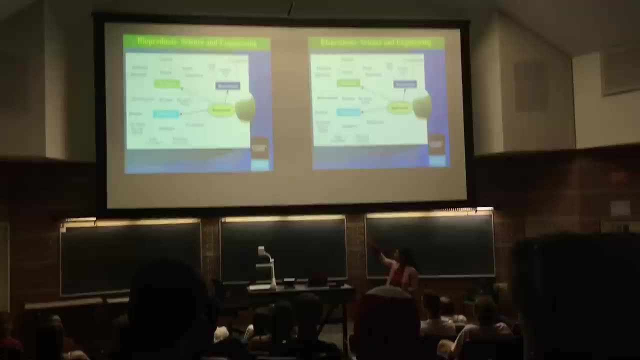 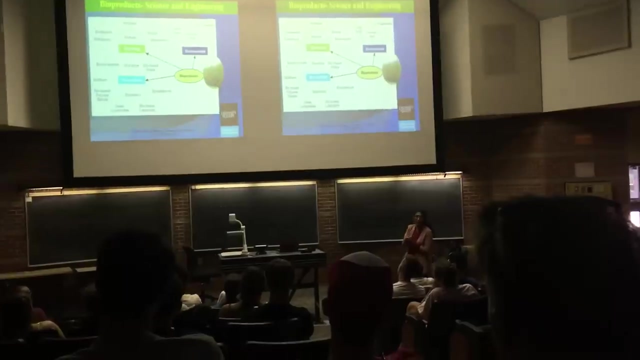 You have to build the system So there will be no waste In the system. So, as you can see Here, The bioproducts, as you can see, Are obtained from any renewable resources And that can be like your. The first one is biochemical. 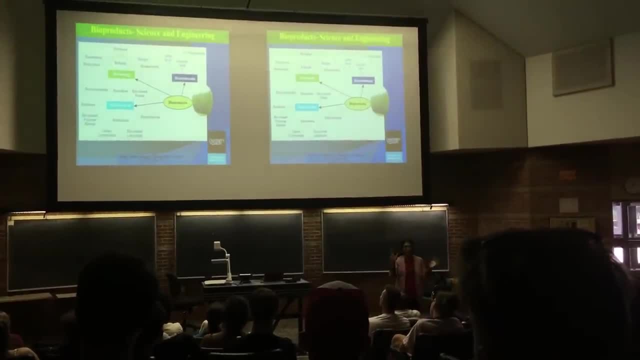 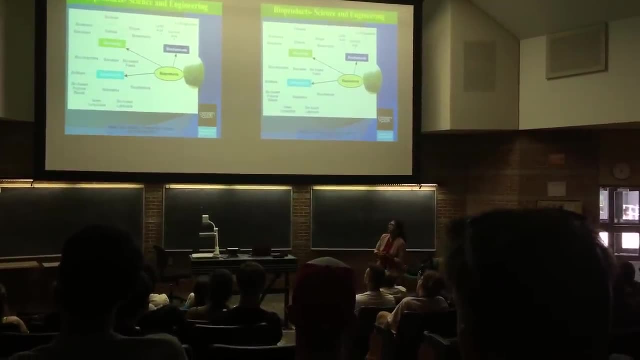 It could be lactic acid, It could be succinic acid Or similar chemical That you can also get from the petroleum industry. The second one On the top left hand side: It could be any kind of your energy Like fuel. 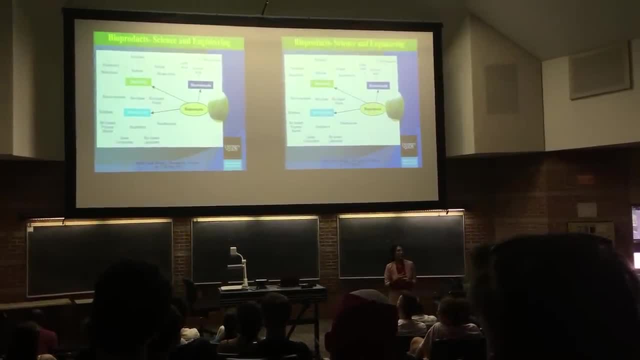 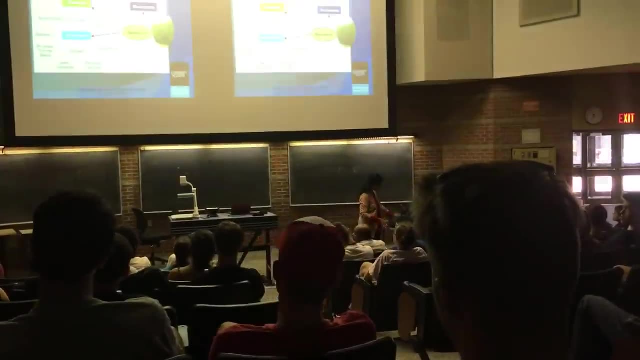 That can be bio, like alcohol, Or bio diesel, Or bio gas or bio electricity Or any kind of product Meaning whatever the salt or the dress Or this kind of carpet, All can be made from the non petroleum resources In that way, 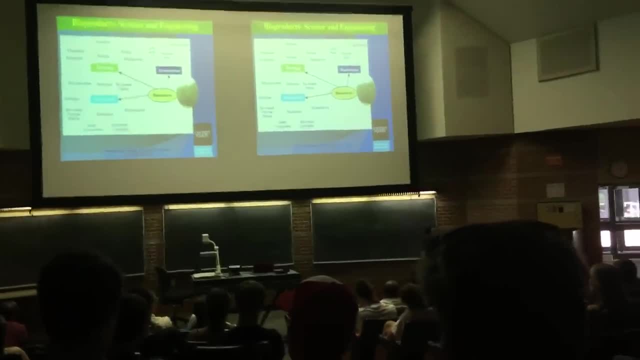 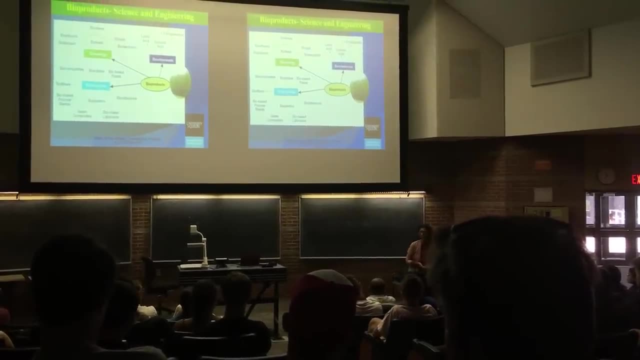 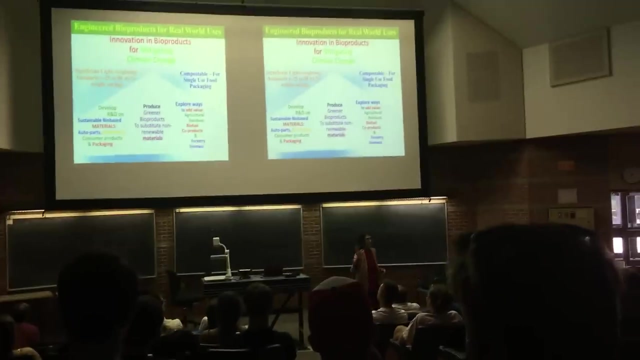 You can sustain the existing petroleum As well as You can have like less greenhouse gas emission And you can have a Really better and green product and society. So The last one, Last part one, of course. So this is my laboratory. 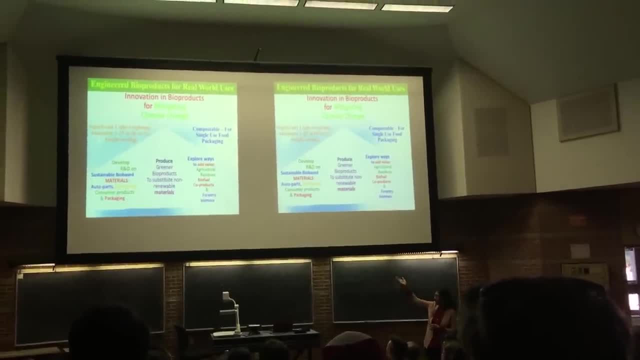 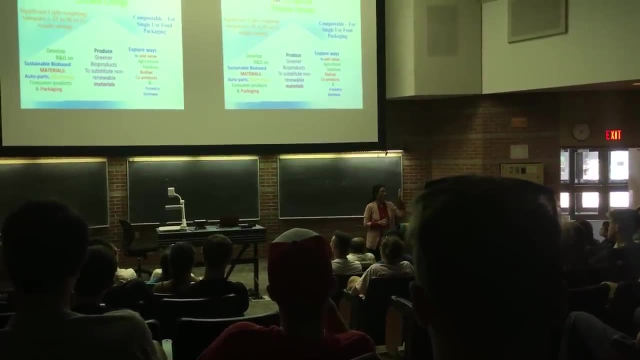 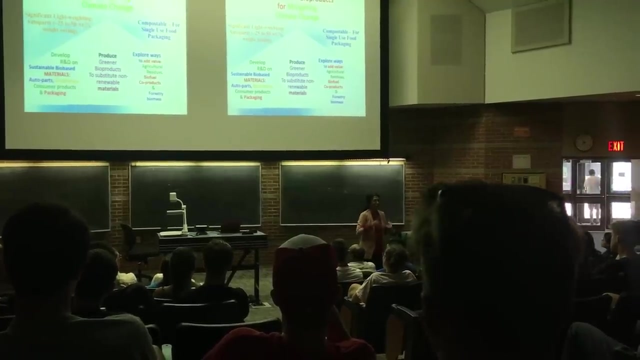 Where we deal with Your lightweight production. How many of you Knew the CAFE standard- Perforate average fuel economy standard That is called CAFE standard, Which means It is mandatory by 2025.. The car should go for. 54 miles per gallon Or it go 23. Like 23 kilometers per liter As per the Canadian standard, And for that You need to make the automatic lightweight. So for light weighting Can be done By different designs. 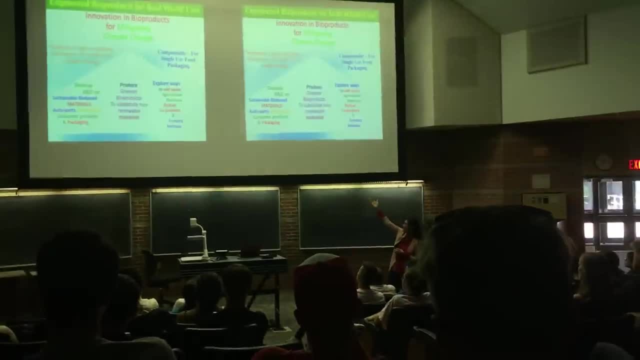 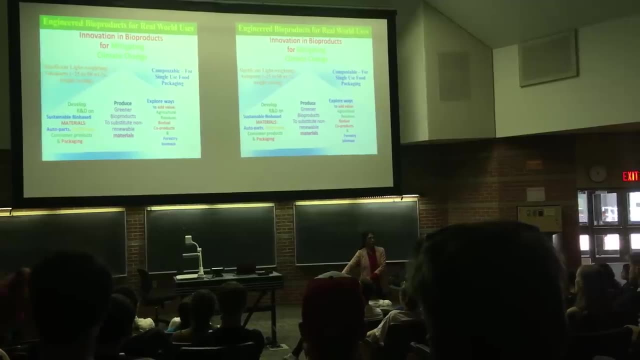 Using different new materials. That is what one of the research we do And the right hand side top one: You can use a compostable full packaging And use it And put it in the compost So this will kind of decompose. 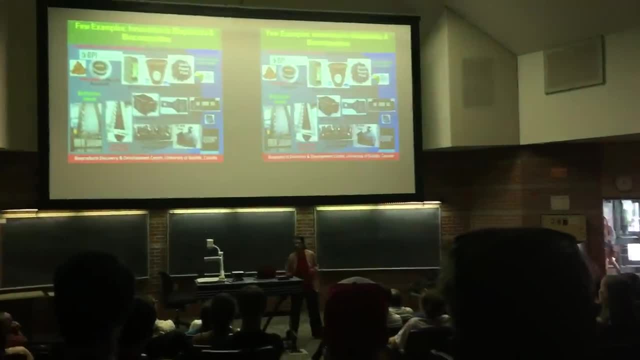 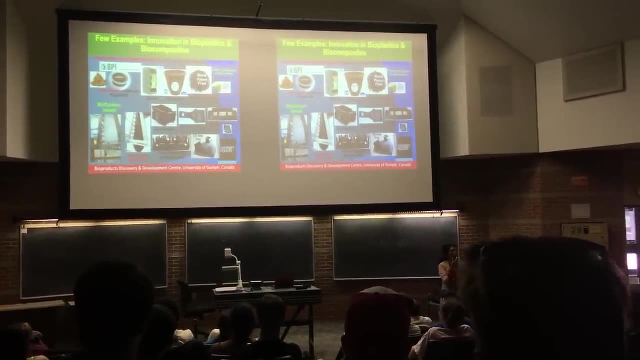 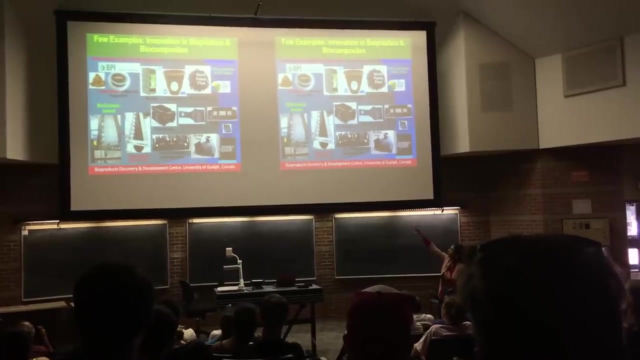 To carbon dioxide and so on. So here are some of the products From our research Which is obtained from the top one One time single use coffinning That is obtained from the Waste feed stock, As well as the beans And the flower pot. 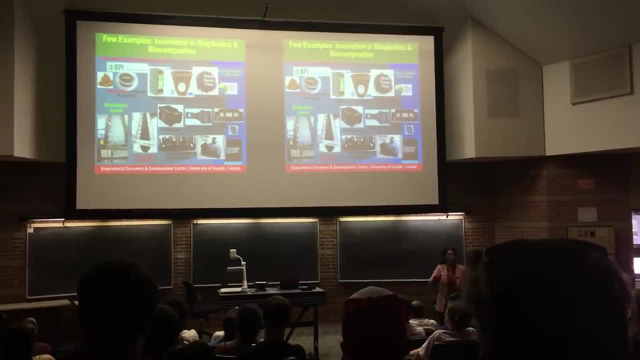 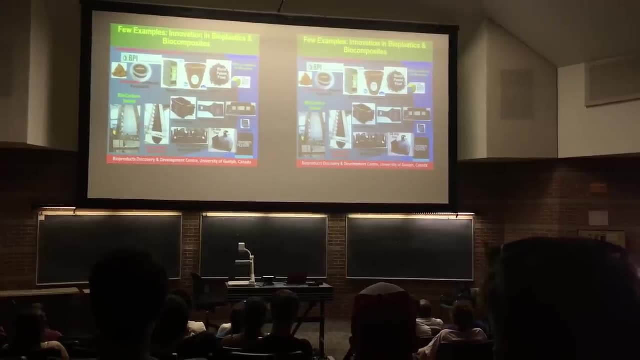 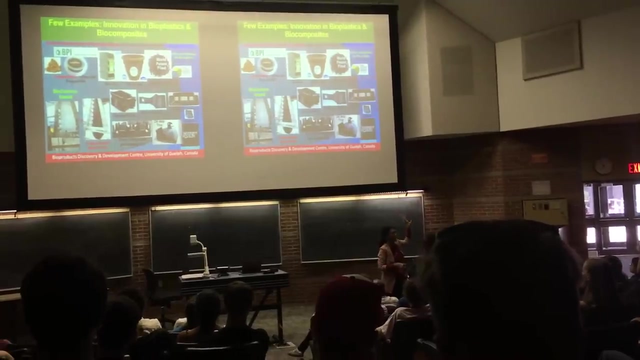 The left hand side is some of the Your film. That is for mulch filling, As well as the coca cola Bottle packaging tray And oil drip tray. All these different parts For different companies are going on And many of them are already in the market place. 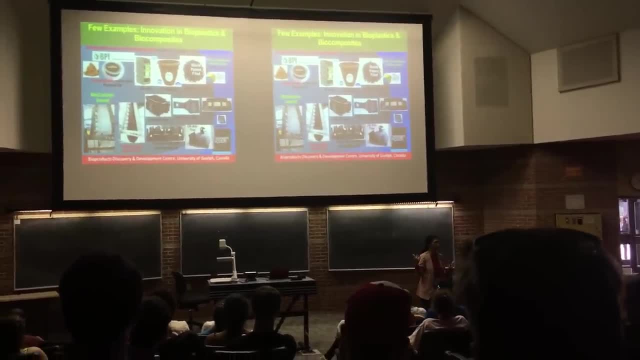 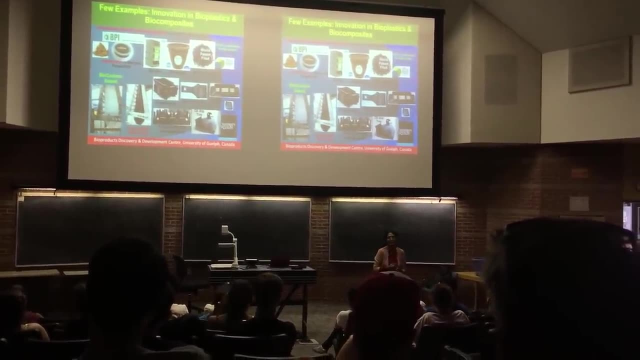 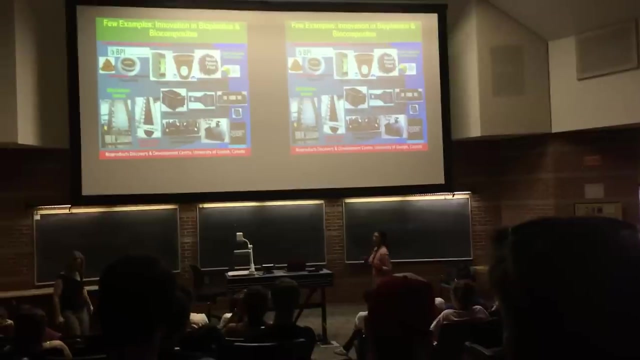 Whether you go to, You can find all these things In the fortune. So you all are welcome To contact And see in case you want to do research In the summer And come back as a graduate student. You all are welcome. 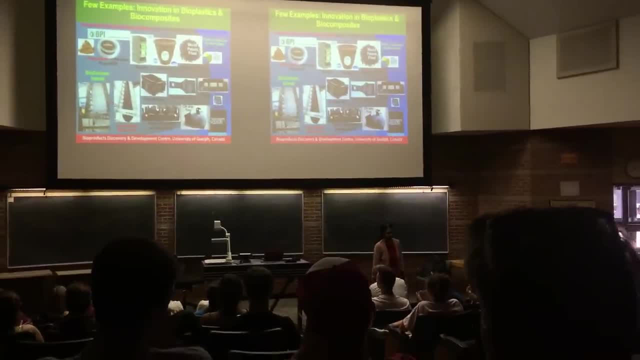 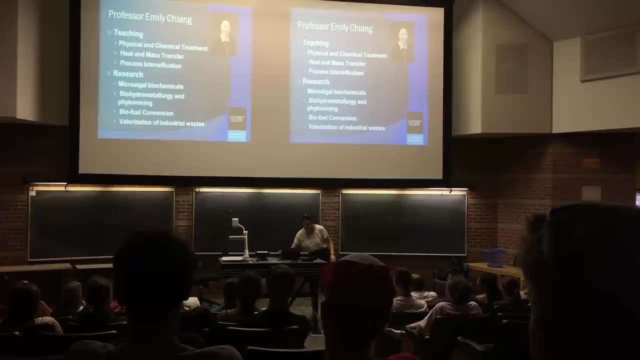 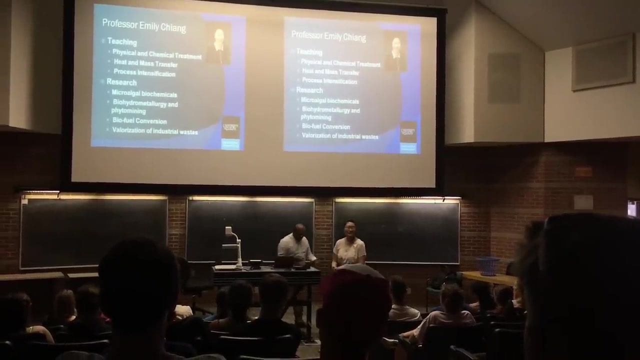 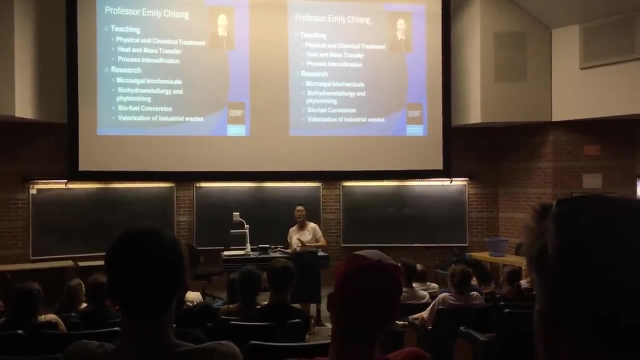 So now we welcome to all of you And thank you so much. Thank you, Hi. good morning everyone. My name is Emily Chen, So in terms of teaching, For me is a mix between biological program As well as environmental. So I will see all of you guys in your third year. 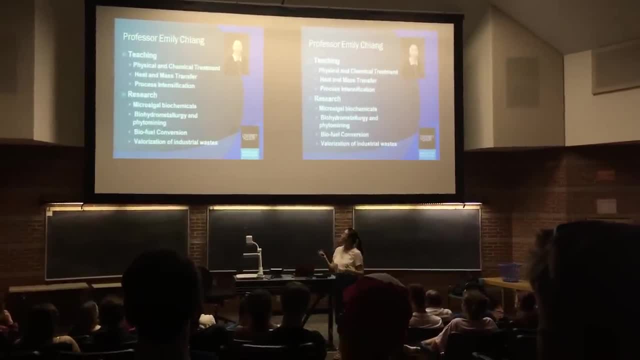 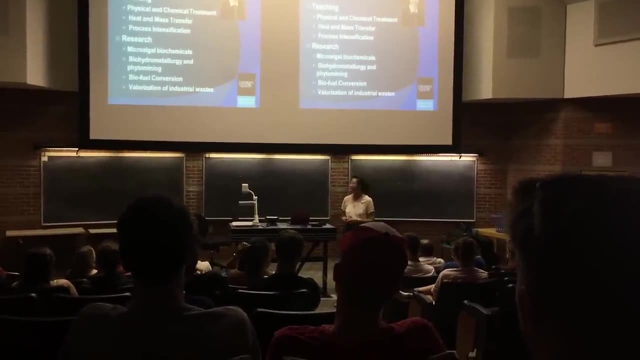 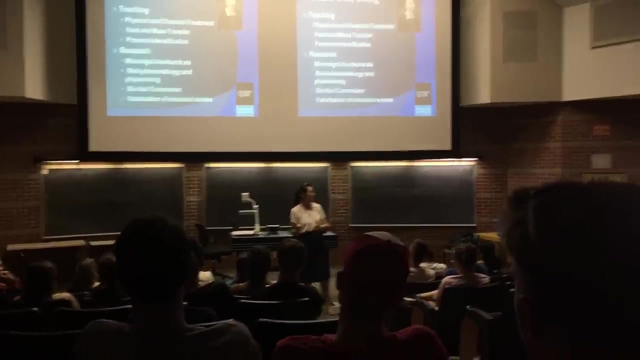 For heat and mulch transfer And I have a fourth year course For physical and chemical water And waste water treatment. That is an environmental course But if you are interested You can also pick it In the graduate level If you want to go on to your graduate study. 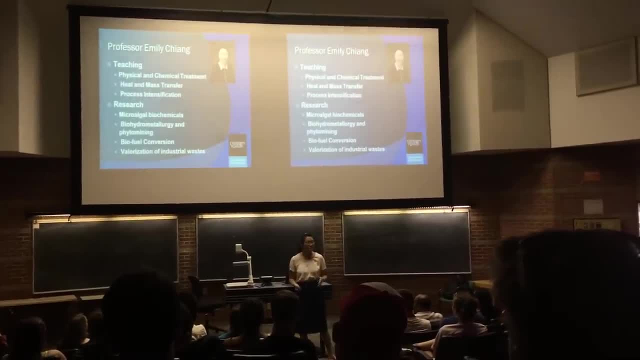 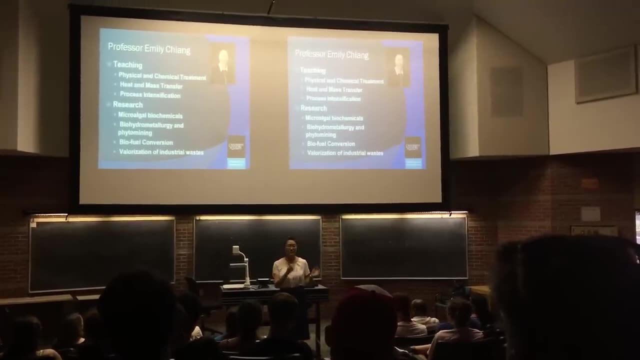 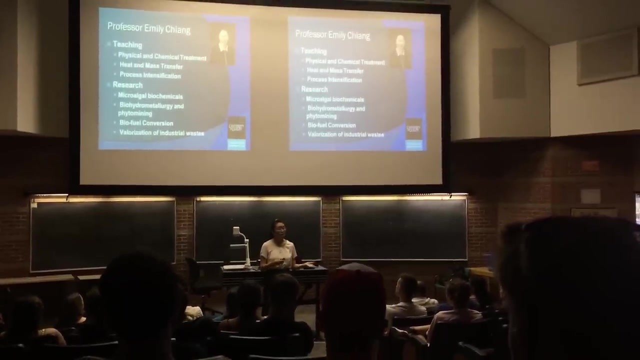 It is a course that you can consider. So, in terms of my research Is also a mixture between environmental And biological engineering. My research is based on Waste valorization, Which I turn industrial waste And convert them into useful product. I use it both biological. 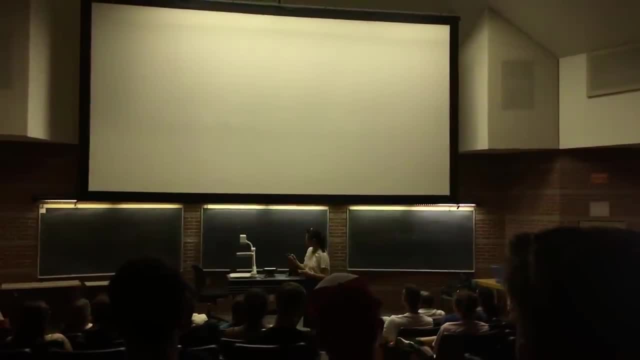 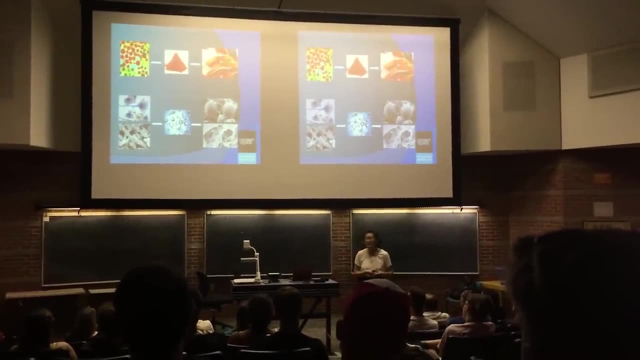 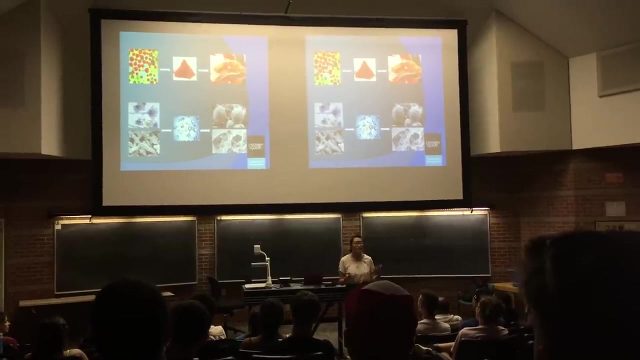 As well as chemical waste to do that, And here are just some examples Of the work that I am doing Here. on the top, I am using micro algae To extract astaxanthin, Which is a very good antioxidant For food and biological use purpose. 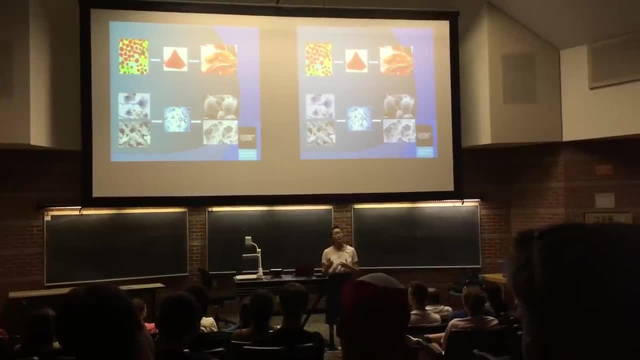 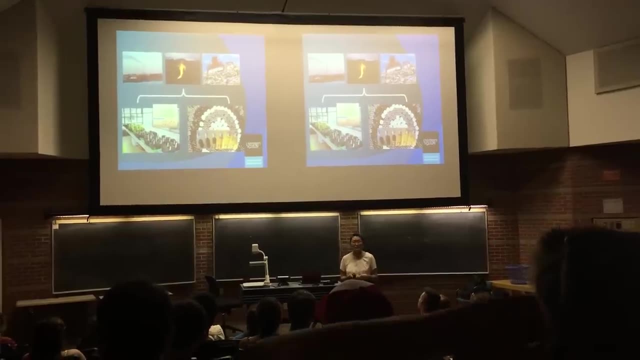 And also I am looking at different bacterias As well as fungi. To try to extract rare earth metals, Heavy metals, from industrial waste Here- because we have so many waste And right now There are natural resources- Is depleting from the world. 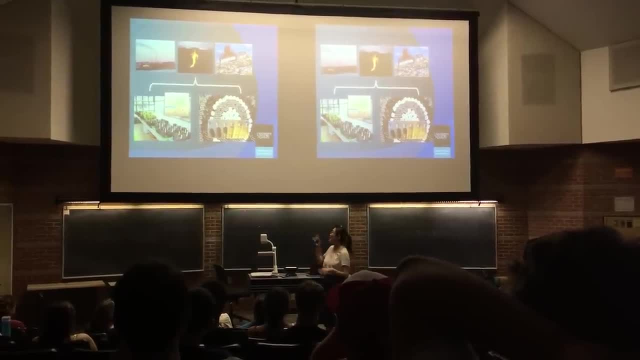 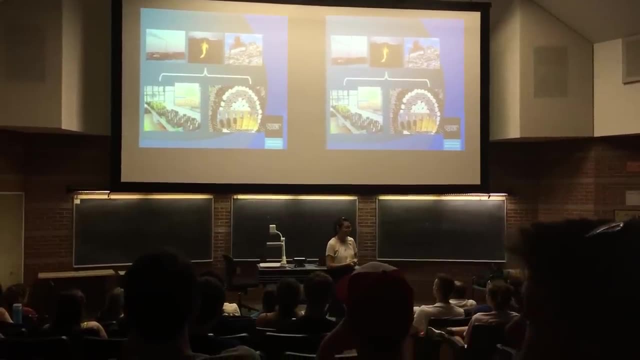 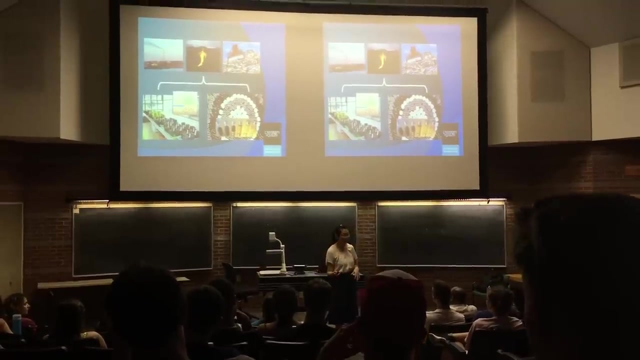 So what we want to do Is convert them into products, And these are different kind of ways We can do that, And the interesting one Is that we are looking at here Using plants to extract useful products From the waste. That way, we can eliminate waste. 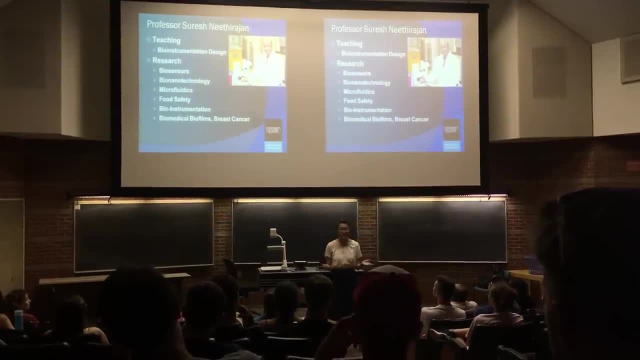 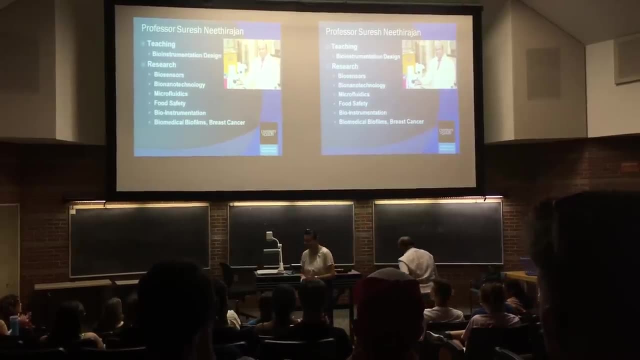 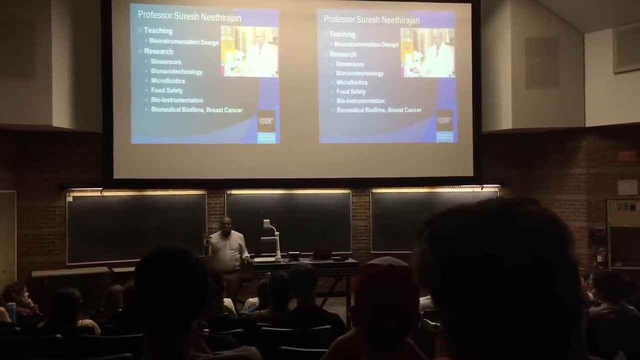 As well as eliminate the use of natural resources. So, basically, this is my research And I just want to say Welcome to the University of Guelph, Welcome to the School of Engineering And have fun, Thank you. So some of 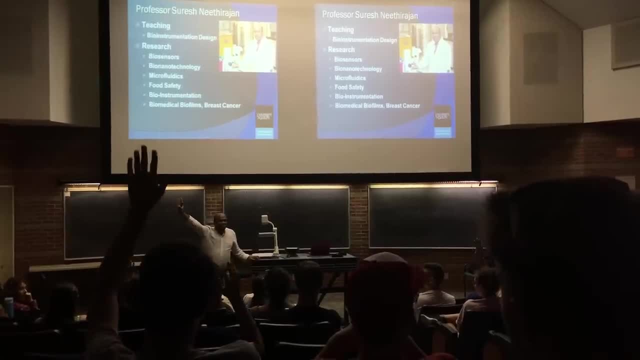 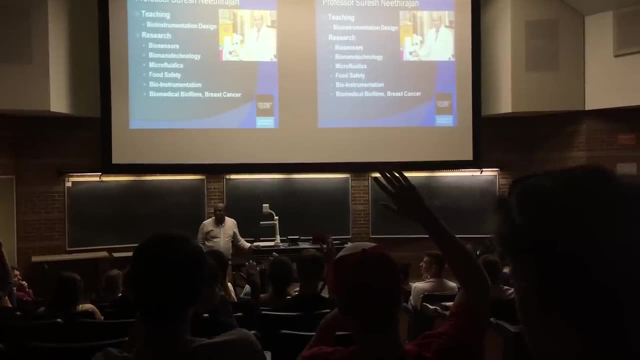 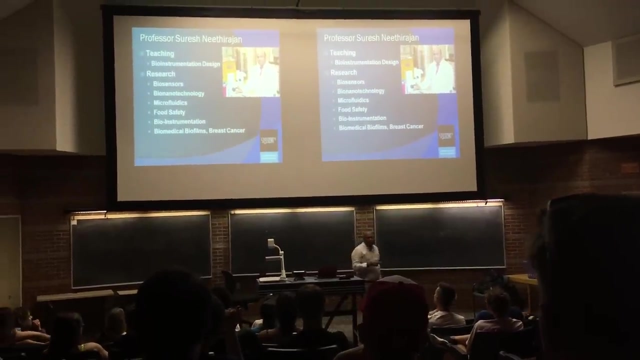 How many of you are in regular stream And co-op stream? Regular stream, Co-op stream: Majority And co-op stream? Three, Of course. So Professor Manjameshwar mentioned That she is one of the rich faculty. 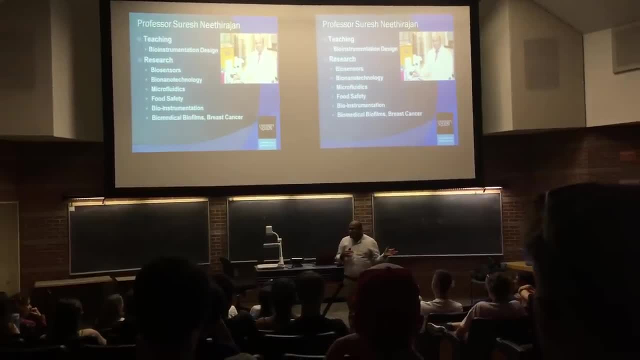 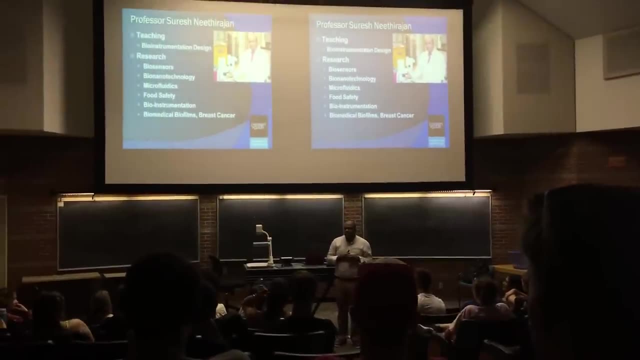 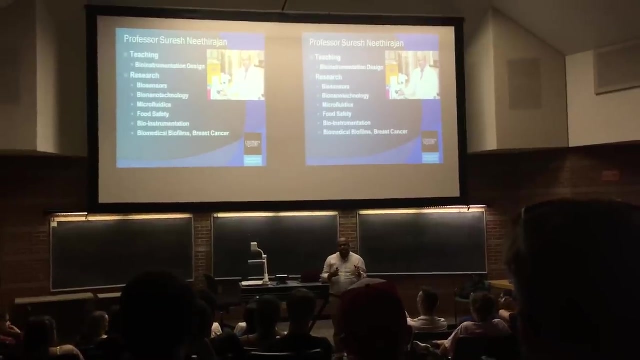 In terms of research funding. In addition to her, There are other faculty members And professors. They have the ability And also the Provide opportunity to hire you As a summer student Or a co-op student for a four month term. 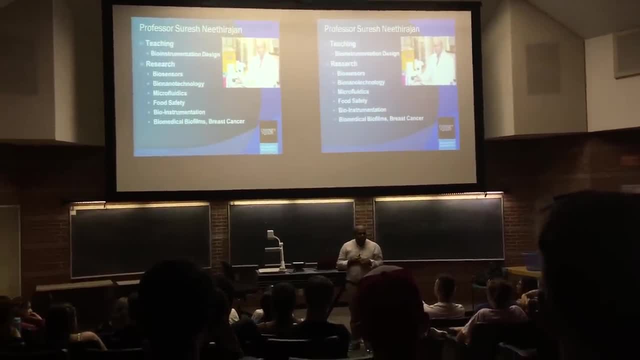 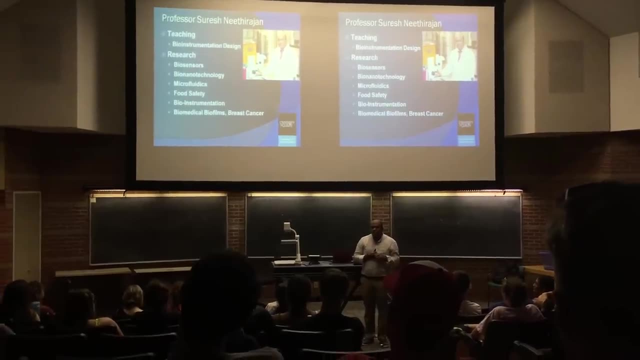 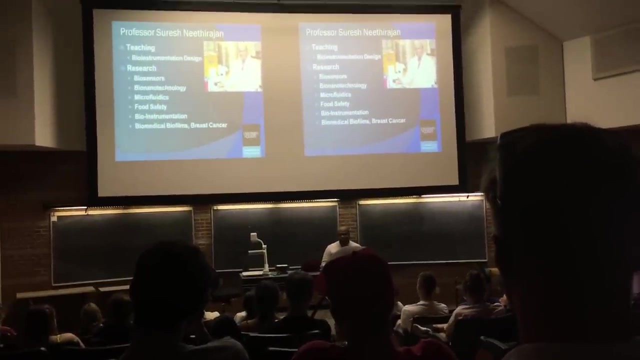 Or an eight month term, So it's a fully funded program. So it is Because the laboratory has state of the art Infrastructure and equipment You would be able to Deal with, Play with And develop novel solutions In the labs. 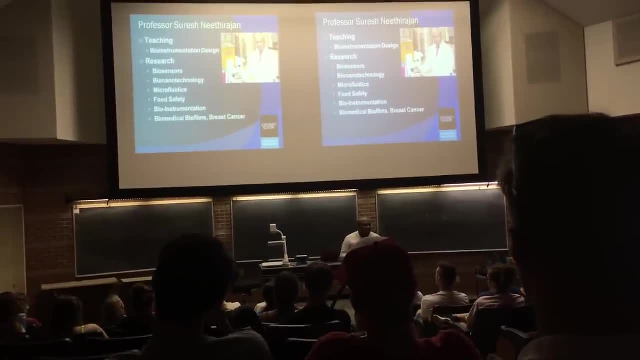 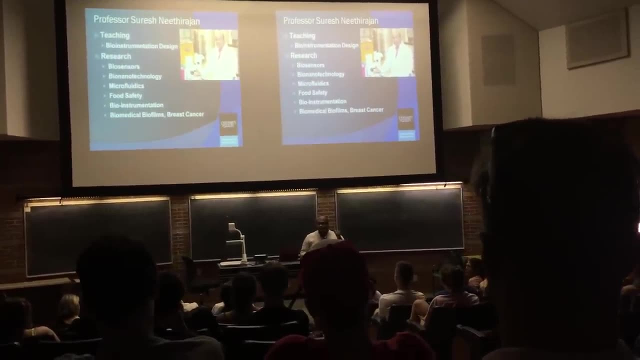 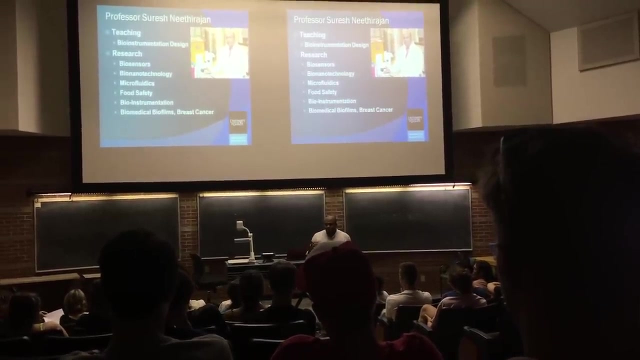 Within the professor's research laboratory. So feel free to Explore From day one onwards, Because if you are going to be a good researcher, You can be a good Employee in any industry. The process of research Is very intensive. The more you learn. 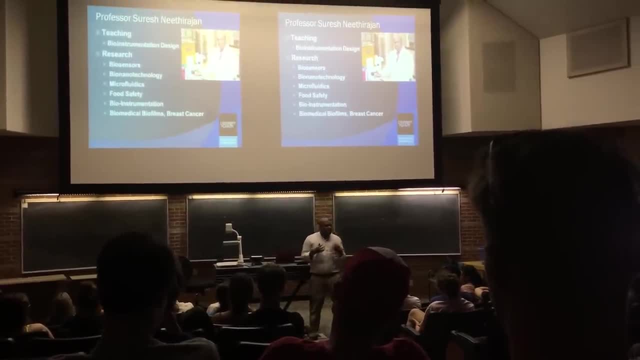 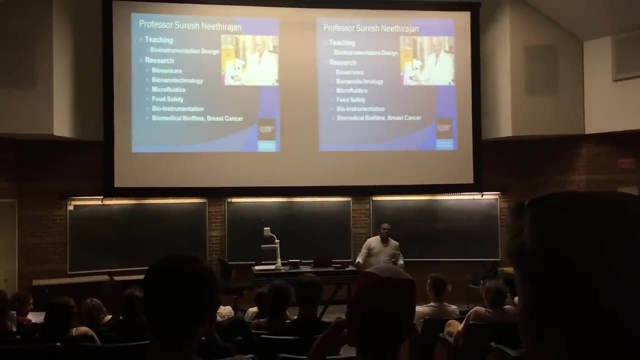 Different technical skillsets At different levels. You would become a better engineer As you grow. So my name is Suresh Nithirajan. again, You can call me Suresh or professor Suresh. I teach a. 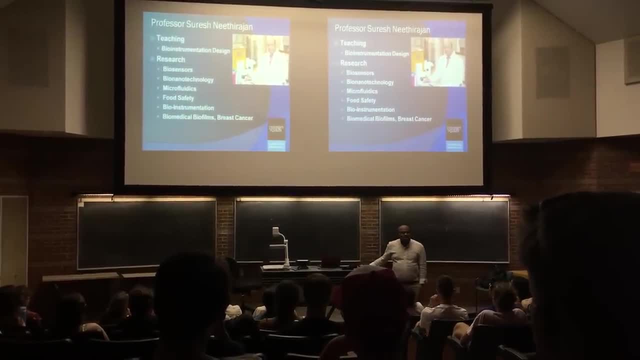 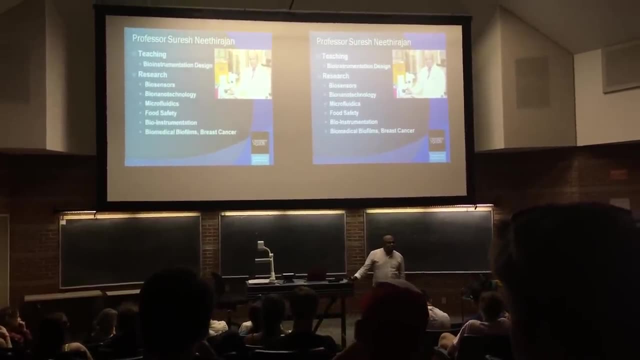 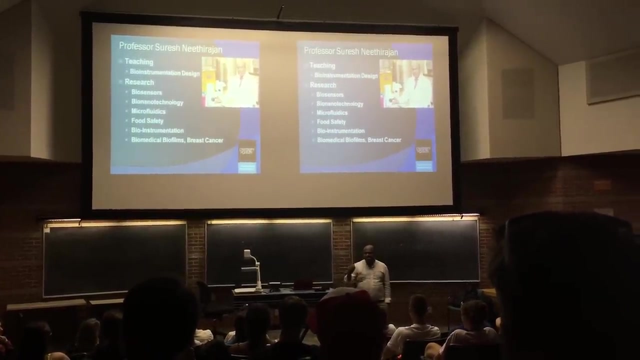 Fourth year course called Bio instrumentation design. It is one of the popular courses Within the biological And biomedical engineering program, Mainly because the students Get to play with lots of gadgets, Arduino- Many of you have used Arduino, So yes. 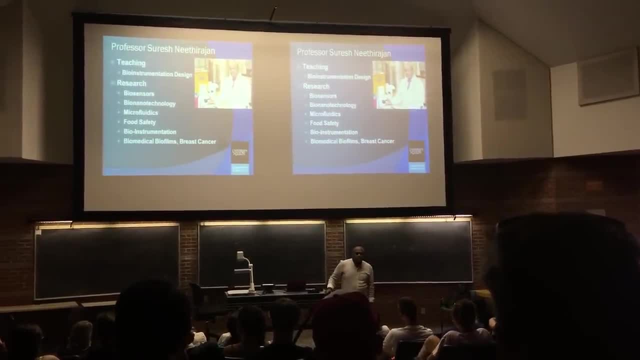 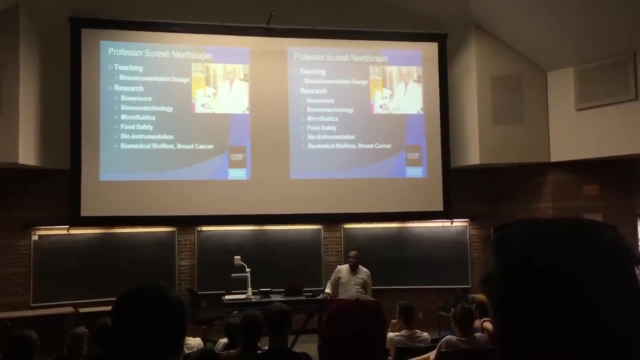 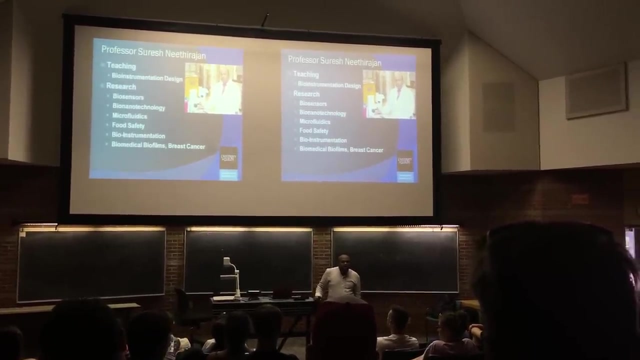 Texas instruments, Microcontroller boards. So you use sensors and transducers And other related Circuits components To build real time prototypes To solve real life solutions. As you make progress, Typically during the third Or fourth week of November. 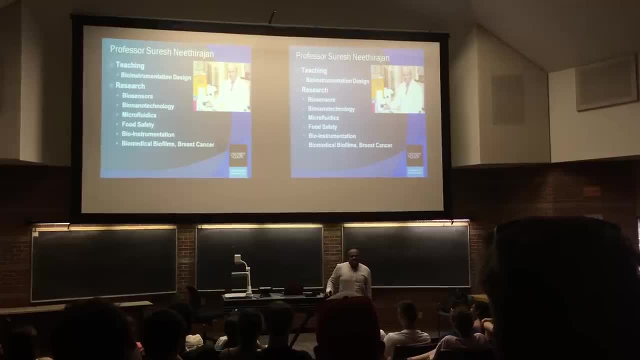 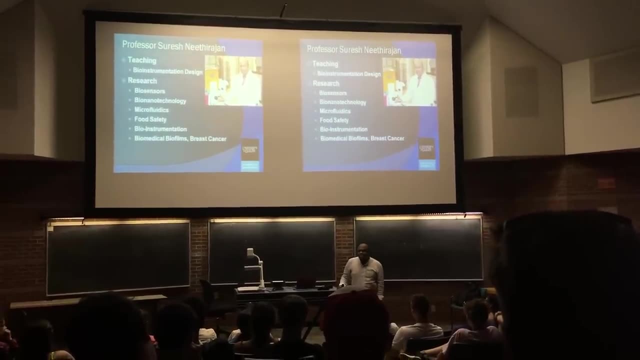 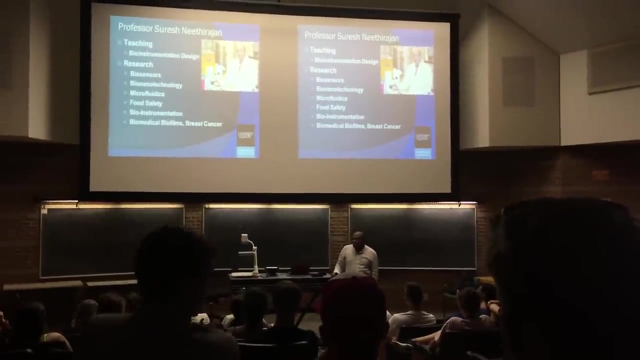 Every year there will be a big Celebration, A ceremony that will happen in the atrium. It is called bio instrumentation Trade show. Several industry personnel Will get to act as judges To judge the design project. You will be working. 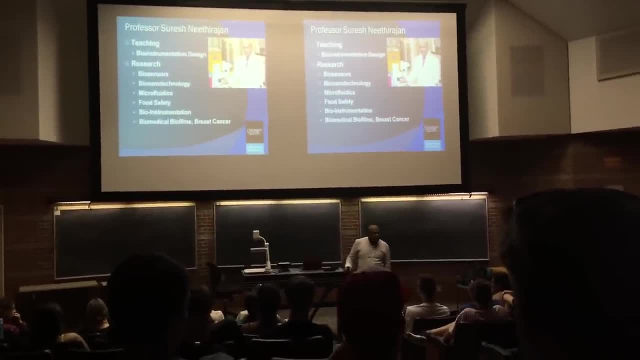 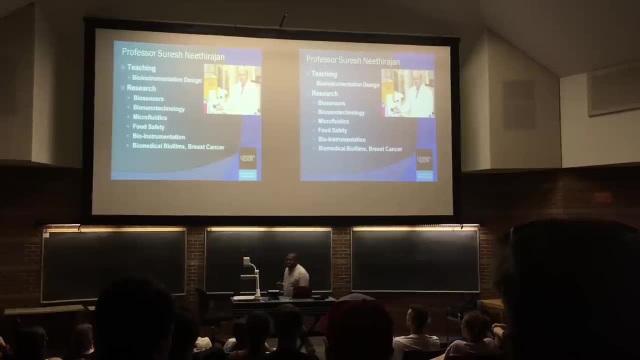 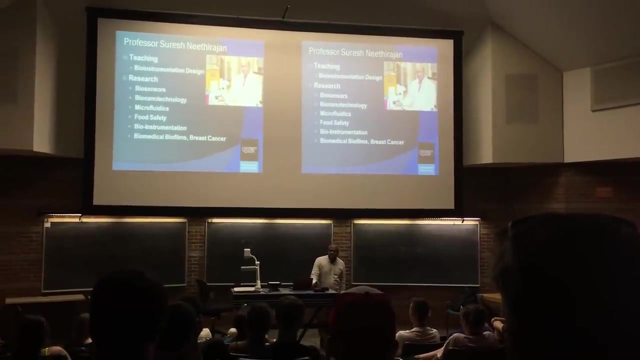 Over the period of three and a half months, And then you get judged And the grades will be provided By the industry judges themselves. In terms of research, I develop a variety of sensors: Sensors for avian influenza, Sensors for breast cancer. 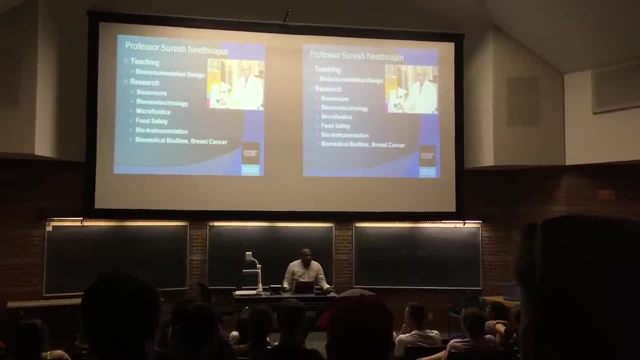 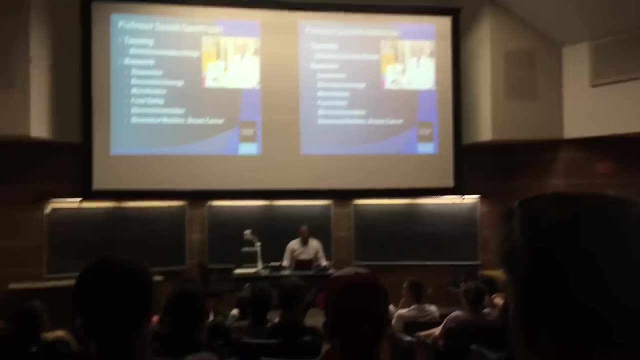 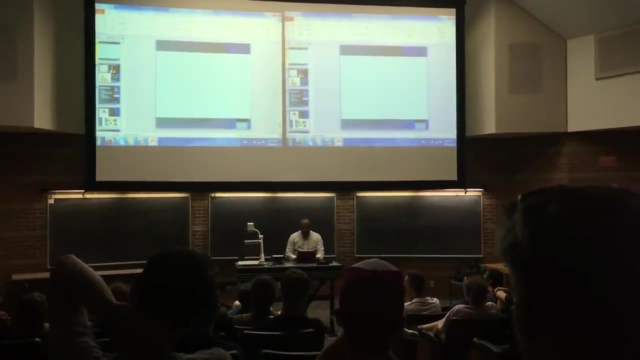 Prediction and detection, Studying bio films, As well as Developing novel tools Such as microfluidics, Mainly focusing on bringing real life solutions For food safety And biomedical applications. I'm going to show a quick video, This two minute video. 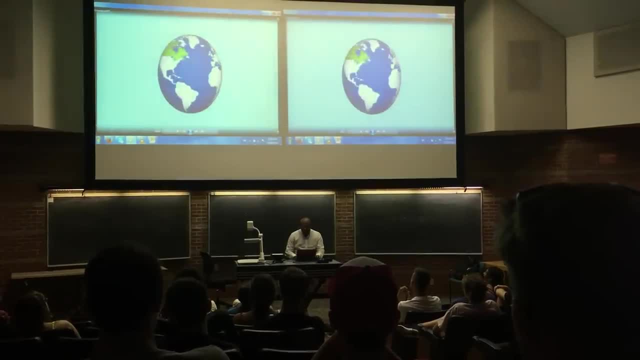 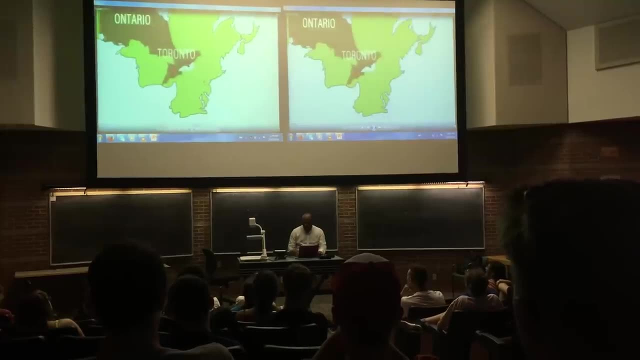 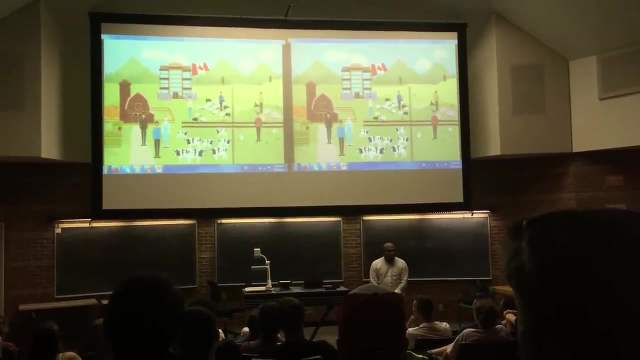 That will talk about The type of research we do. Located at the University of Guelph In the Canadian province of Ontario, About an hour from Toronto, Is the Bio Nano Lab. Researchers at the Bio Nano Lab Help create And keep our food supply safe. 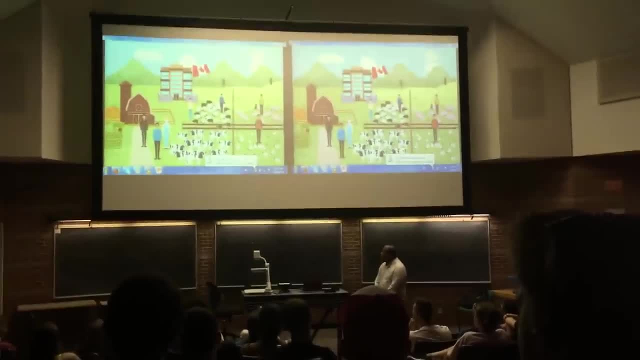 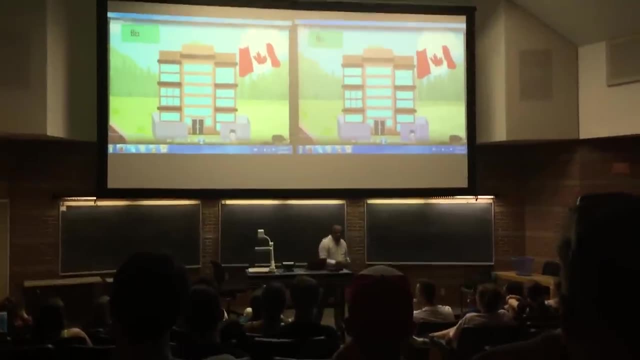 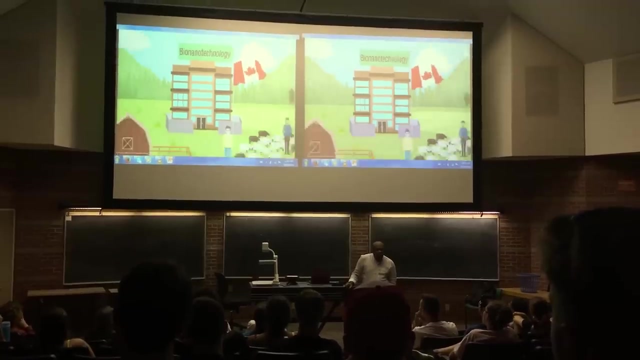 By improving the way farm animals Are diagnosed and treated For health threatening symptoms Such as ketosis and avian flu. They develop new tools By combining biology, Chemistry and physics With tiny mechanical structures Known as bio nano technology. Unhealthy farms. 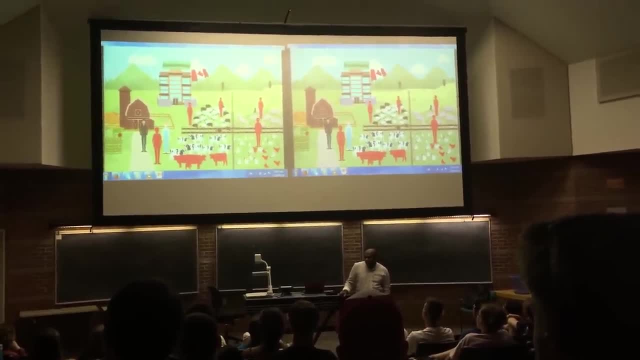 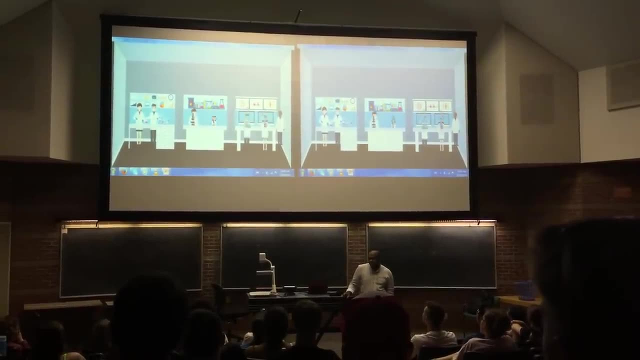 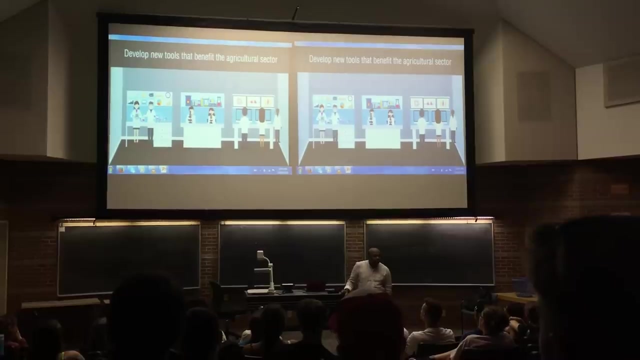 Not only threaten the lives of livestock, But also the lives of humans. So The team of researchers Study the complex behavior Of molecular cell mechanisms In order to develop new tools That benefit the agricultural sector. Their research Of nano scale biological systems. 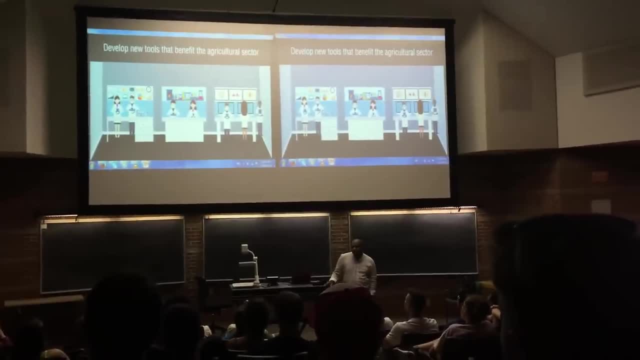 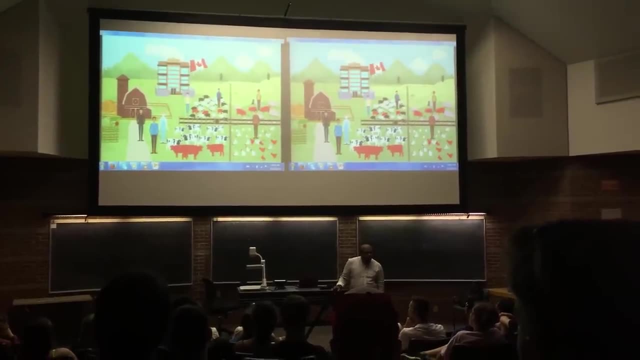 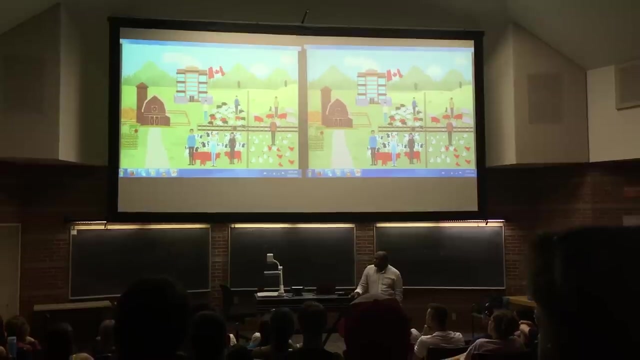 Has led to the development Of analytical and diagnostic Hand held tools That can emulate a lab in the field. This means Animals with health issues Can be diagnosed on the spot, Without waiting hours or days. The sooner a diagnosis, The quicker a remedy. 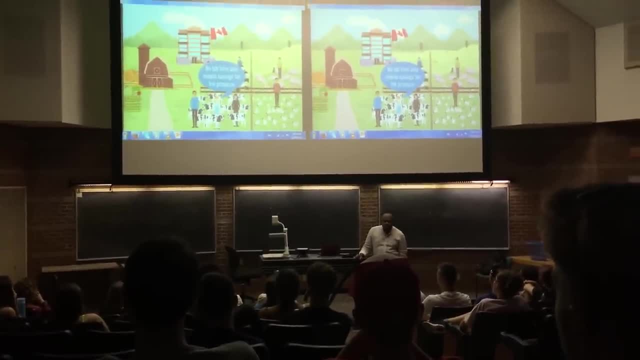 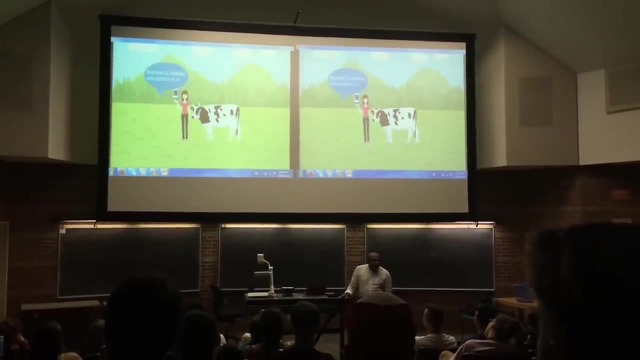 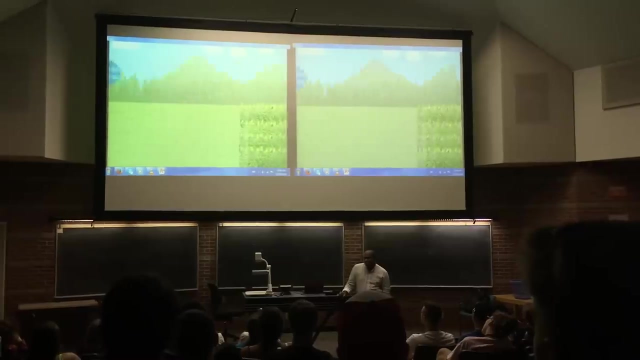 No lab time Also means savings for the producer. So far, The bio nano lab has developed A bio sensor For detecting the cause of milk production In dairy cattle. Early identification of avian influenza In poultry from cell structure behavior. 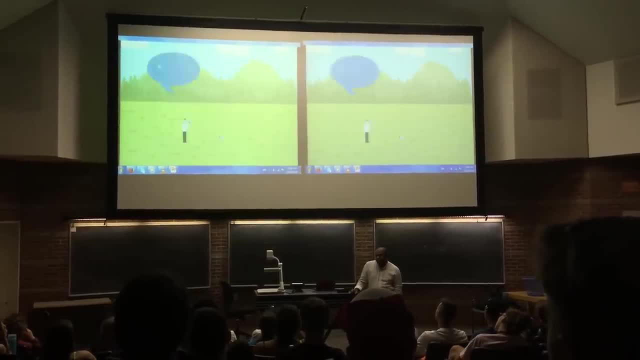 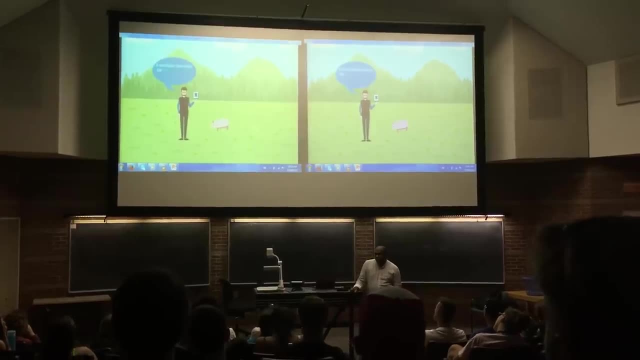 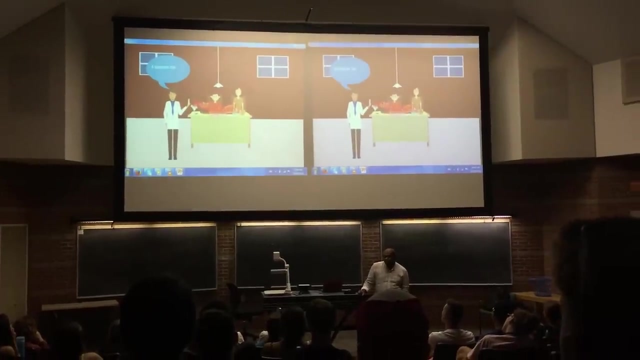 Chromosome imaging That marks genetic disorders, Methods of screening pharmaceuticals For their effects, A micro fluid and tissue model That emulates wounds And allows treatment In cases of drug resistance. And a bio sensor That quickly detects allergens. 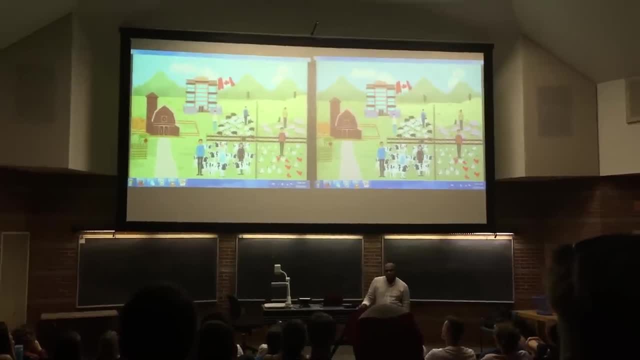 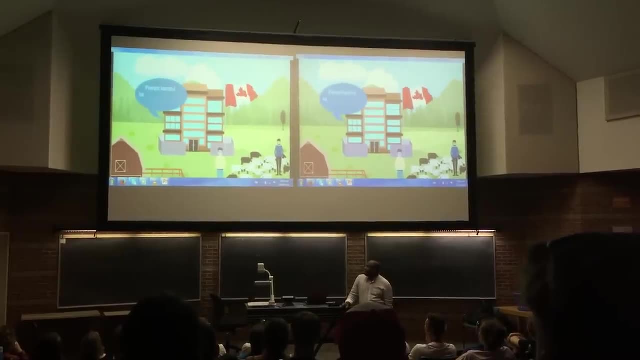 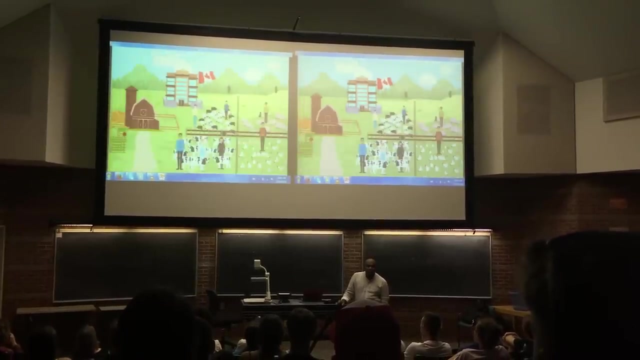 Like peanuts and gluten, And many of these developments Are currently being used in the field. today, The bio nano lab Has also been researching ways To prevent harmful bacteria From infecting wounds And prevent rejection of implants By using an electric current. 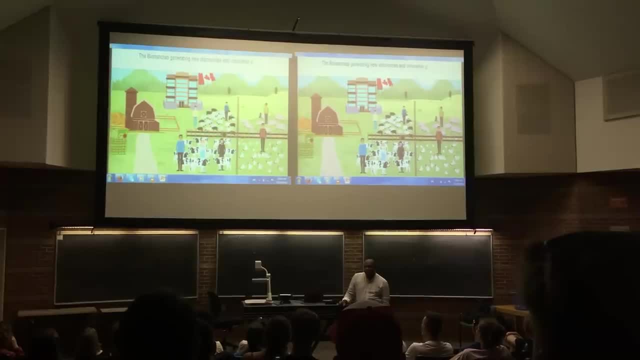 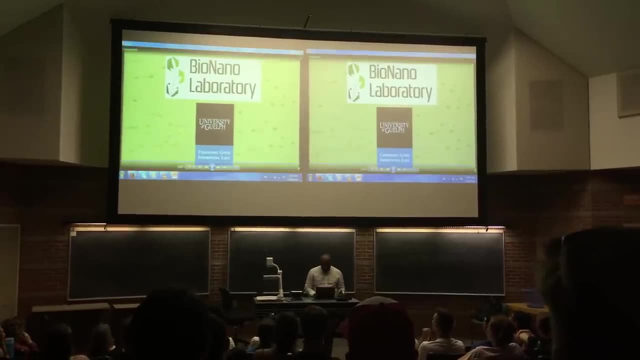 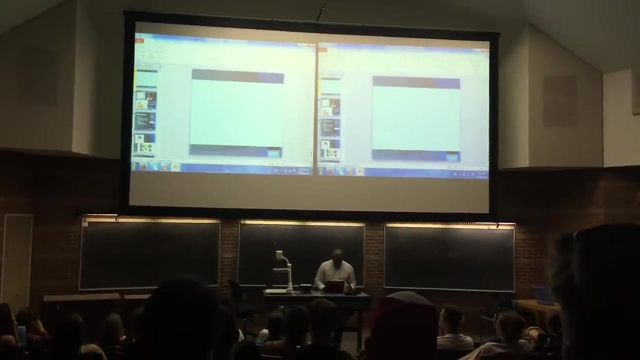 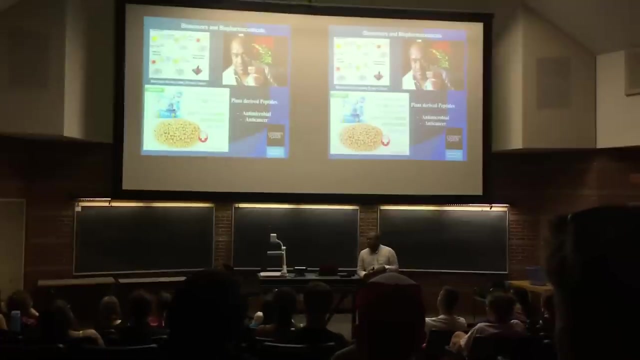 The bio nano lab, Generating new discoveries And innovative products That improve the lives Of all living things. So, in addition, We also synthesize novel chemicals, Such as protein based peptides From soybean. Some of you may be allergic to soybean. 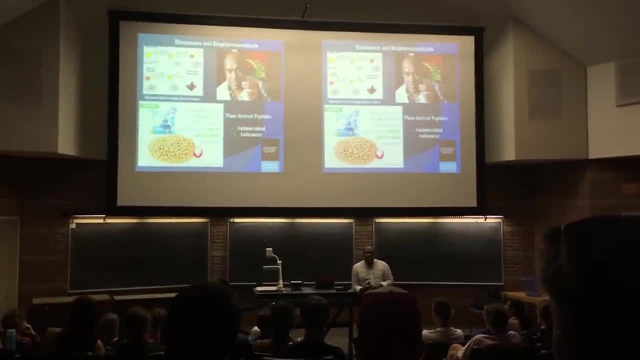 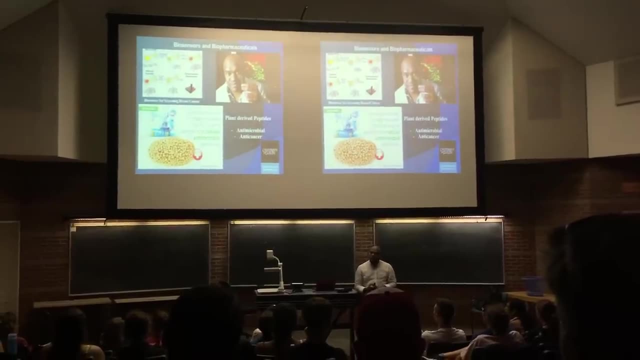 But they actually serve As a component To kill cancer And also act as an antimicrobial agent, So it's called bio pharmaceuticals. Non-petroleum based chemical Can be produced from plant based As well as the skins of microorganisms. 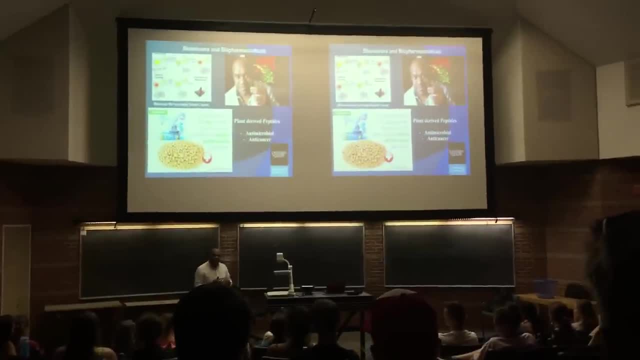 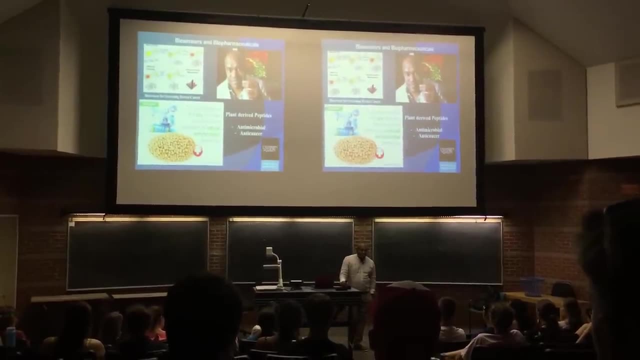 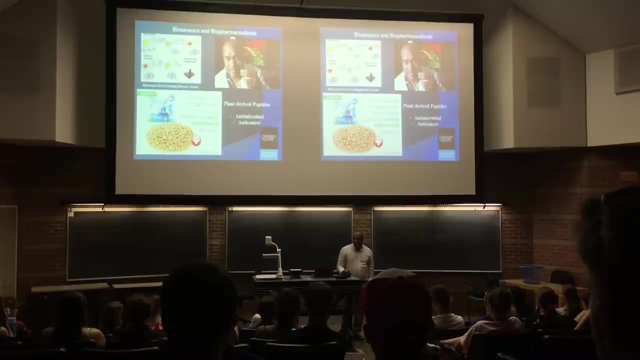 And frogs And other tiny little animals. We can synthesize specific components, Specific chemicals, Such as peptides, To act as anti tumor agents And anti microbial agents. So that's the type of research we do, In addition to the development. 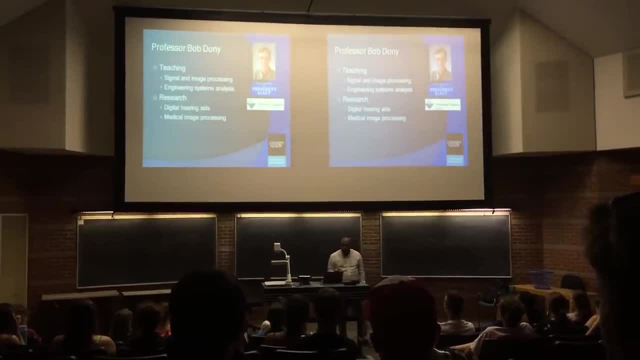 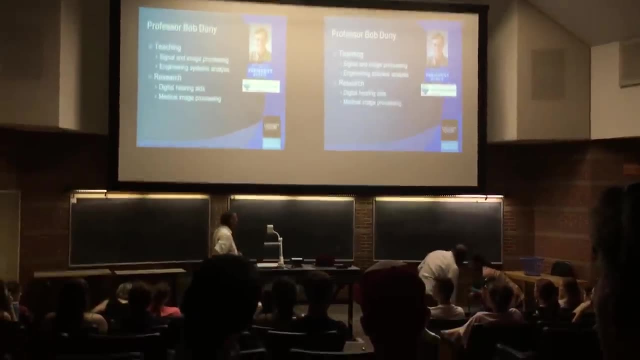 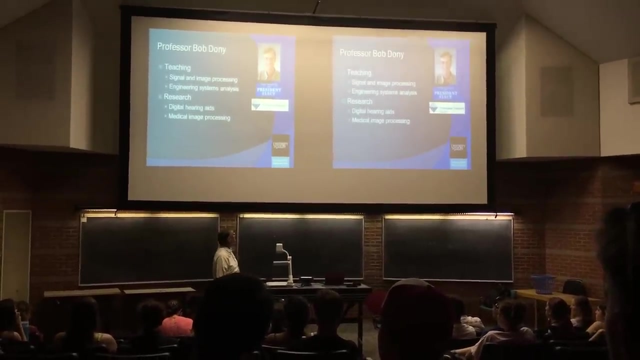 Of biosensors And bio instrumentation tools. I would invite professor Domi now. Thank you, I'll be very quick. Unfortunately You're not going to see me Next year. Normally I would be teaching An engineering systems analysis course. 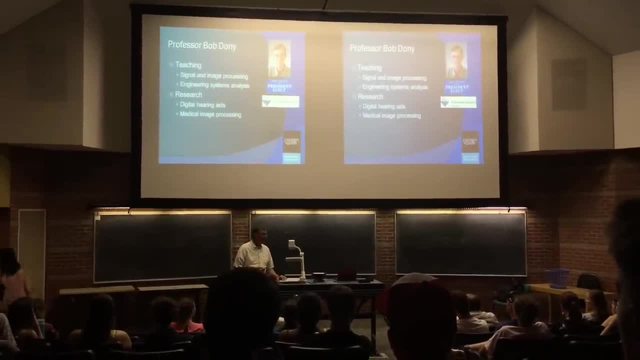 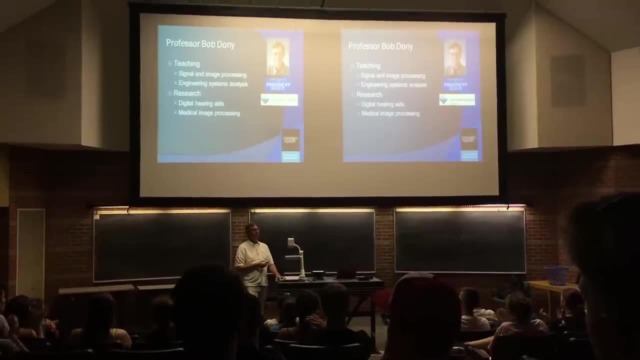 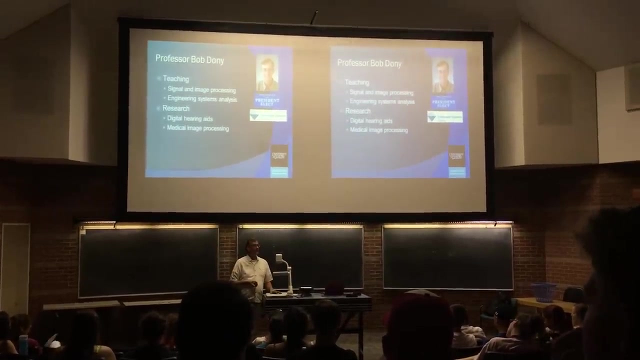 But I'm going to be a little busy. I was just elected president Of professional engineers Ontario, So In fact I have a history here Of people being elected, And I'm also glad to be Professor emeritus Four times. 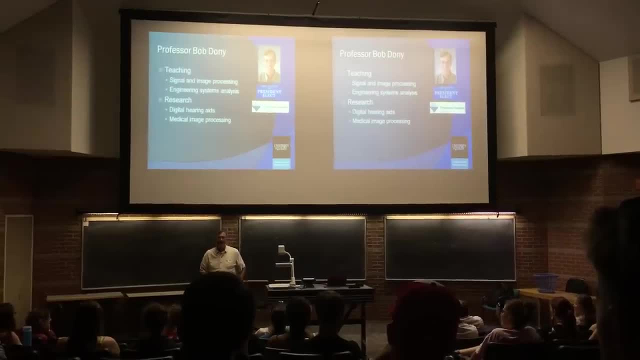 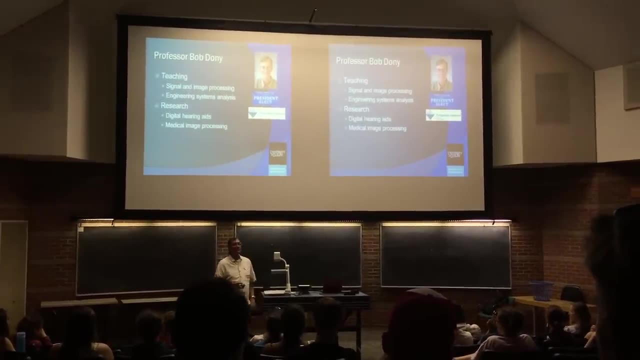 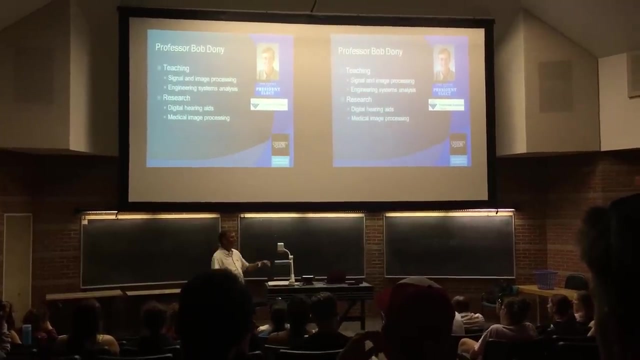 Which I'm not going to go four times. Anyway, That's what I'm going to be busy with Next year. During my sabbatical, I also teach in student processing And some medical imaging work As well. So I'm one of these strange people. 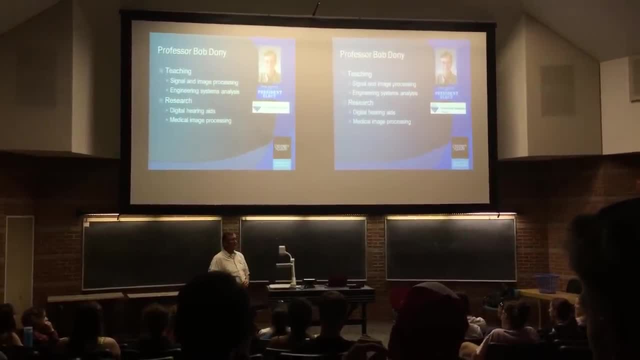 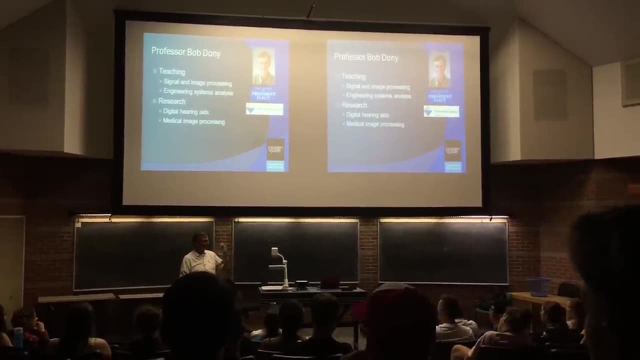 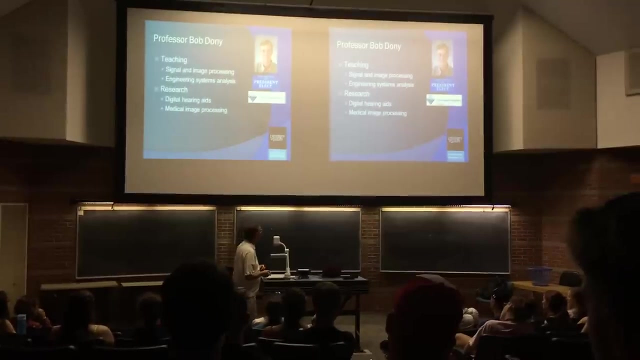 I'm often in various programs That help with the ESNC, Help with the biomedical. Again, we don't have departments So we tend to talk Again, like I was talking, about part environmental, Part biological. So that's one nice feature. 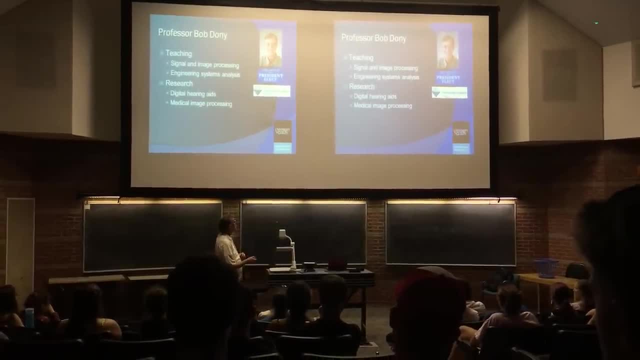 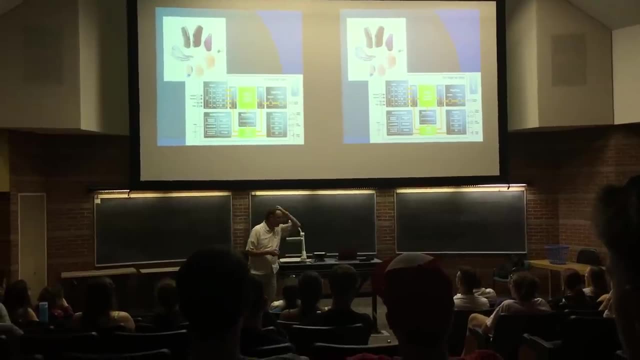 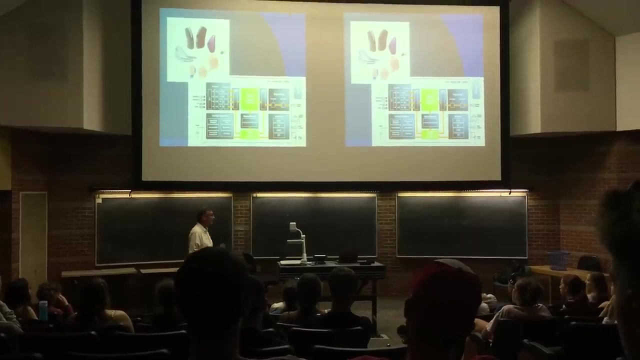 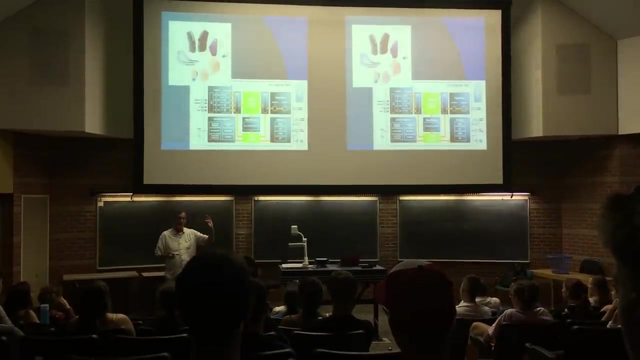 Well, Um, No, All right. So some of my research Comes out of signal processing. Hearing aids, A medical device. Hearing aids nowadays are mostly Little computer chips in your ears. They have a program. You program them. Thankfully they don't run Microsoft Windows. 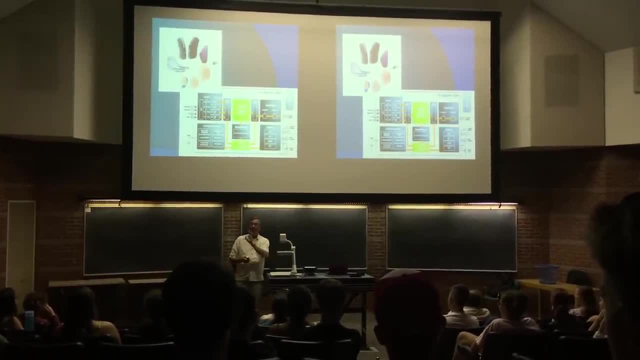 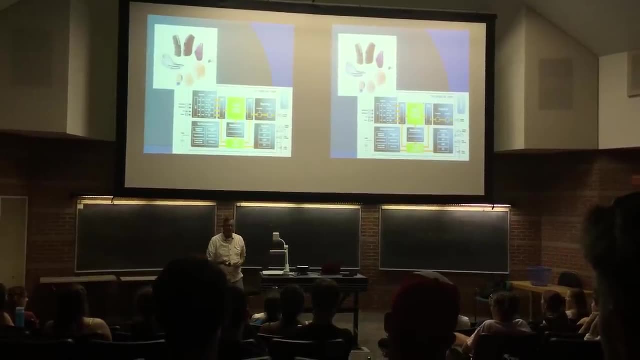 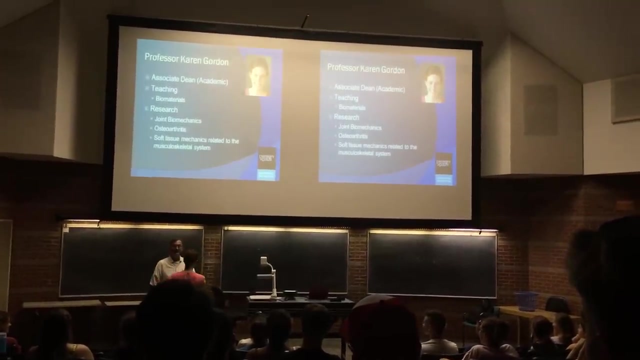 But What algorithms Can be used To make sure that the noise cancellation Here is different from the noise cancellation, Let's say, in your house And I will pass it on to the next? I said I'll be quick, Yeah. 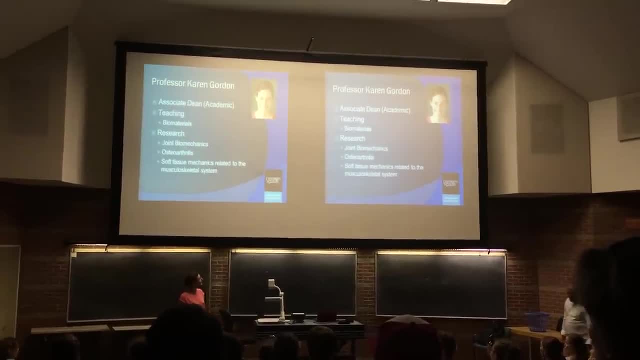 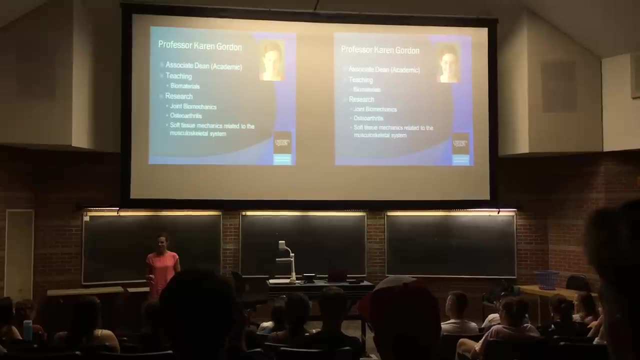 I also will be quick. Good morning. So my name is Karen Warden. I am a professor. Actually, I'm a professor here in biomedical engineering as well. I actually went through the biological engineering degree from my undergrad, So I know the ropes. 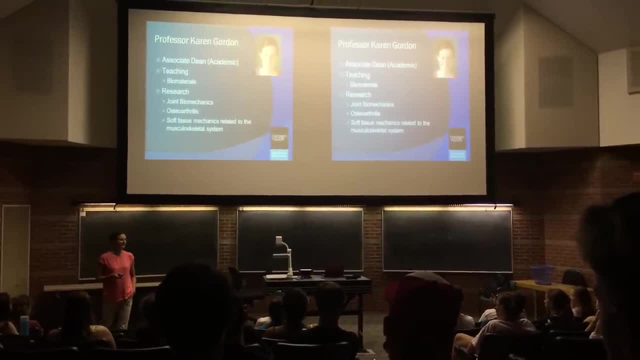 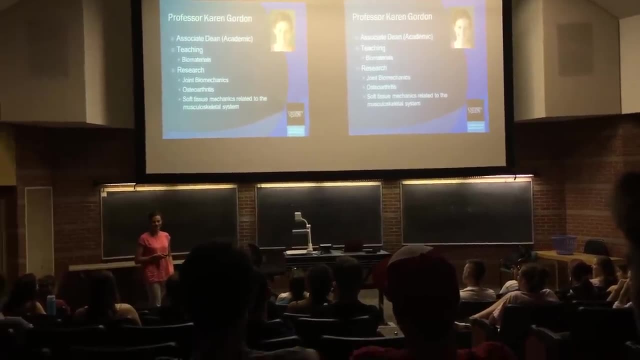 And then went on to do my PhD In orthopedics, So looking at artificial replacement joint And prosthetics. I teach biomaterials. You'll see me in three years If you're bio or BME Or if you're mechanical. 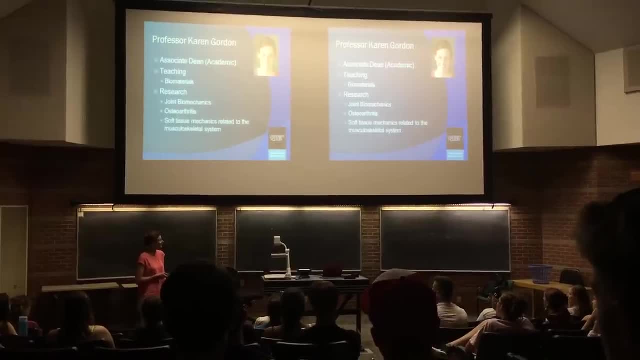 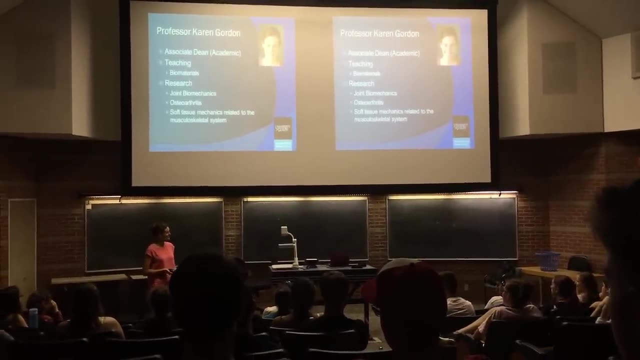 It's a good course. Starts in a couple days. Watch it tomorrow. My research now has been pretty varied Since I've come back to Guelph, So I look at joint biomechanics, Osteoarthritis, Tissue testing. 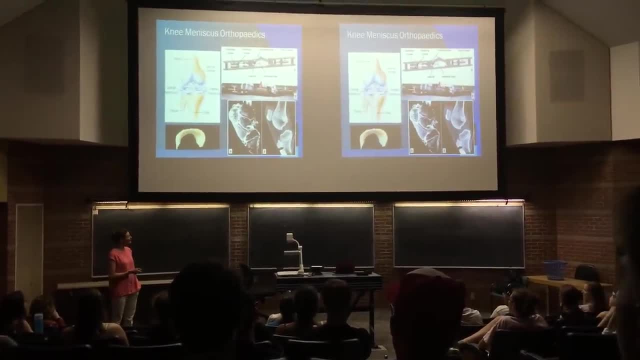 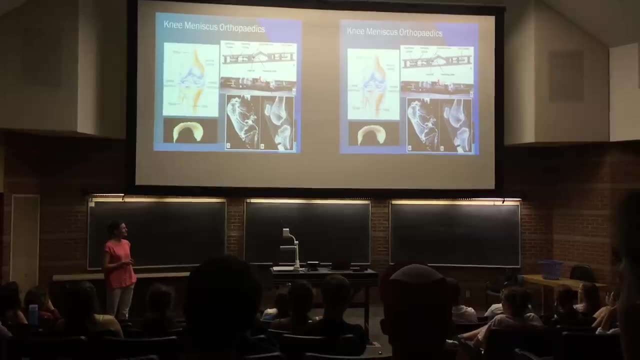 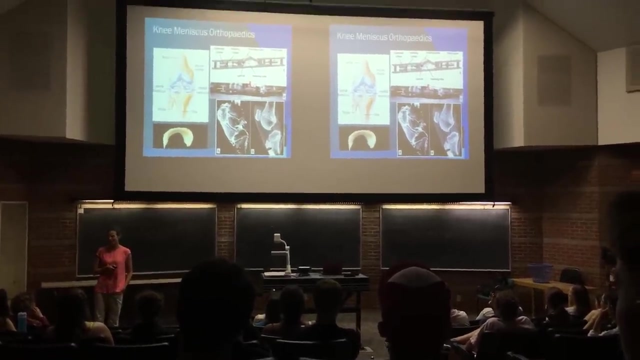 And moving now into wearable tech. This next slide A little bit, Is that the border? Yeah, So up in this corner Is sort of some of the stuff that I've done here lately, Where this is a big device Which takes the cadaveric joint. 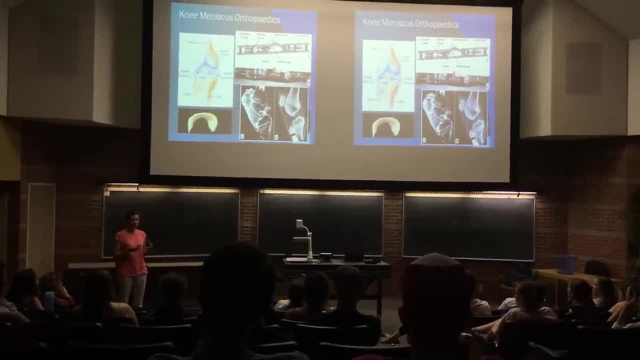 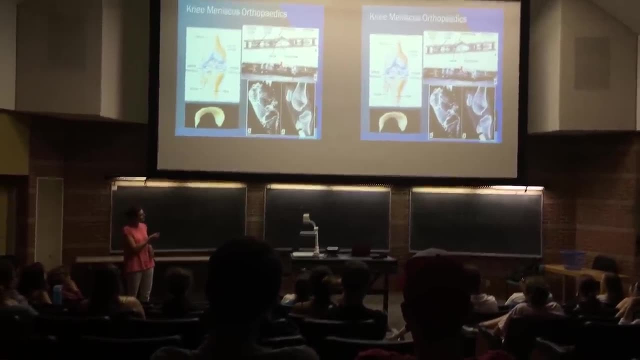 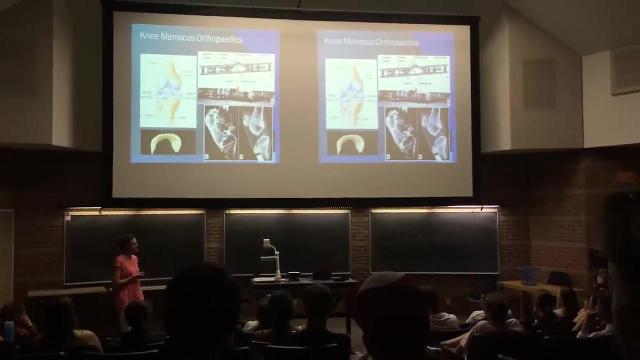 And pushes it through It's normal motion Under it's normal load. So this one way up there Is for the knee joint. Okay, This is a photograph You can see there's a cadaveric knee right in there. We've got some hydraulic actuators and cables there. 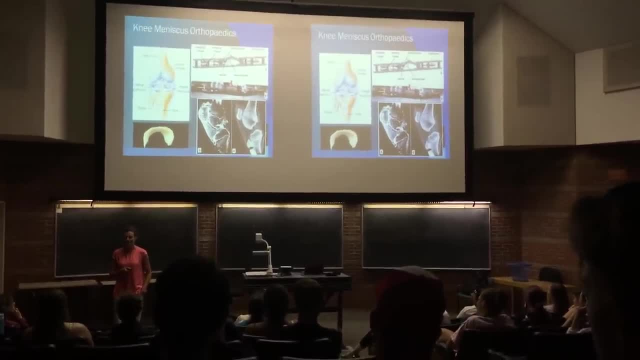 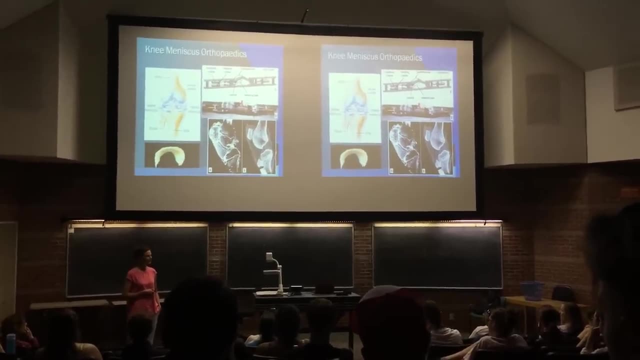 To simulate muscle action And we try to replicate gait that way And this is really useful for surgeons. So this work was done with a surgeon At UWL In London, Ontario, Who was interested in trying to optimize The surgical procedure. 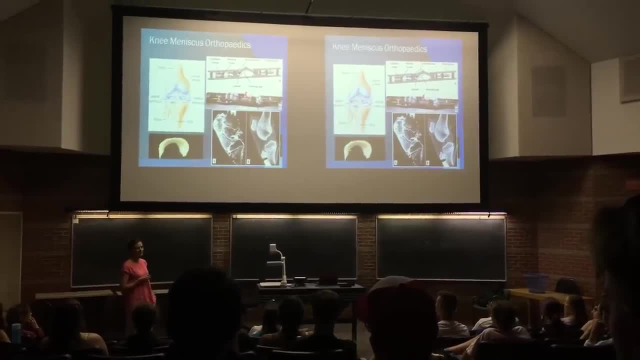 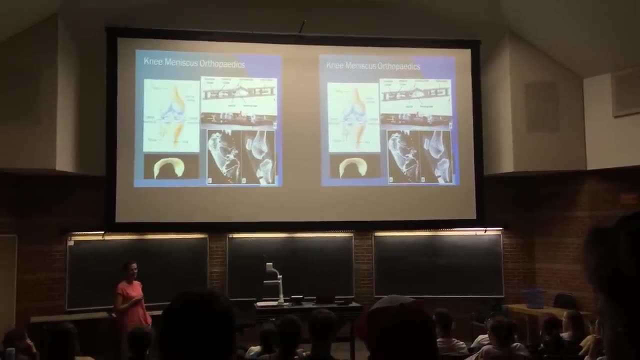 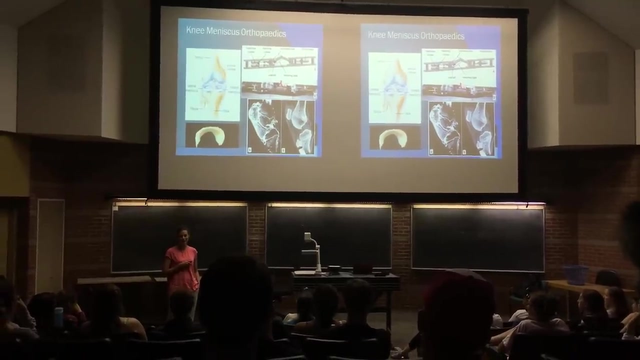 To insert these? Do we know what those are? Anyone? Meniscus, Meniscus Good. Anyone ever torn their meniscus ACL? So lots of injuries where the treatment now Is surgery And you might get a replacement meniscus. 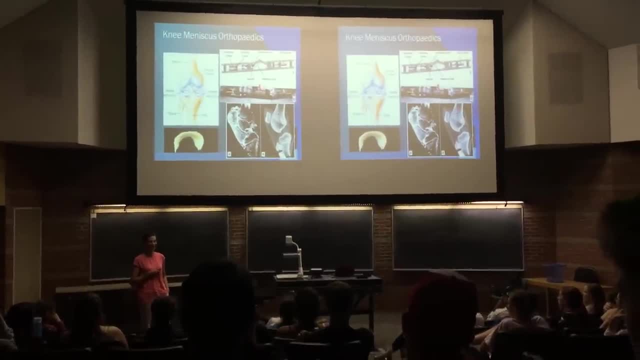 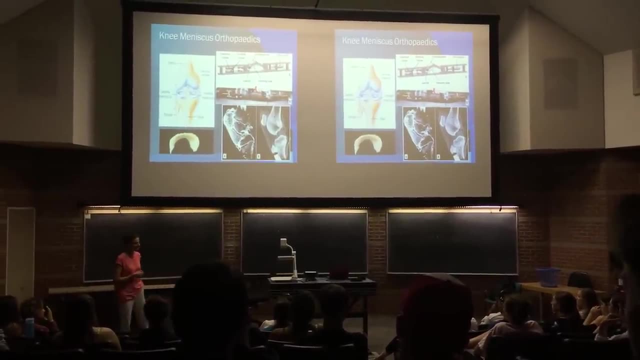 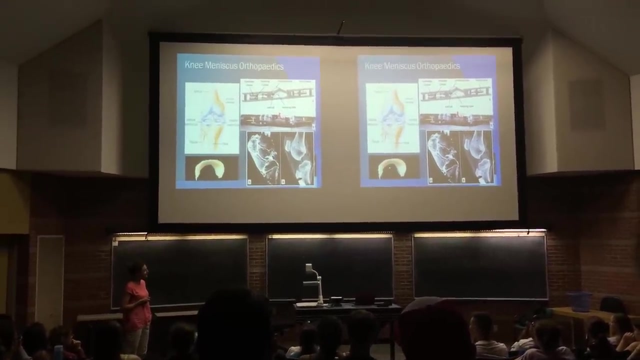 Where do we get replacement meniscus? from Anybody? Cadavers, Donor cadavers- And we're working on artificial materials, Antigen materials, To get these with. The problem with putting these in For the surgeon Is that you can stick them into the joint. And they're so down That you have a multitude of different Surgical techniques to sew them down, But the biggest issue is That they tend to bulge out In the patient afterwards. So this device, We made it compatible with MRI. 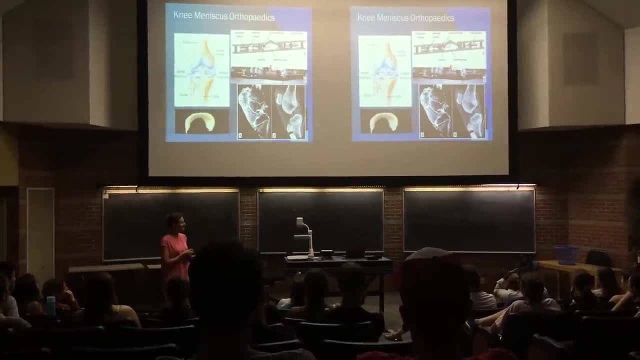 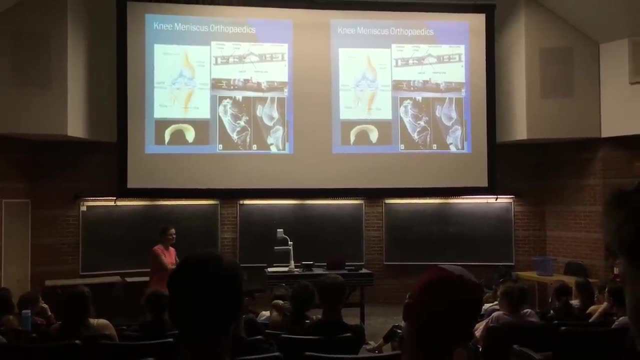 Which was difficult, But we could get both MRI images And CT images of the knee joint Under load during simulated gait So we could actually see whether or not Technique one Would result in a bulging meniscus or not. 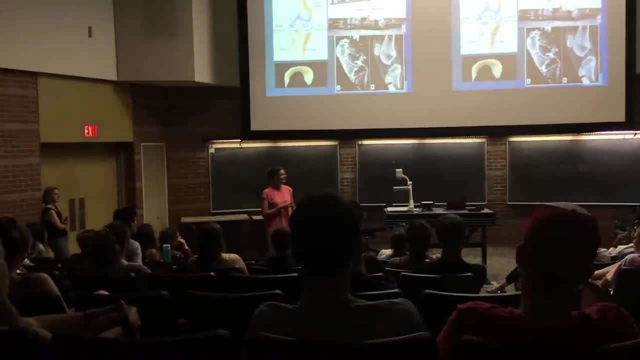 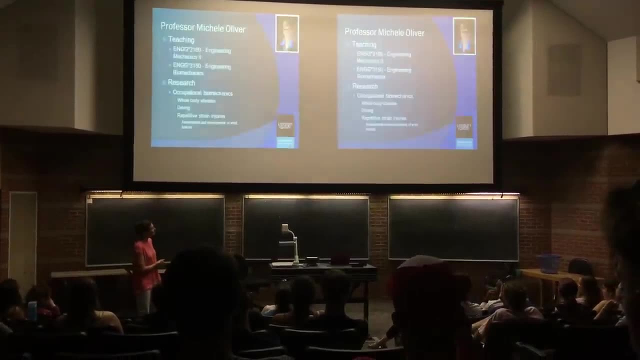 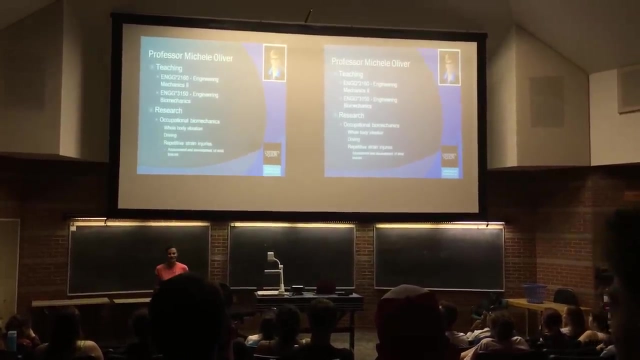 Okay, So we're working at Developing a similar, Similar simulator For the upper extremity And working with- Yeah, she's next And she's not here, So I'm going to keep going Working with Michelle Oliver On carpal tunnel syndrome. 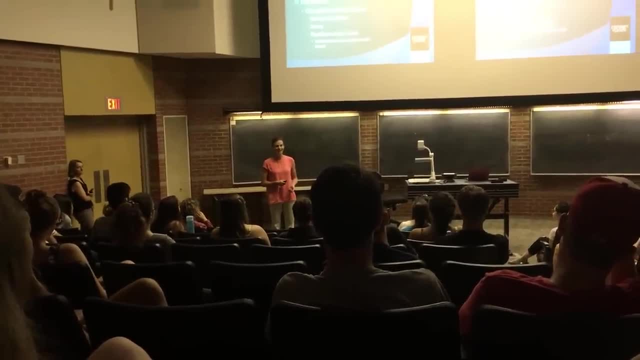 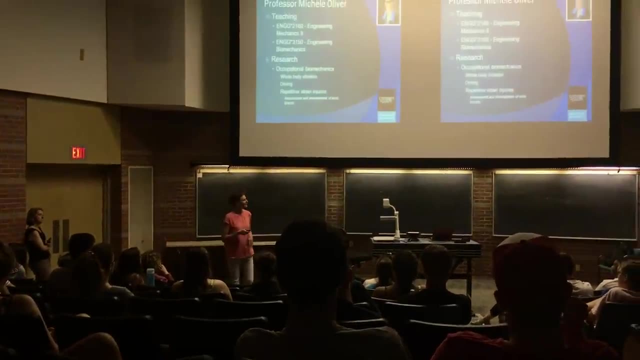 And using a simulator, Like you just saw for the wrist, That will allow us to stick a wrist In a CT or an MRI And take images At that time. So this is Michelle. She's working on that project with me. 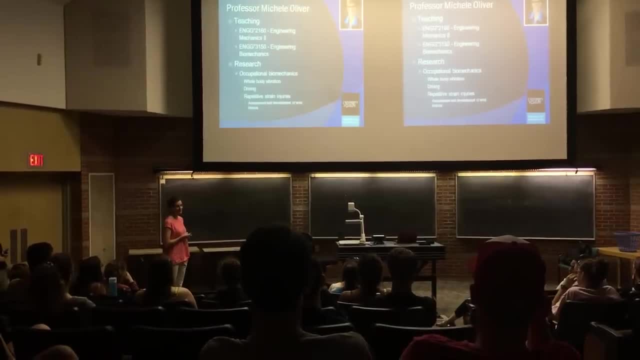 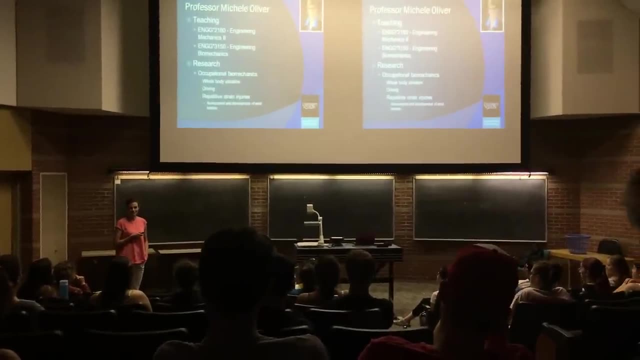 She teaches Second year mechanics- So you'll see her next year- As well as third year engineering biomechanics. So that's an elective course If you want to go sort of A more biomechanics type group In your studies. 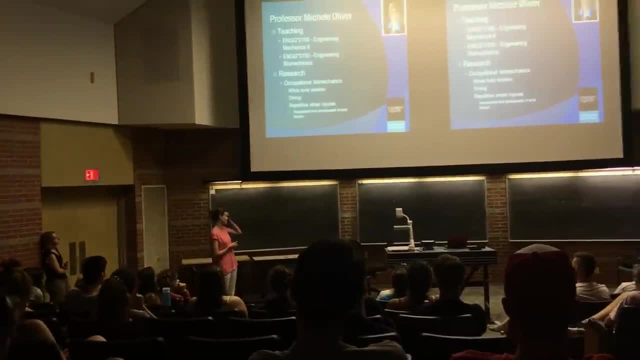 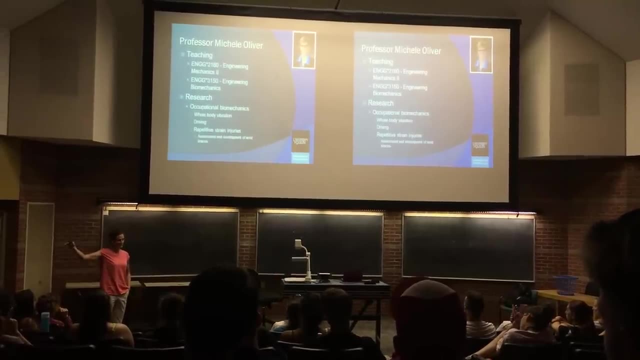 Her research is on occupational biomechanics. She studies whole body vibration And has a big driving simulator Which is pretty cool, Just on the east side of the building, Right by the parking lot there, And she does Most of her work. 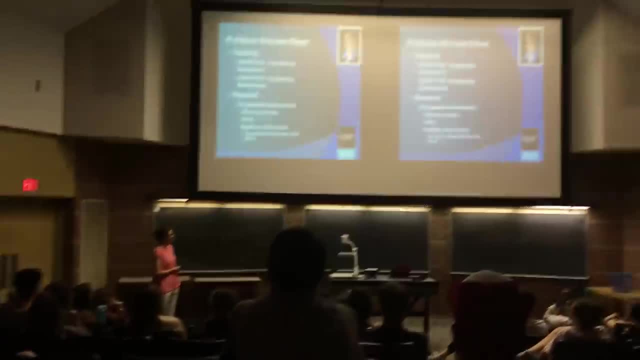 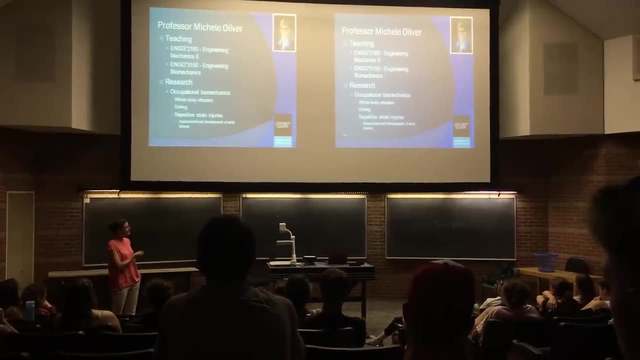 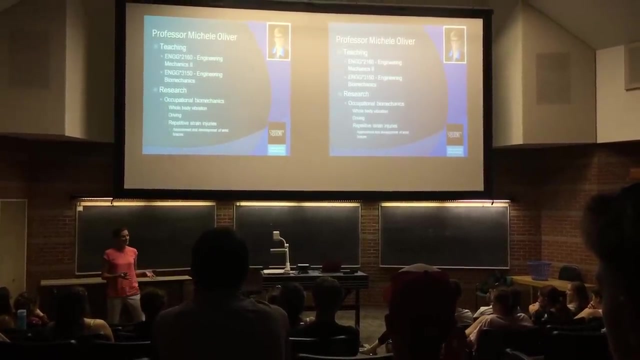 Sort of revolves around repetitive strain injuries That can be Obtained in the workplace, And so, as I mentioned, We're looking at Wrist braces together as well That could be worn in the workplace, That are Have wearable technology instrumented. 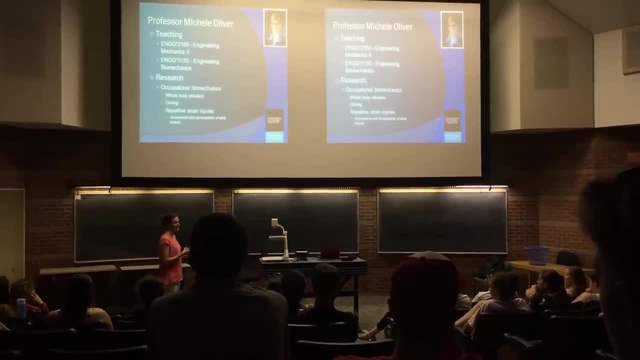 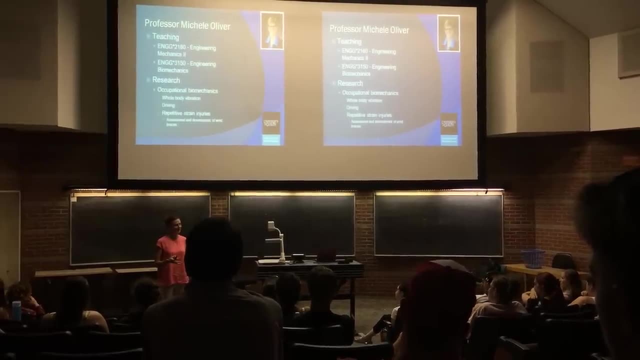 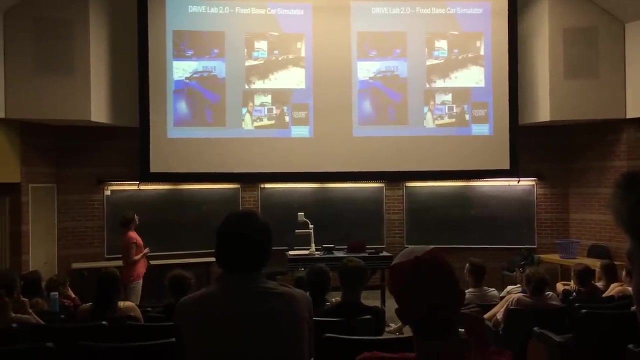 Inside them So that we can tell When you're on a shift You're hitting a point Where you really need to stop And take a break And sort of assess How much load And how many cycles You have exerted on your wrist. 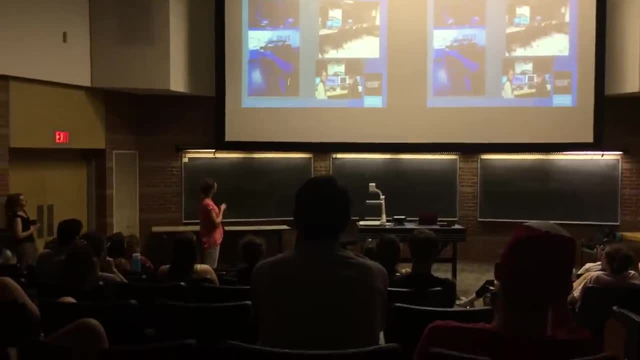 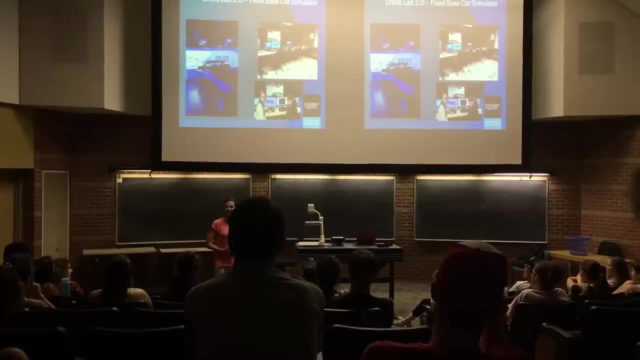 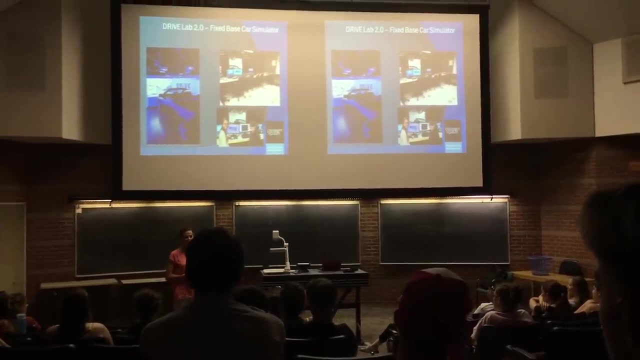 Okay, So this is her driving lab. This is her driving simulator. She's got a car in there. You go in, You put on the virtual reality goggles And you feel like you're driving. So it makes you feel sick. She has a whole fridge full of ginger ale in there as well. 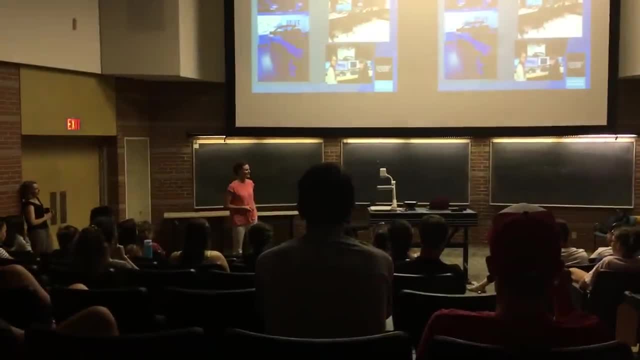 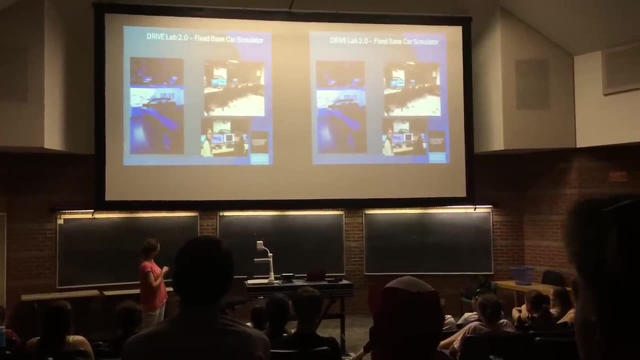 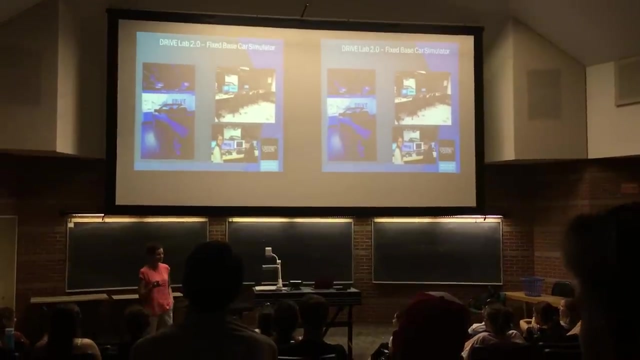 I go in there from time to time And don't tell her When I'm thirsty. And Yeah, This is one of her graduate students Who just got hired by. This is actually Dr Joni's daughter, Who just is about to finish her masters. 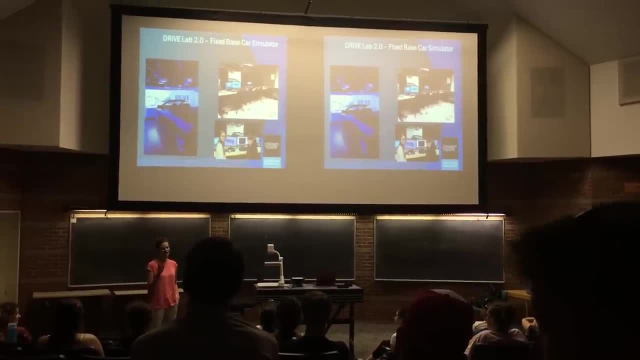 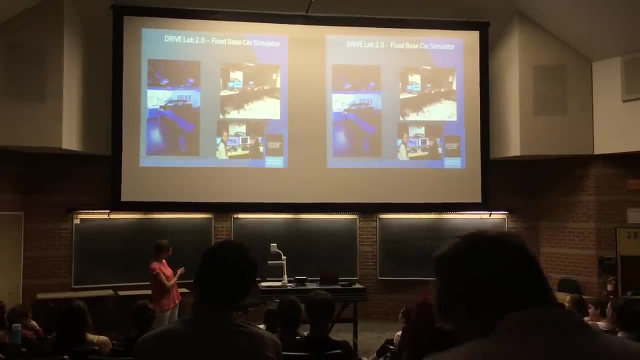 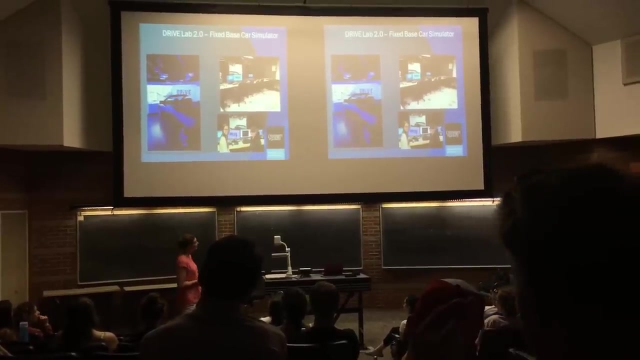 And was hired by General Motors For their self driving research division. That's right, She's driving cars. She is one of two engineers Who was just hired to work on that research, Which is a pretty wicked job, If you ask me. 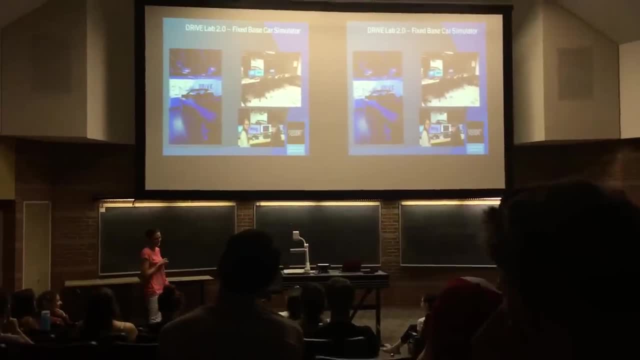 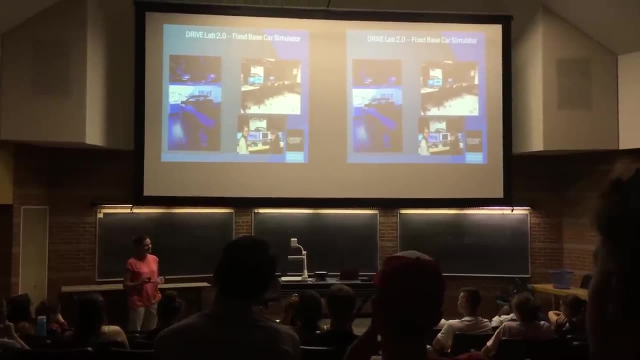 I'll take her job. Yeah, No kidding. And then Just to point out one other thing About some of the benefits here at Guelph, Or some of the things that I really enjoy about Guelph. This is I believe she says it's a psychology student. 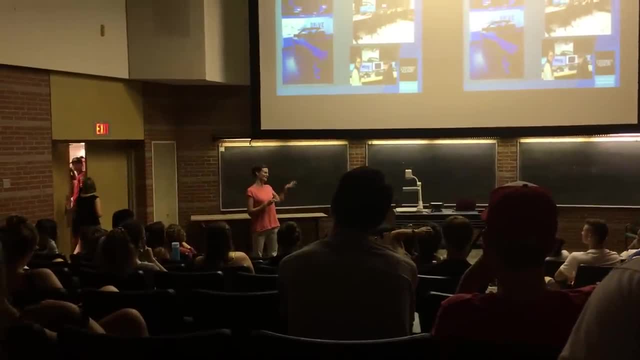 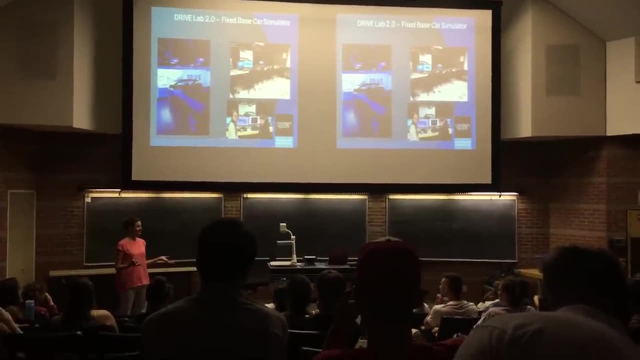 I don't know her personally, But this research is interdisciplinary And one of the big buzz words for Guelph Is that we're We're not departmentalized. in the engineering department, We like to talk to each other, We like to do research together. 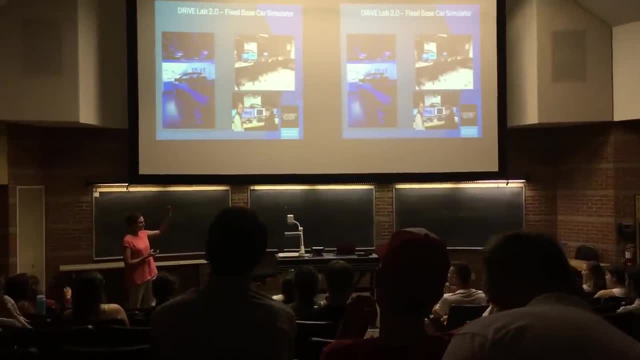 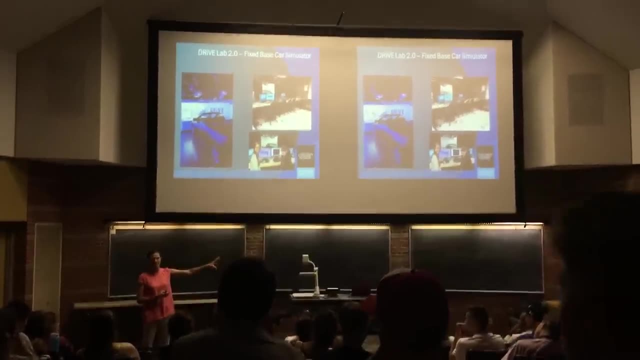 And, as well, we really try to do that interdisciplinary work Where basically the PI's are the principal investigators On all of this drive research That Michelle is doing, She's the engineer, She's working with someone in psychology And I think there's someone else in another department. 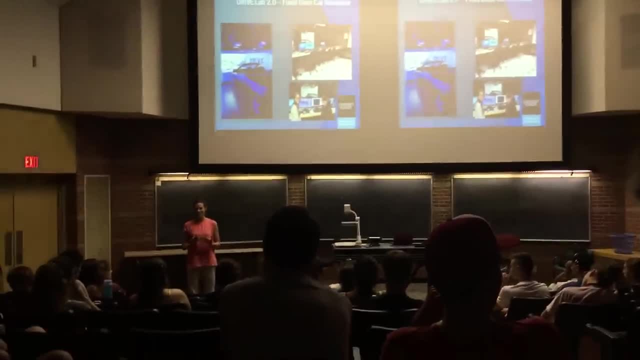 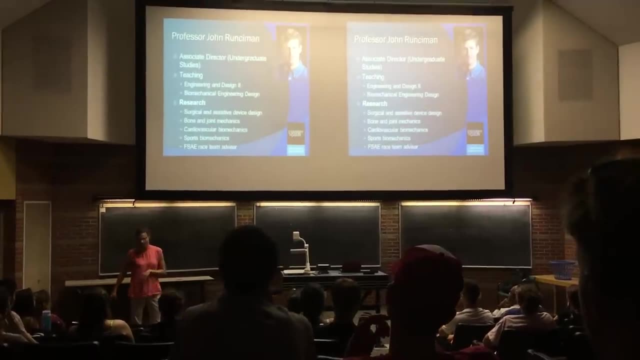 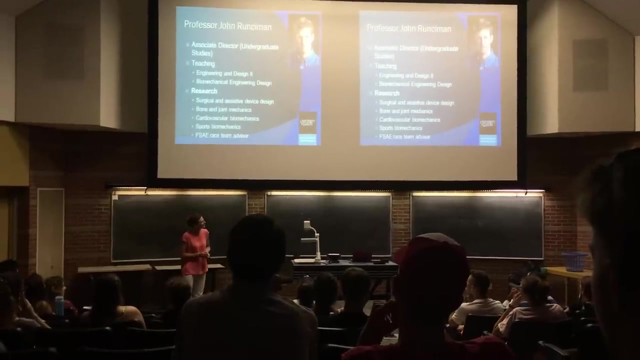 And so these students Even get to work together. So you have an engineer working with a psychology major, And so on and so on, And that's another big feature. Alright, Is John here? Oh, I thought I saw him. Okay, so I'll keep going. 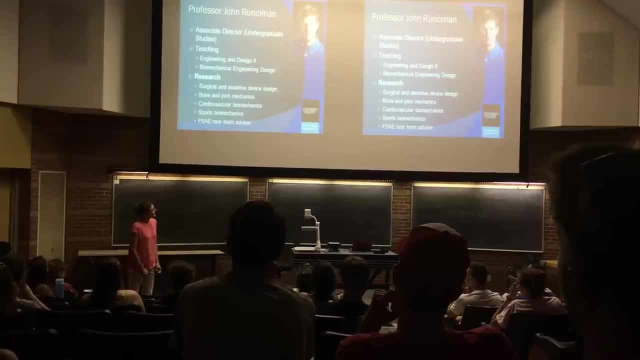 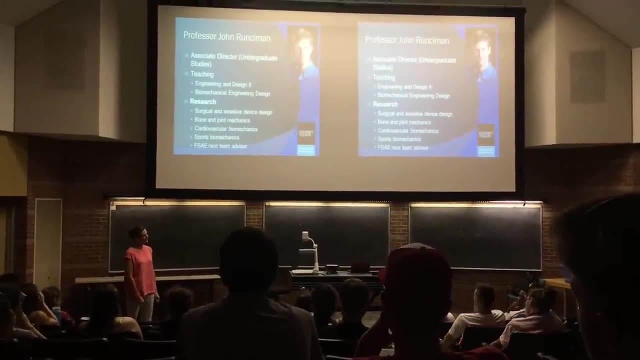 Okay. so, John, This is John Westman. He is your associate director for undergrad studies In the school, So he is overseeing the whole undergraduate program. I did that for a couple years. It's a big job. He's also teaching second year design. 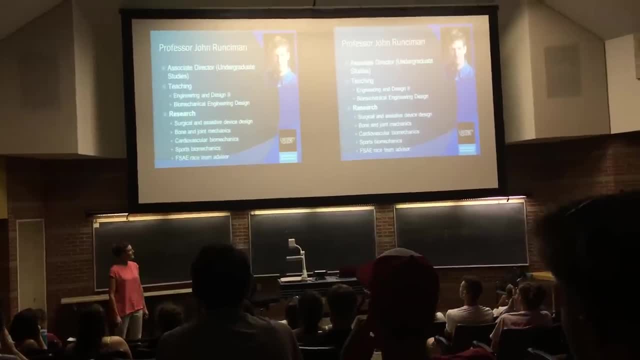 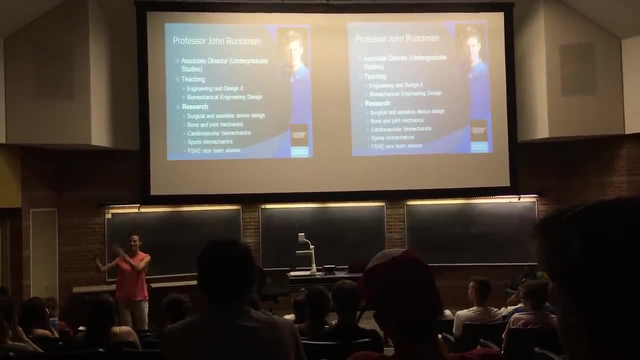 So you'll see him next year. He's in design core And he teaches a fourth year course In biomechanical engineering design. So this is an elective course In that biomechanics stream, If that's your interest in BME. 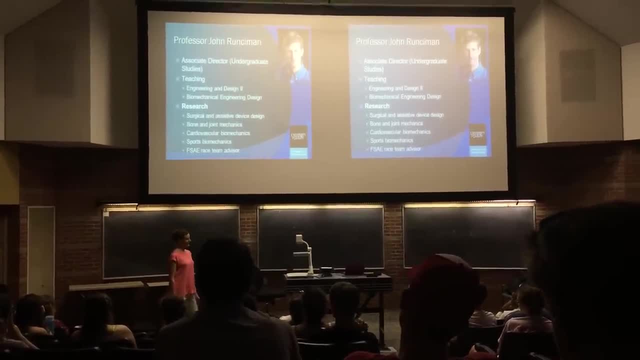 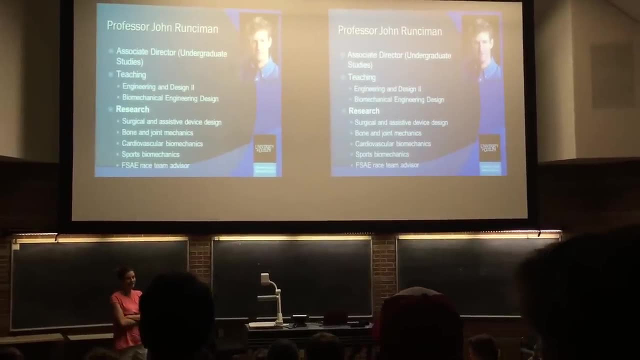 His research Is also biomechanics focused And he's done a lot of work With the vet college And he also is interested in bone and joint mechanics. Like me, We have a lot of similar interests- And looking at surgical and assistive device design. 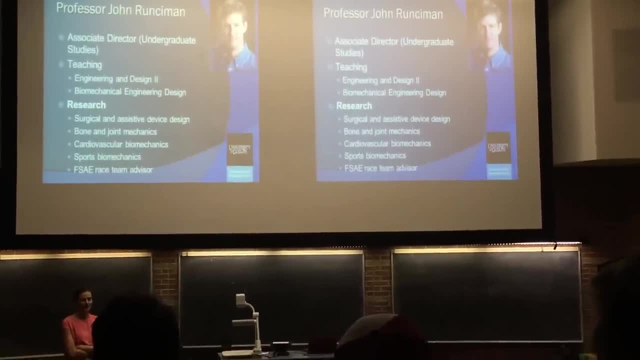 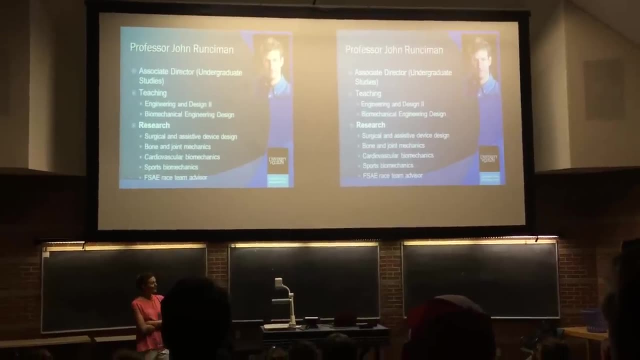 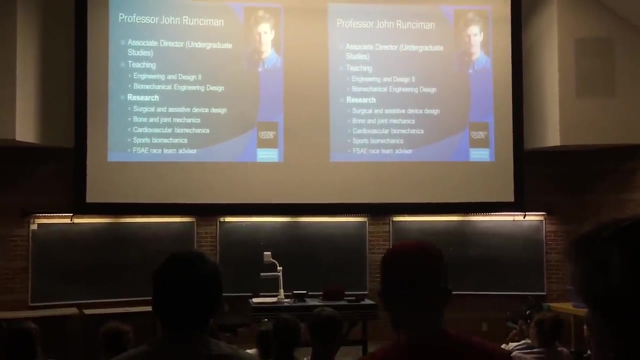 Again, He's worked with a lot of vets On helping them optimize surgical procedures As well. Lately he's deviated a little bit more Into sports biomechanics. Is that the next slide? Nope, He's done some work looking at different paddle designs. 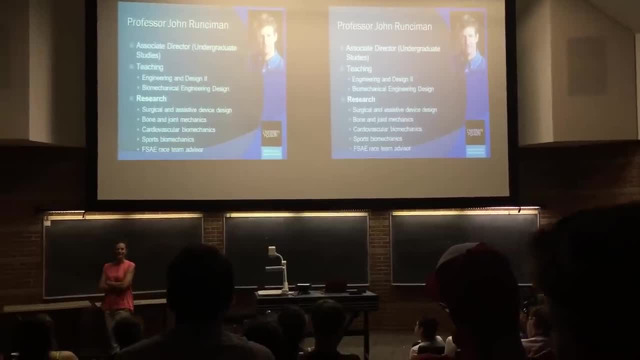 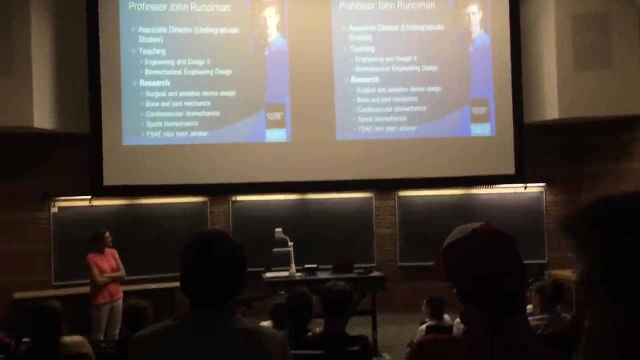 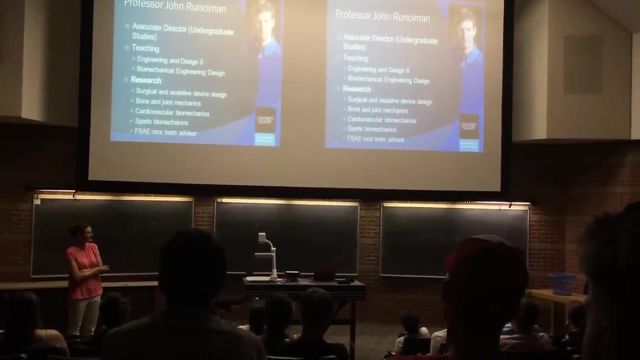 To minimize drag For kayaking And commuting, And also at water skiing And the design of your water skis, So stuff like that. And he's also Working right now On cardiovascular biomechanics, Specifically with horses And, given that we don't have a medical school here, 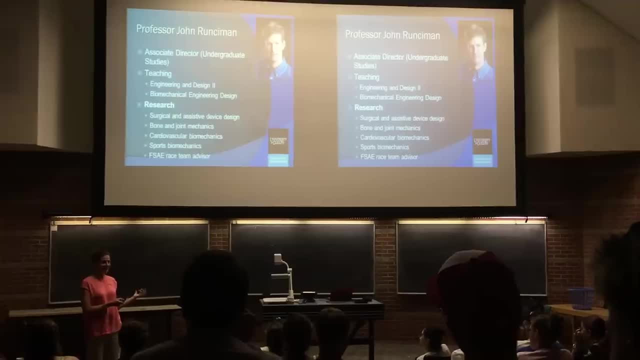 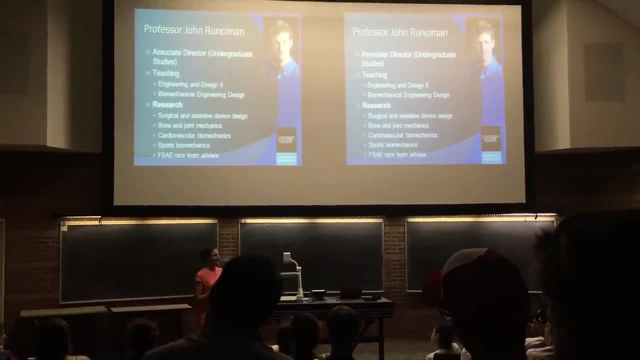 We do have the vet college And he has developed contacts there, As have I, And that's one of the key things that might be good, If you're BME, To know that this does exist Where they give us a medical problem. 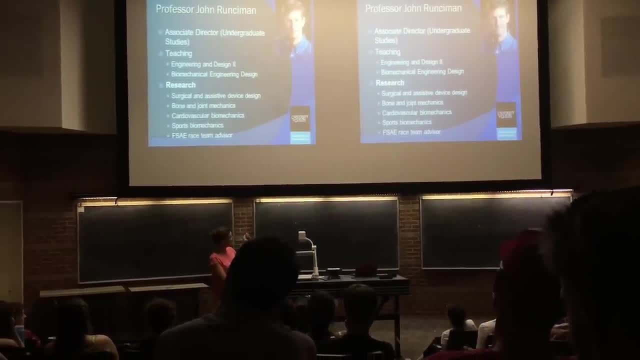 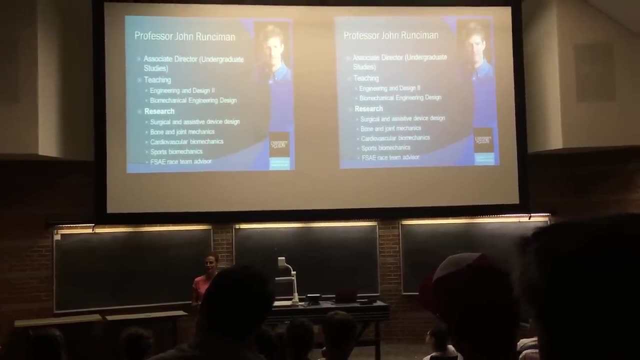 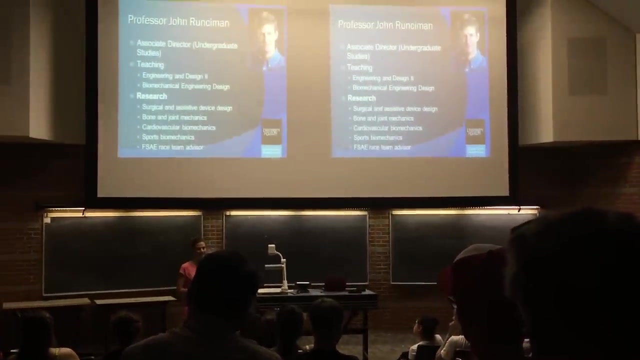 And then we work on it And for this particular project, Race horses Develop a problem And then they're trained, Overworked And their arteries actually calcify And can burst open And they can die And have to be put down.